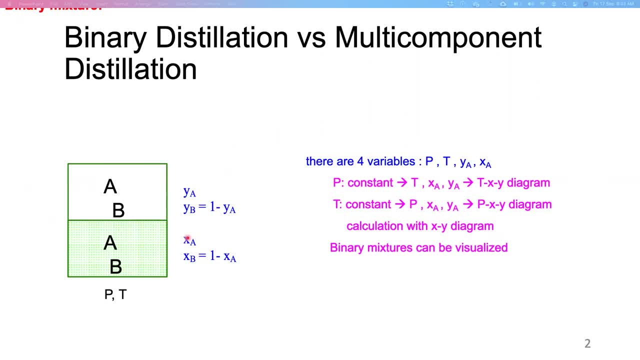 and mass fraction is called- sorry. the mole fraction of the liquid is called XA and XB is the fraction of the B, which is equal to 1 minus X a. right in the vapor phase. we have more reaction of a in the vapor, which is y a, and we have also y B, which 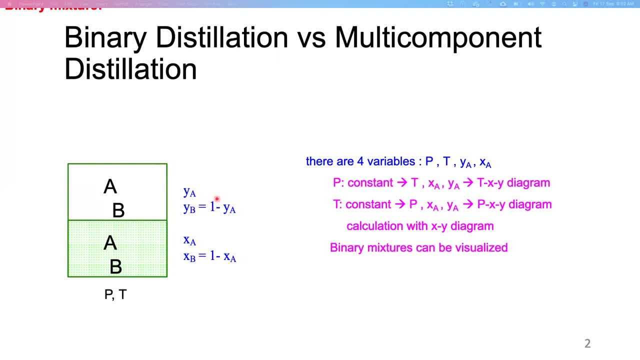 is 1 minus y a. okay, and at this condition it is also the equilibrium, or the condition is actually correlated, and then dependent on the pressure and also the temperature. yeah, so with that we have four variables. there are pressure, a temperature, mole fraction of a in the vapor, mole fraction of B in the 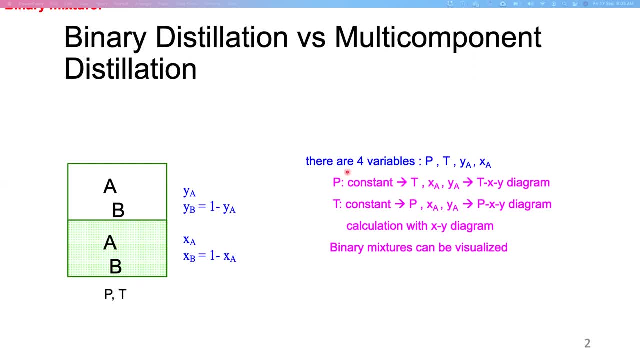 liquid. so there are four variables. okay, okay, so we have four variables. okay, so we have four variables. okay, so we have. and so we also understand that. so if the P, if we keep constant, if we kept constant, then we have the variable at the temperature, X, and also Y, yeah, and 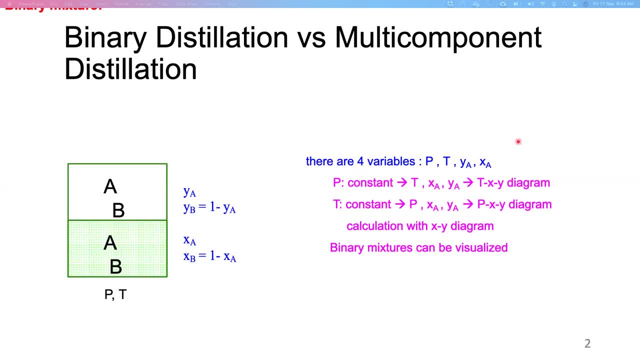 then this can be, we can. we can visualize that in TXY diagram. okay, if it is a T constant, which is, but well, it's not common. yeah, we use always P constant, but anyway. but if we have a constant temperature and then the system is defined by to be changing with temperature, then we can. 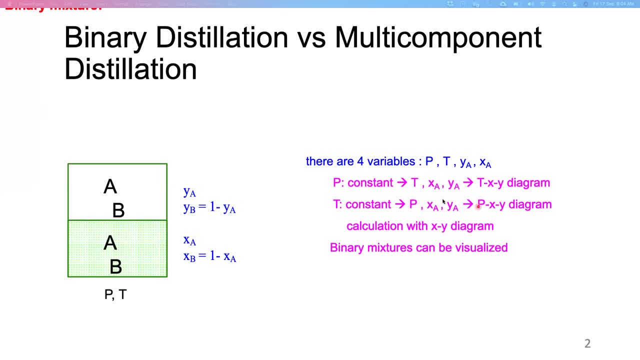 have a pressure as a variable, X, a as a variable and also Y a as a variable. then we have P, X, Y diagram. okay, so those three, those diagrams. it's actually a three-dimensional, so we can, we can visualize it in in the three dimensions, okay, P or T, X and Y, like in the remember with the tongue diagram, yeah, diagram. 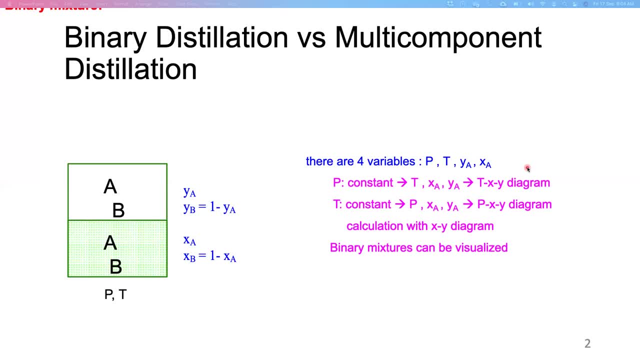 lidah as a few few weeks ago. okay, so with that we also can understand the correlation between X- Y diagram as well. yeah, so we can visualize it in the three dimensions. okay, P correlation: the trend, right. so the true difference between the two is between 2 times path and 5 times length. 110. price name end per. 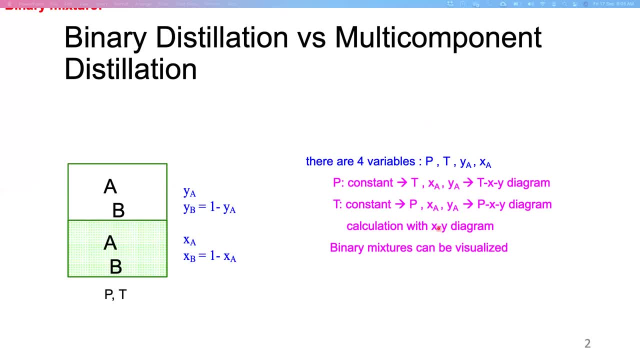 the term pulse, right, so the far what is? somebody see the different terms and do we understand the terms red and white over here? right, so that will be B. mark the time always by using the, for example, to see the composition of the equilibrium between YA and XA. so then we can, we also can have XY diagram. so so that's why thing what you've done so far, actually for the preparation for the next week time. the binary makers also can be: visualize, right, find three different combinationism, and then the energy, make sure to necessarily made. 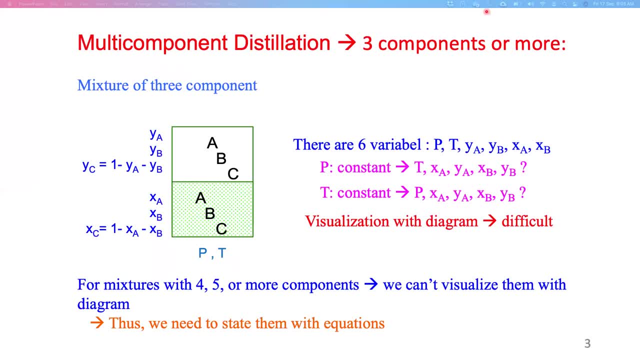 Okay, next, So what happened with the multi-component distillation? Three components, four components, five components. What do you think? Do you think you can sketch it on a diagram? Anyone? Let's have a look, Yeah, In, let's say, three diagrams. In three diagrams we have the in the three components. here we have a condition of pressure, Yeah, And also temperature, Right, And also we have a composition of X A, a composition of B in the liquid, XB, and also composition of C, where then it is dependent on the XA and XB, which is 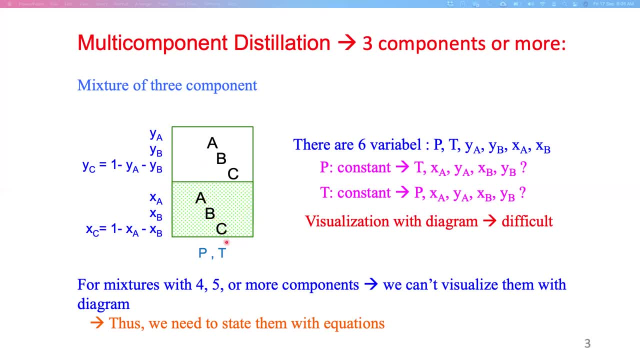 one minus XA and XB. Okay, Right. And also look at the vapor phase. Yeah, there is a YA, YB and also YC, which is dependent on YA and YB. So if we have, if we combine them together, then we're going to have six variables. This is only for three components. If we deal with 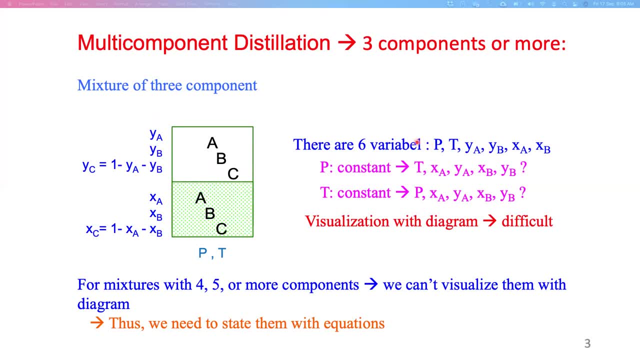 many components, for example from the crude oil. of course they have a lot of components, so then the variable would be really so many, Yeah, So here at the P constant, then we have a T, but then also there are a number of parameters: Y, XA, YA, XB and YB, Right. So even in the T constant then also 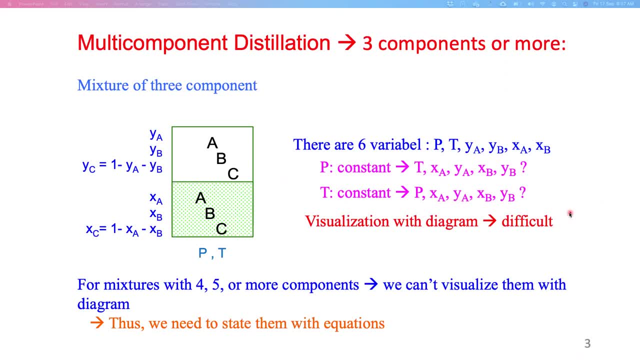 there are minimum five variables. So because five variables? can you visualize it using a 5, using a 3D diagram? What do you think? Can you visualize it using a 3D diagram or two-dimension diagram? Yeah, It's really hard. Yeah It it, may it it it maybe can. yeah It it, it might can. but we have to set the. the other, maybe two should be in constant. Yeah, So we have to slide it. So we have to put maybe XB and YB constant then. then we can again construct different. So so, but because with every changing XB, 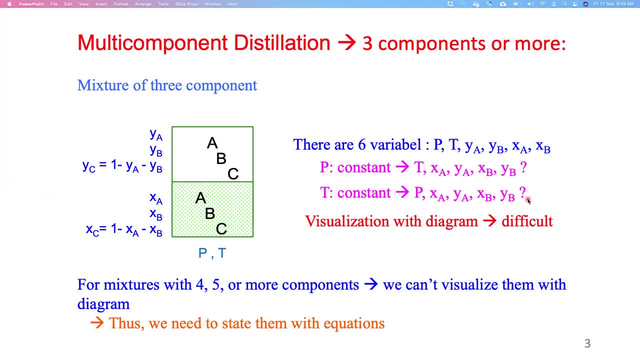 every changing XA and YA. of course it's going to be difficult with the diagram. So for the multi-component distillation, we're not going to do it using graphically but we're going to use it using equation. Yeah, So we're going to have a set, some set of equations, So we're going to try to visualize with with those equations, to solve those problems and also to check the, the, the, for example. 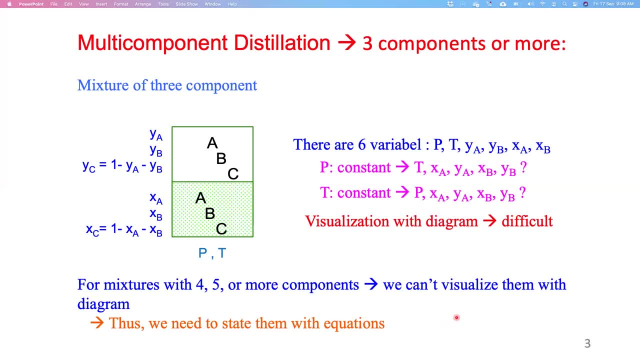 to find the equilibrium stage, to find the reflux ratio, to find the, the number of stage. yeah, to find the intercept, for example. We're going to use it some with some equation, Okay, The equation that that also accommodate those variables. Okay, Right, So let's, let's go to the next chapter. Okay, So. 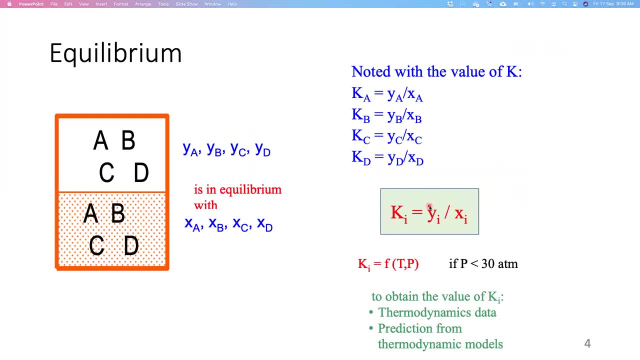 So let's see here again. So for the equilibrium, because we can't visualize it with the two-dimension diagram, we can visualize it with. you can visualize it with the. if there's any problems with that, it will be okay. 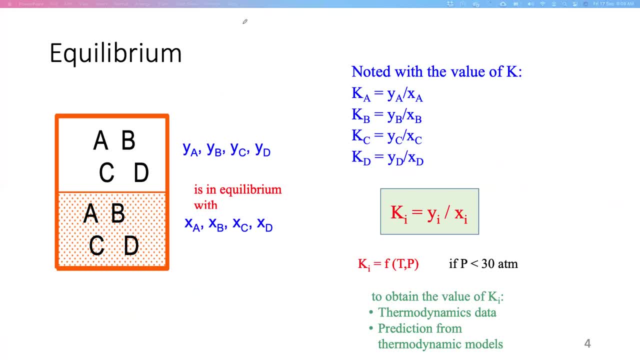 XY-diagram: Yeah, So in two-dimension we can have XY-diagram, for example: Yeah, Equilibrium. But for three or four or five components we can't visualize that because there is a dependent. yeah, there's a correlation between y a, y, b, y, c, y, d, x a, x, d, x, c a. 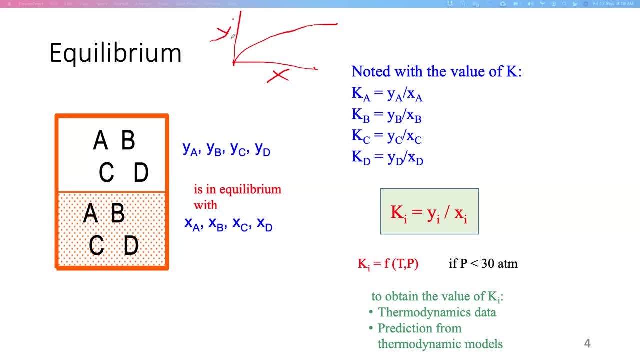 t. so because of that, we're going to use this one, the the value of k using k value. yeah, do you know about k value, is it? uh, have you? have you learned that about k value in the termo, in the thermodynamics? hello, is it something that will guess it? 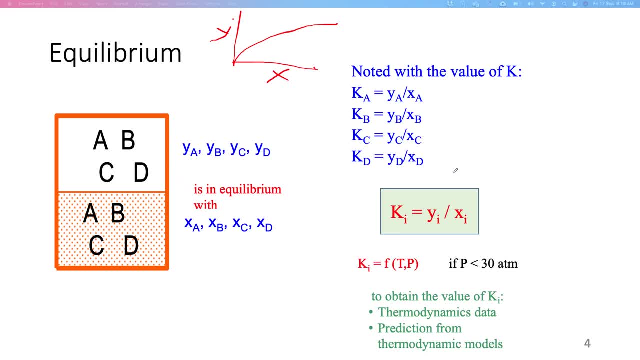 no, a little bit different. oh, you know, you're not the fugacity, yeah, uh, yeah, okay, all right then. so if it's not about, if you haven't learned about that, so i'm gonna introduce this k value. this gas value is actually: uh, um, this one is actually a ratio between the 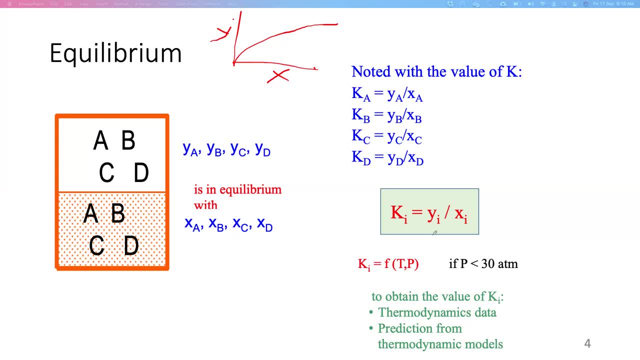 fraction in the component of i in the vapor phase. divide that the mole fraction of i in the liquid phase. okay, and this k value is a function of temperature and pressure. okay, so we're gonna use this one okay value, uh, so, uh, and then after that, uh, this, uh, later would be. 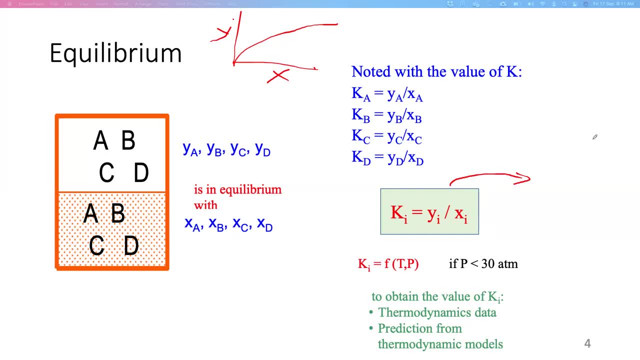 uh, and then to to check also the relative volatility of each. uh. i is actually- later i'm gonna introduce a term of relative volatility- hi, uh, this is actually the k, uh i, divided by k, h, k, a heavy key. i'm gonna tell you later, yeah, but anyway, uh, this is the one that you should. 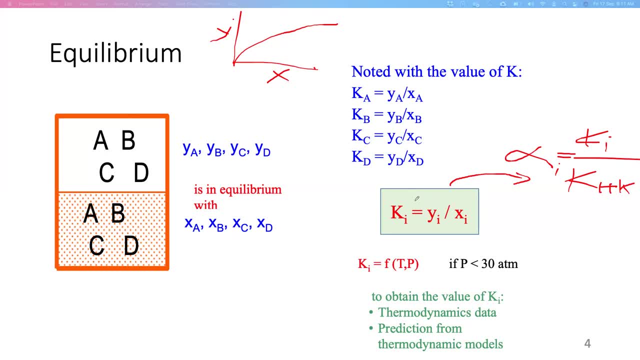 uh start to getting along with, which is, uh, the k value. and because k value is gonna change this correlation, uh, this is base. actually, if you have in this point, you have uh composition in the equilibrium in the vapor phase and also equilibrium of in the liquid phase, okay, and then this point is: 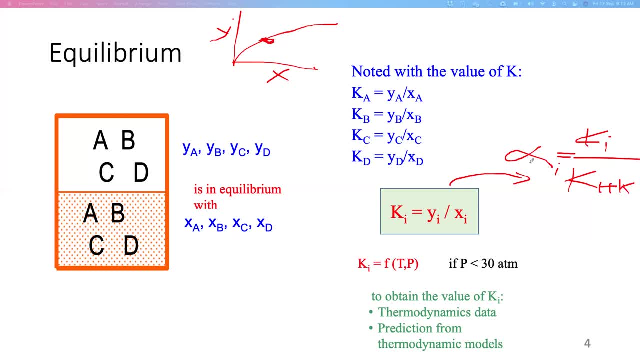 changed this point into this point, so, and then in the liquid phase, and then this point is changed into this K value. okay, and to obtain the K value, it is based on the thermodynamic data and also the prediction from thermodynamic model and also all of the 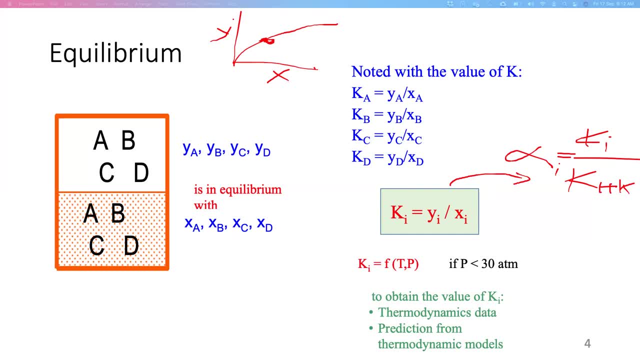 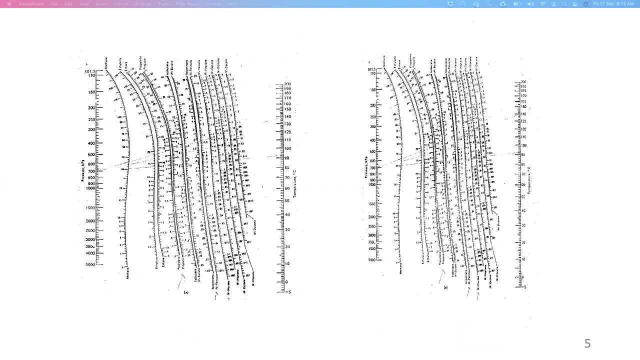 heavy database. we also can have it in high six. yeah, that's why maybe after a few weeks after this, we gonna introduce high six to so, because we also can find the K value in high six. but but it's basically it based on all the database and then they put it into the software, right, okay, this is too big, so small. let. 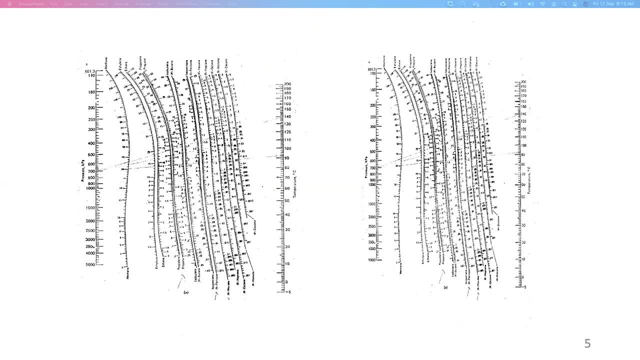 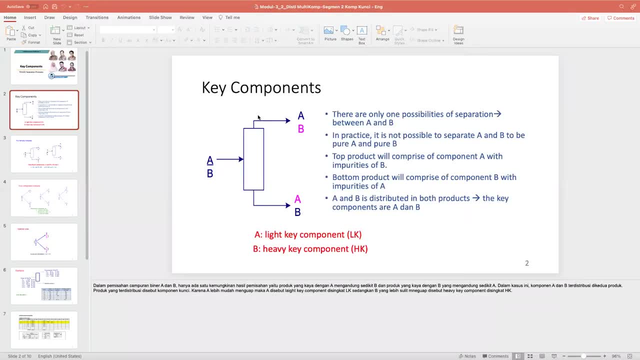 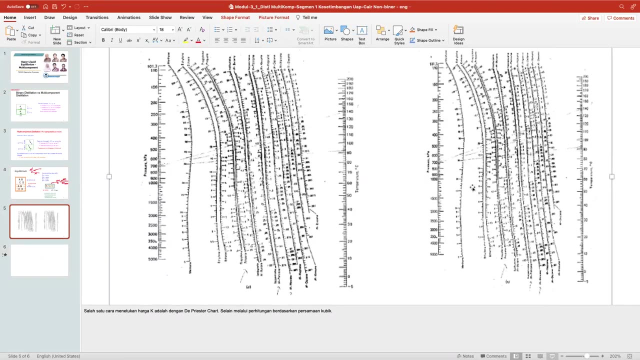 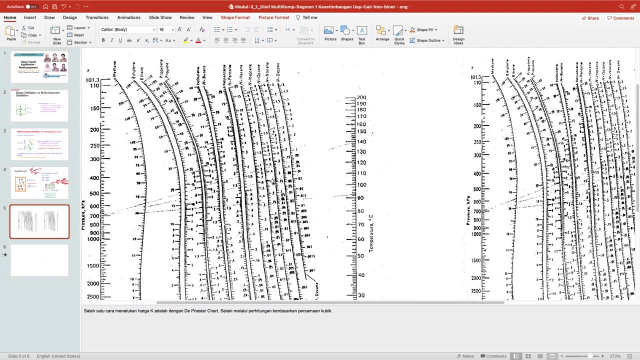 me and show, and then let's have a look on the each component. right, let's make it bigger, okay? later I want you to print some of this and also, or maybe, if you can do it using a line, using here is also fine, but okay, so for 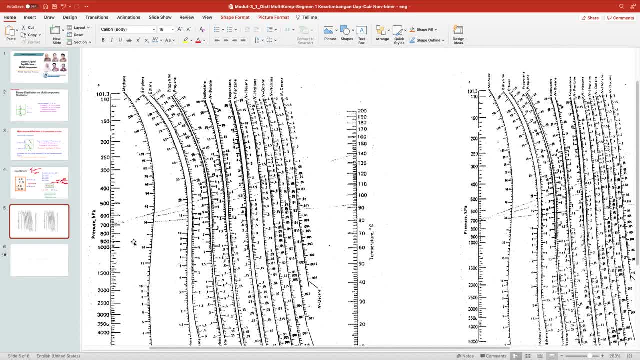 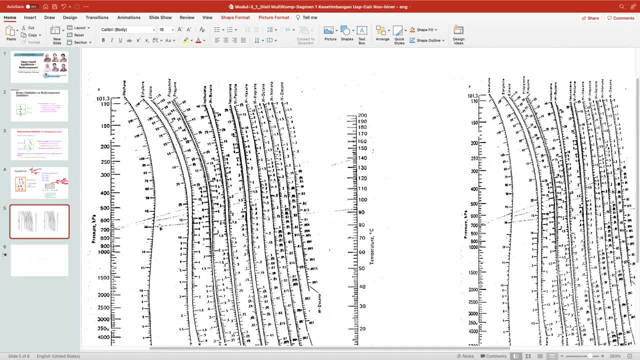 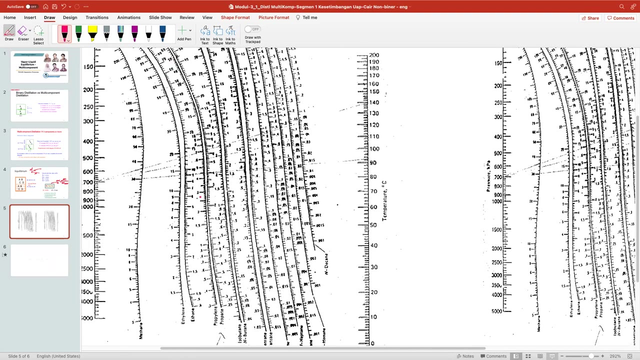 example like: yeah, let's make it bigger here, right? yeah, so this one is a very old nomogram. I think I took it also from thermodynamics books. so if, if you look at around here, there is a component, the name of the component can you see? can? 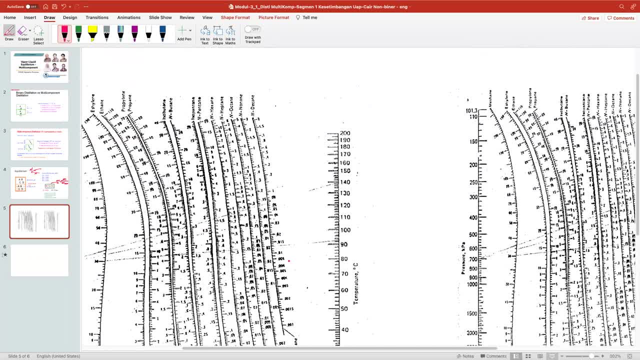 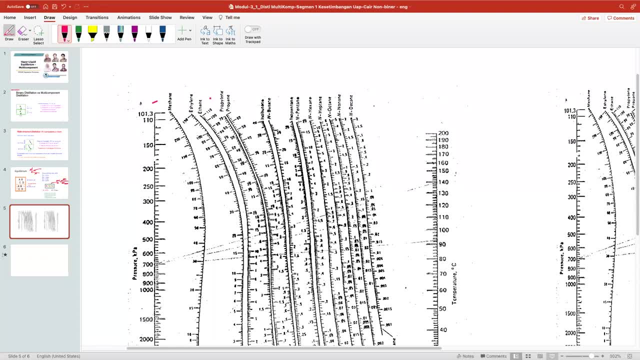 you see, yeah, yeah, yeah, it should be a little bit bigger. see, there is a methane, there is ethylene ethane, propylene, propane ice, So butane, n-butane, isopentane, n-pentane, n-hexane, n-heptane, n-octane, n-nonane and n-decane. 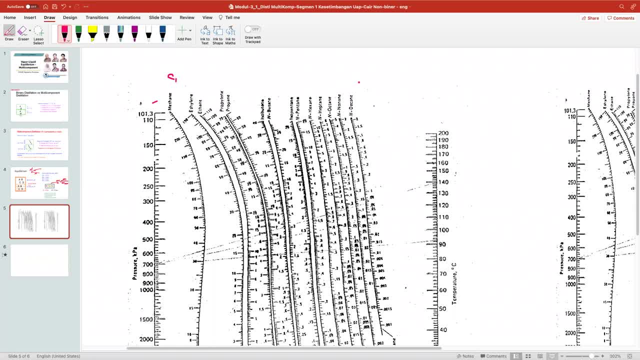 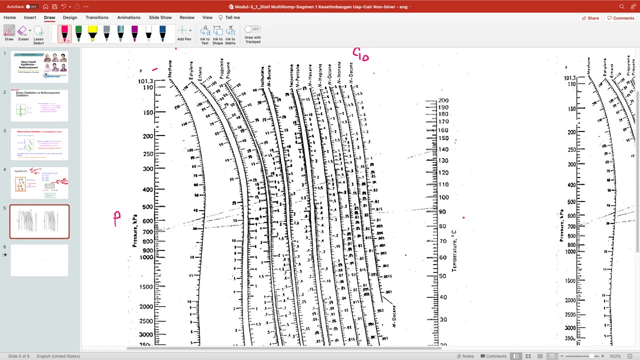 So it's basically from C1 to C10.. So all of this ruler, the curve ruler, here are the scale for the K value for each hydrocarbon. In the vertical one you have pressure and over here you have temperature. So remember, let's have a look. 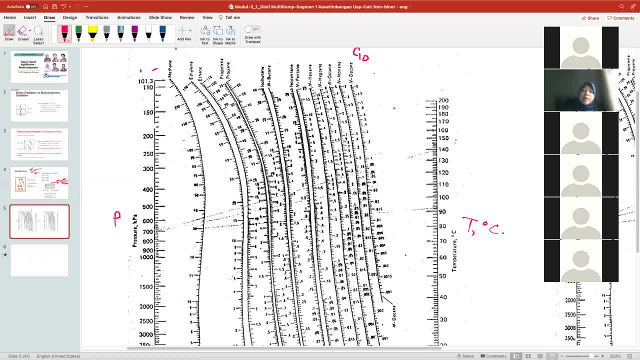 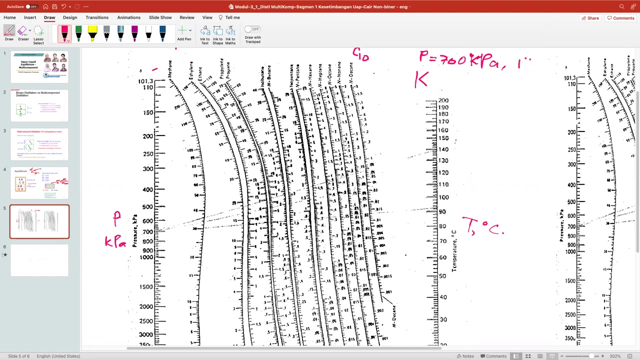 So let's check. don't forget to check the unit. so P in a KPA and also temperature in a degree Celsius. Now how to read the K value of, for example, at the pressure is 700 degrees 700 KPA at, for example, at 150 degrees Celsius, for example. 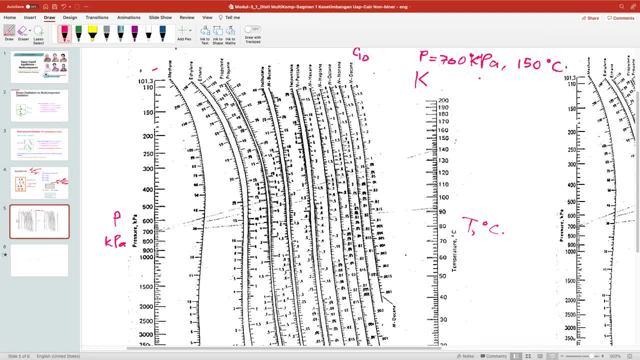 So what is the K value? So what we're going to do is we're going to put insert again line from the pressure of 700 around here to the temperature Which is about 150 degrees. Okay, got it. Okay. 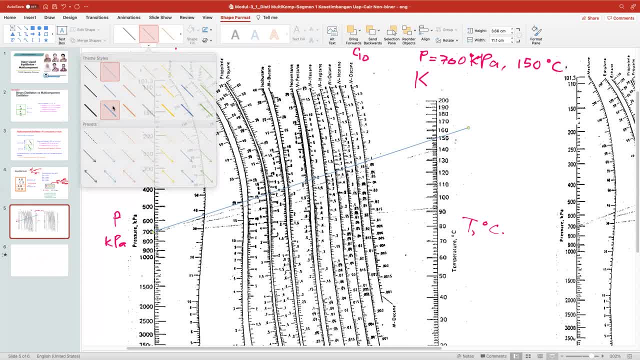 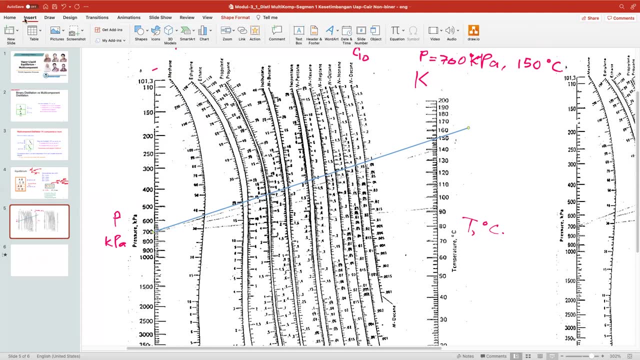 And then maybe make it a little bit bigger there. Okay, Oops, too big. Okay, yeah, can you see the line? And then now you can read the K value for each component. Yeah, you need to do it manually, because now we are training you. yeah. 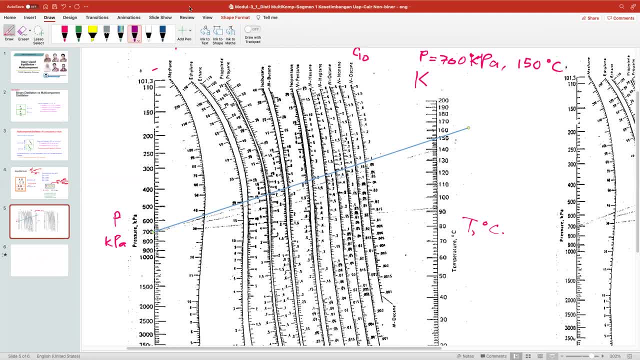 We're training you to, To understand, but later, when you do it in, for example, final project, or in the, in the operation, in the, if you're, for example, when you are at work, of course you're not. you're not going to do this. 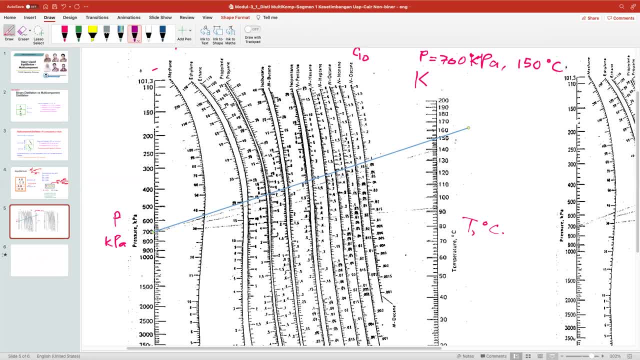 Yeah, you're. maybe you're going to use the high CIS, but before you you're using the high CIS, you should know how to really get it using manually, Right, Okay? So what is the K of the? let's have a look. 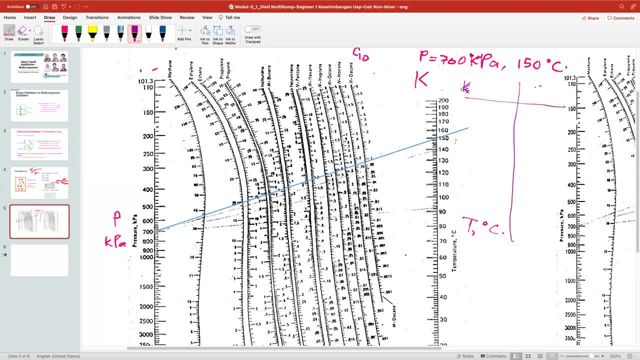 So maybe let's have a have a look. So what is the K value? And then this is the, the component, Yeah, C1.. Then we can read it here: Okay, I can't really see. So this is 50,, 40,, 30.. 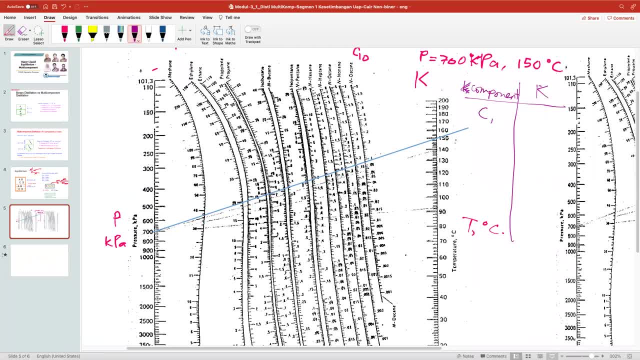 So 30,, 32,, 33,, 34,, 38.. Yeah, around 38.. Yeah, So so for C1, the K value is 30.. So so for C1, the K value is 38.. 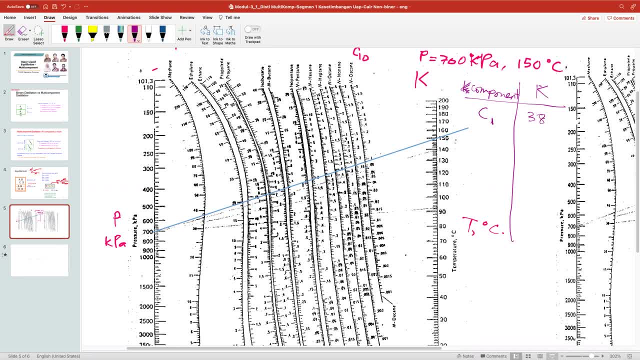 Yeah, Over here 18.. Yeah, This is ethylene, This is 18.. So maybe around this one- It's a little bit difficult to see it- Maybe around 10. 20. It is 20. 10.. 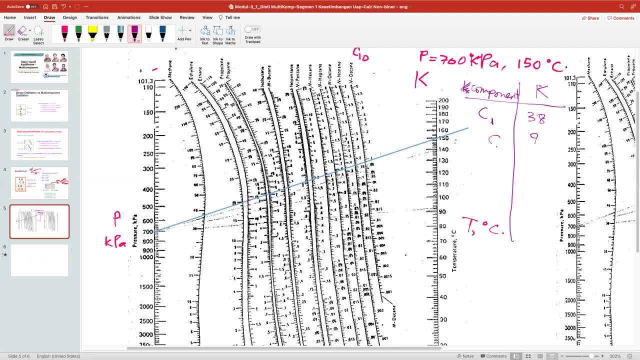 Maybe around 9.. Yeah, And then look at the propane. Yeah, This one, And it's getting along. yeah, This is 15, 10,, 9,, 8,, 7.. This is the C3. Sorry. 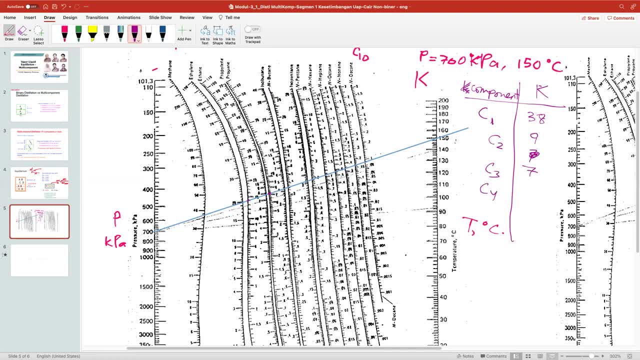 This is the C3, 7. And then C4. And we attain maybe about 5,, 4,, 3. So maybe about 3.6.. Yeah, Um, Uh, For the assignment. of course I'm going to give you the more clear yeah compared to this one. 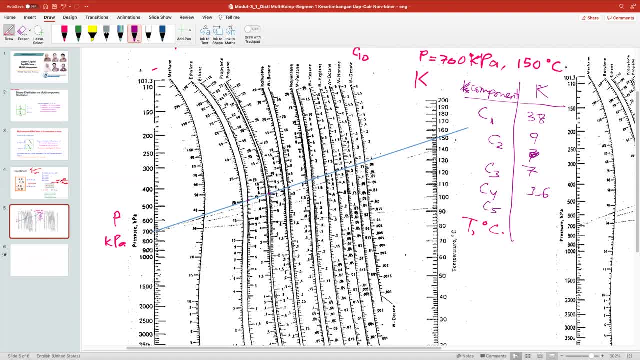 Should be much easier. You have to make it clearer. And then, this one is 1.5.. This is 2.. So maybe 1.9.. Okay, For example. Okay, So this is an example: How to reach the component at a certain pressure. 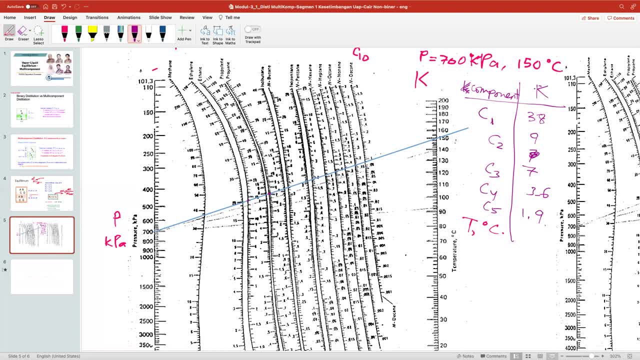 At a certain pressure and also uh temperature. yeah, um, what can you uh see from here? Uh the K, what can you, what can you see from this data? The K is decreasing. K is Decreasing. 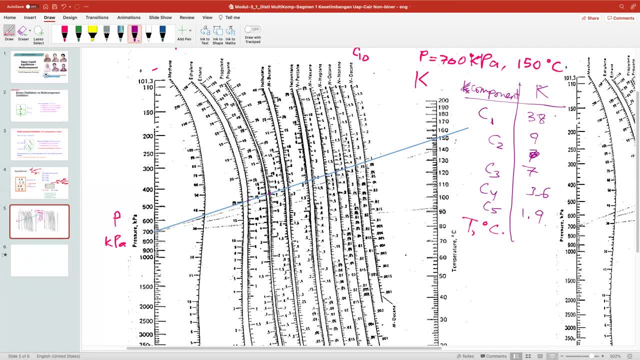 Increasing with, I mean decreasing with, Oh, decreasing, Oh right, Yeah, Uh, uh. K is decreasing with the increasing number of molecule. Yeah, You mean, Yeah, Okay, Uh, right, So you can see, the C, uh, the C one is the the more volatile. 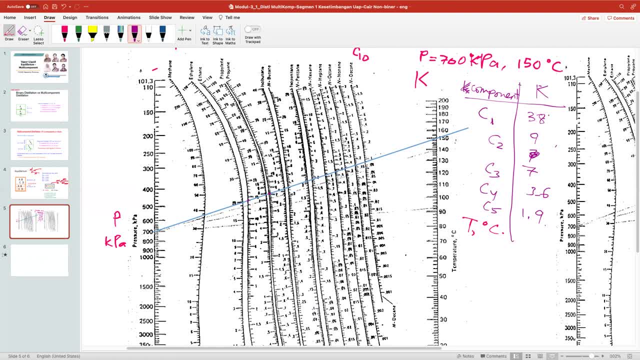 Yeah, So the, the, the higher K is, that means that the, the component, is more volatile. Yeah So, uh, later, when you, when you have this type of K value like this, then you can write that This becomes your A component A, which is the more, the most, uh, volatile. 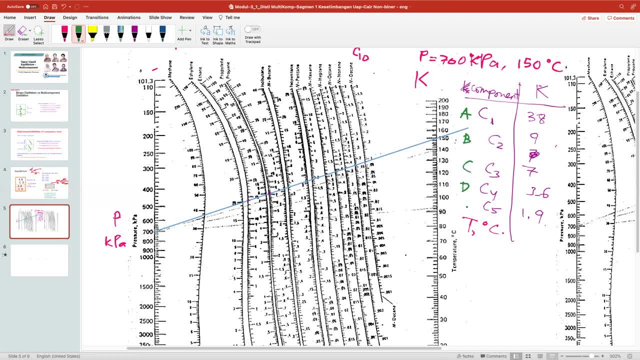 And then this is the component B, This is the component C, This is the component D, This is the component E. So the numbering for the components we got we're gonna look at from those K value. If the it is uh, the, the more volatile it is, which is K, uh, the higher K means that the, the fraction would be much more in the vapor phase compared to the liquid phase. 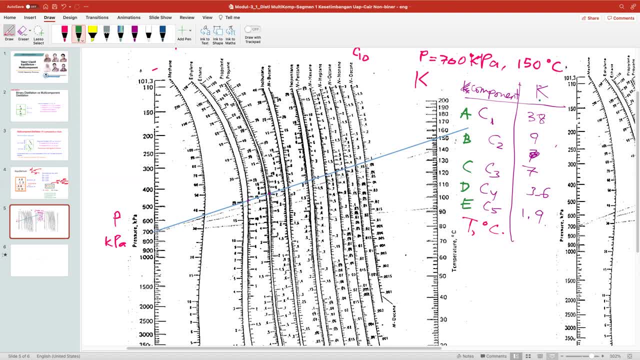 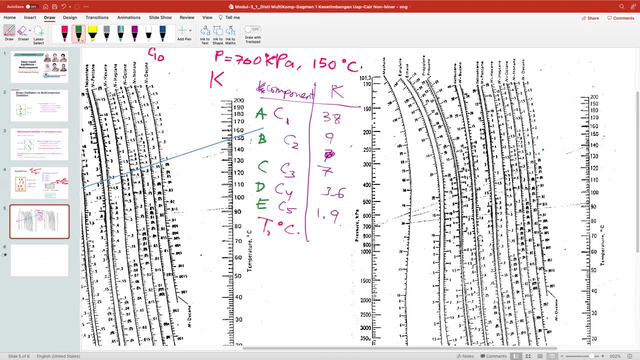 Right, So The higher K is the more volatile of those components. Yeah, Uh, over here. uh, let's have a look. It's also similar, but but at lower temperature, I think, and also at higher pressure. 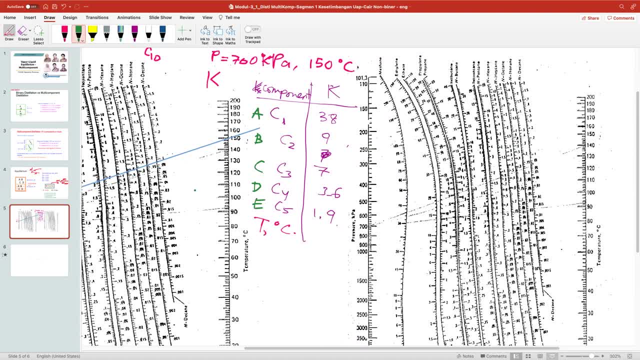 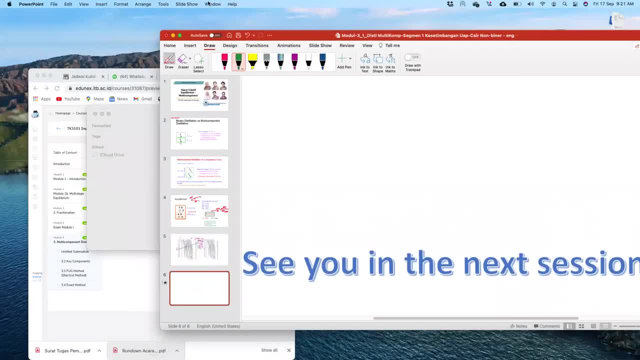 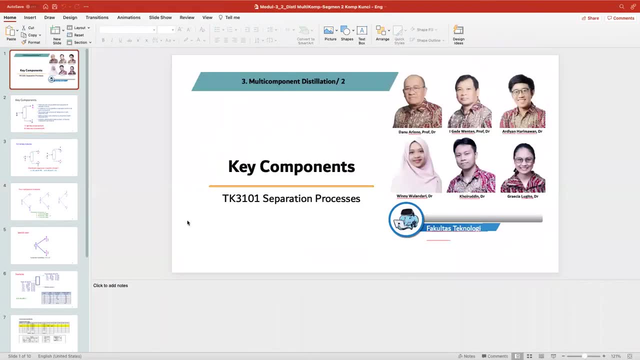 So you can also have: look, uh, with that one there. All right, Uh, so this is the end of the session, so let's uh go, let's have a look on the next module. Right, Okay, Um. 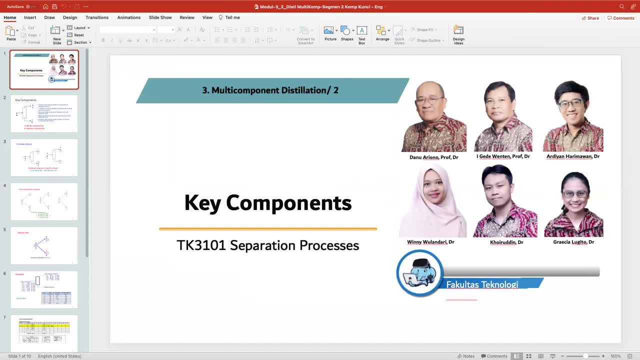 I'm going to see, uh, like you see that my pen looks funny when I uh put it full screen. So, um, I want uh, yeah, I, I want be in the full screen now, So then I can write something here. 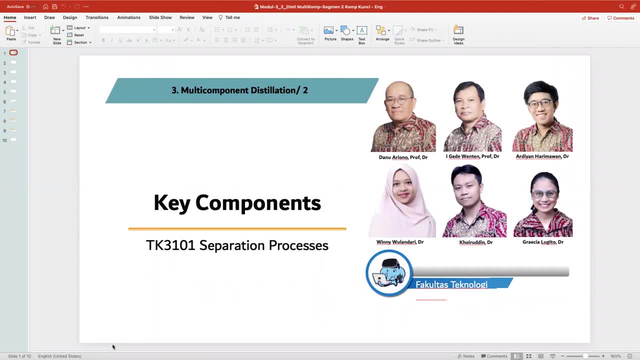 Okay, Now, once we know about the, uh, the concept of multi component distillation, why we have, uh, four, why we have four components. Yes, Okay, Let's see, Okay, uh, we need to have a k, yeah, okay, the k value to get the equilibrium now let's have. look about the. 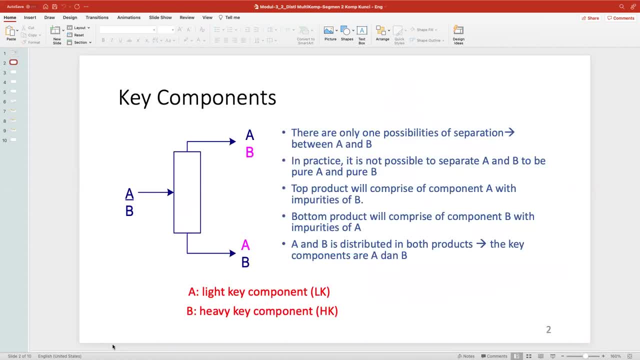 key component, component kunki: yeah, so what is the key component? okay, um, what is the concept of key component? it actually happens also in the binary distillation. yeah, if there is only uh, if uh, for example, if it is only binary distillation, um, uh, you know, uh, there's one possibility of separation. 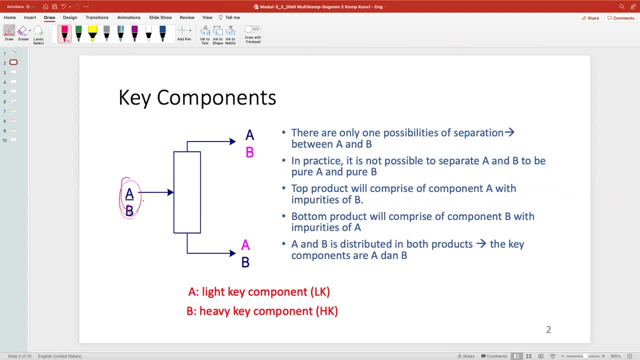 between a and b. yeah, this one is the. the separation is around here, okay, uh, of course, in practice it's not possible to separate a and b to be pure a and b, so the top product would be comprised with component a, with a little bit of impurity for b and component b. 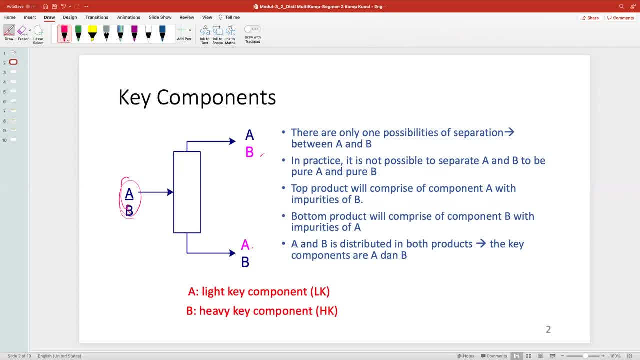 also would have uh have impurities of a. okay, um, so, uh, at this point, uh, a would be the light key component of uh light key component in the bottom product, yeah, and b is the called the heavy key component in the uh distillate. okay, so, uh, usually, uh, we, we check the, the the requirement in the problem in the problem uh. 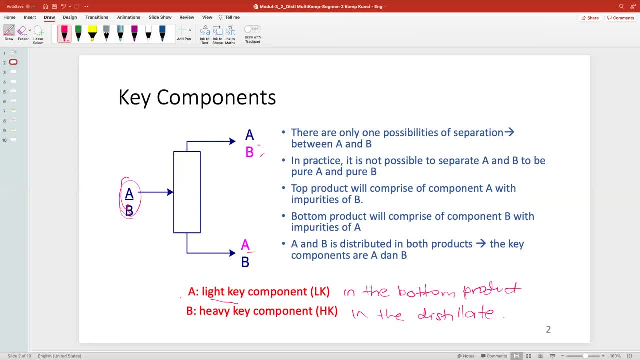 that is assigned uh, how much the lightly component or how much heavy key component we want in the process. for example: okay, i want a product which comprise of 99.95 percent of a, so it is locked that the heavy component, yeah, the heavy component which is b in the uh distillate should be 0.05. 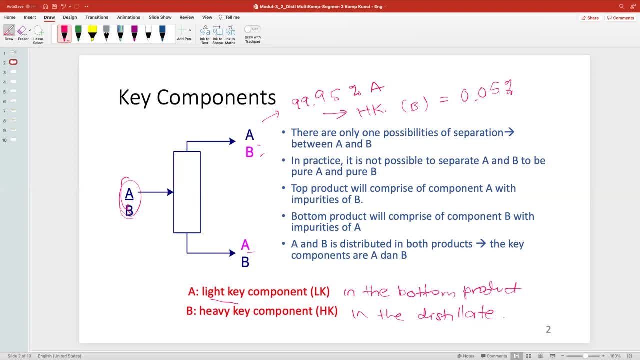 yeah, we have to require that. we have to lock them because it's a key component. should be uh, 0.05 or maybe less than that. yeah, if we have the product, uh, our uh tower or our equipment has more than the requirement, that's fine. yeah, but we have to lock the minimum requirement. 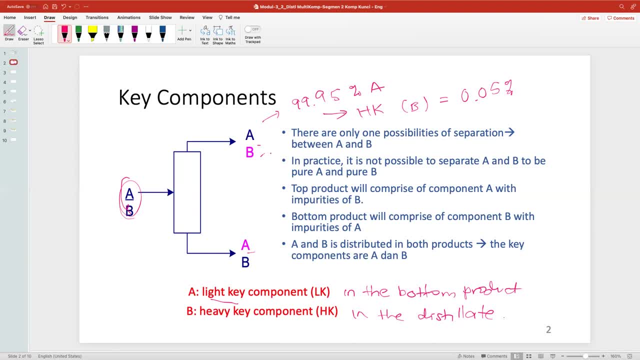 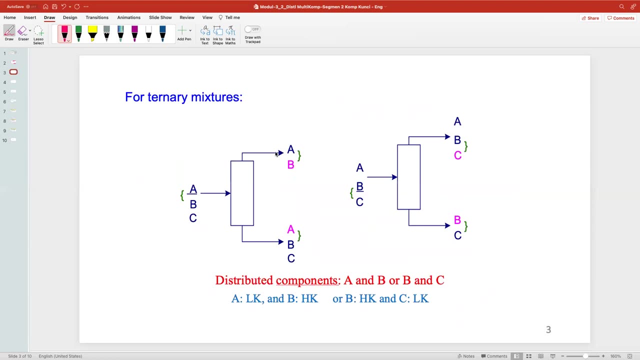 as the product, so the our product should be on spec. all right, uh, this is for two components, which is? uh, there is only one possibility, yeah, between a and b um. now for tannery mixture, uh, this, the distribution, or the. yeah, the distribution, it can be, uh, the distributed component, it it. 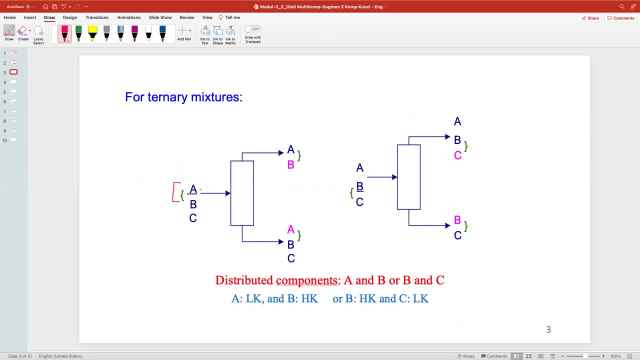 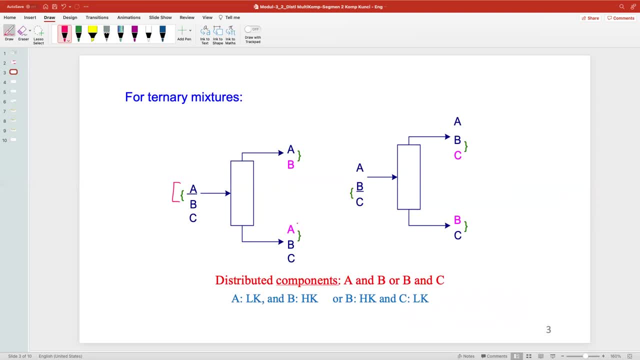 distributed in the uh bottom, yeah, or maybe b, yeah, so there are two, uh, uh, two opportunities here. yeah, there are two type here. uh, there's a scenario or b or c. b and c is distributed, so so that means if, if this is the key components, that means we gonna 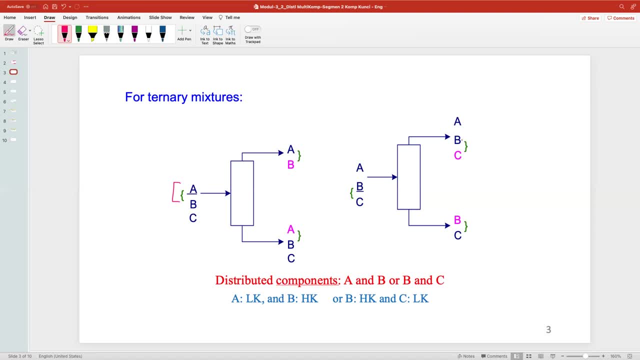 have a, of course, at the top product and uh, b and c. uh, here b, and then little bit of c in the distillate and, yeah, in the silly, while in the bottom then we have, we're gonna be a little bit of b. okay, so in. 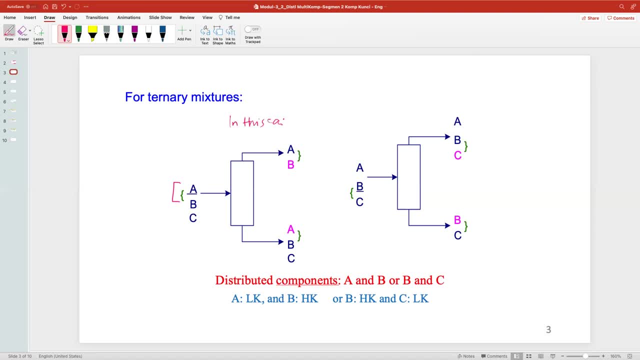 this case, What is the heavy key? Which one, B or A, B, B? but why B? It's impurity in the distal Right. okay, okay, Nazifa, Because it is separated between A and B. so heavy key is the most heavier component. that's important and that is present in the distillate. 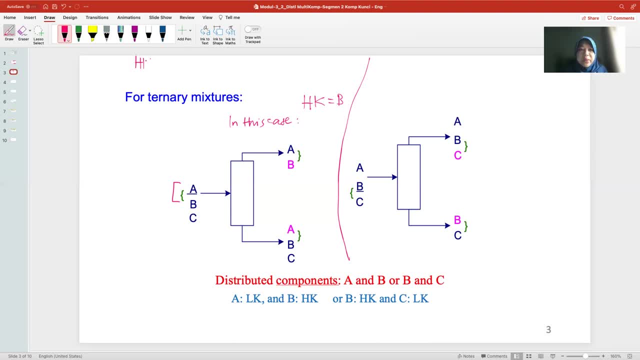 Okay, so I'm going to write it here, because sometimes you need a little bit of a concept. So heavy key is the heavy in important component that's present in the distillate. Okay, so heavy key is the heavy important component that is present in the distillate. 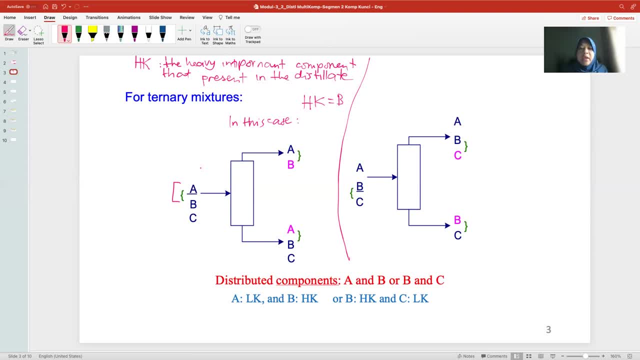 Yeah, I have a question When I see this one. I have a question to Pak Danu. Pak Danu, how to determine which one is the heavy key, Is it B or is it C? And Pak Danu said that if we have a number of components, it's actually going to be specified in the problem or we have to extract them from the problem. 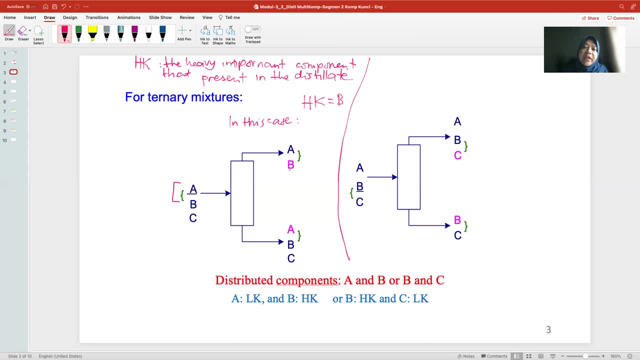 I mean Usually in the specification of product. there are some important impurity. There are some important impurity that is very important, that must be present in the product. If it is more than that, then the product is on spec Yeah. 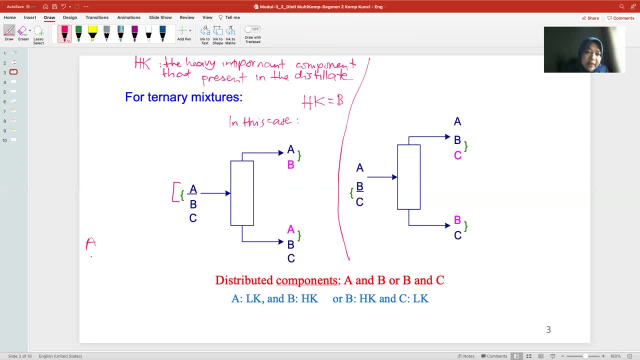 So then for heavy key, so for example there are one, two, O, A, B, C, D, E, F, for example. Yeah, So it might be happen that sometimes the heavy key may be, for example, around this one. 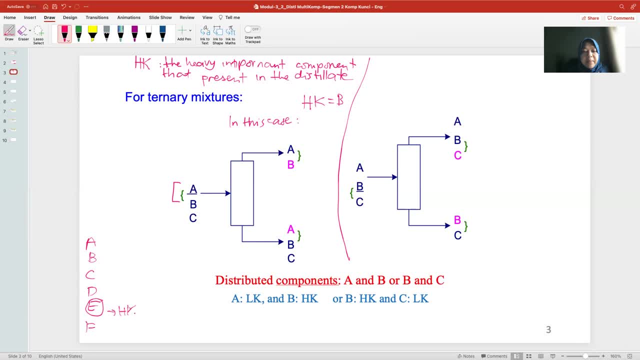 For example. it may be applied. an example. Or maybe for the light key should be, for example, this one: It might happen. Okay, So this is all right example. So with this definition, we can conclude that Heavy key is the heaviest important component that is present in the distillate. 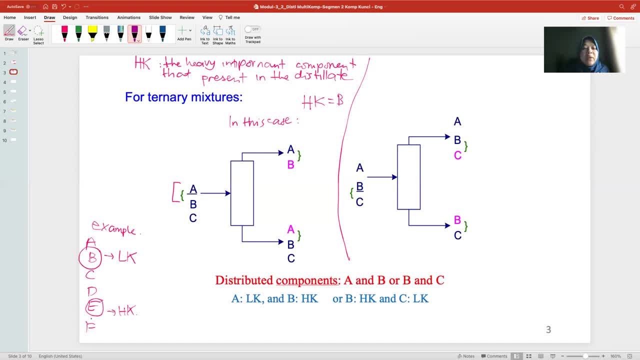 What about F? Maybe F doesn't present in the distillate? Yeah, It would be. maybe it would be, but very, very, very tiny and it's not important for the specification of the product. Okay, So that, for example, this is: A is the heavy key. 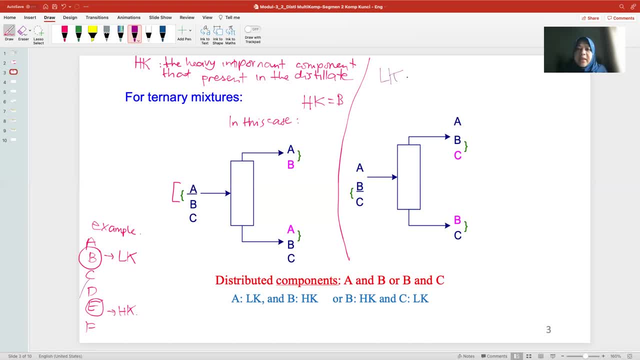 Now, with that, what is the light key? Yeah, Contrary to the heavy key, the light key is the light important component that must that present in the bottom product. So the light important component that present in the bottom product. So the light important component that present in the distillate. 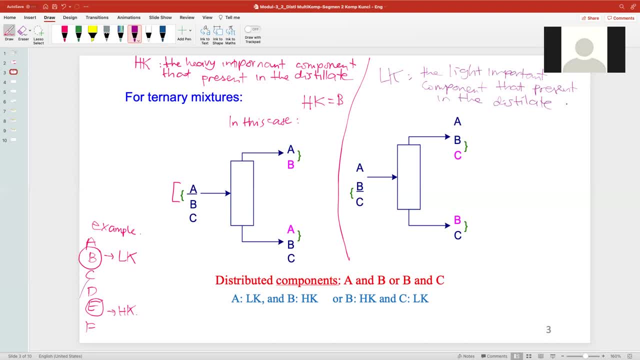 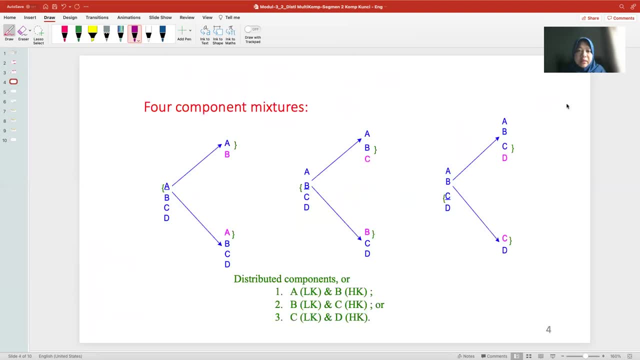 Yeah, Okay, So is it that you only can have one type of heavy key and one type of light key? Yeah, Usually like that, But sometimes there would be some distributed later on. I think This one. There's some special case that this is distributed. 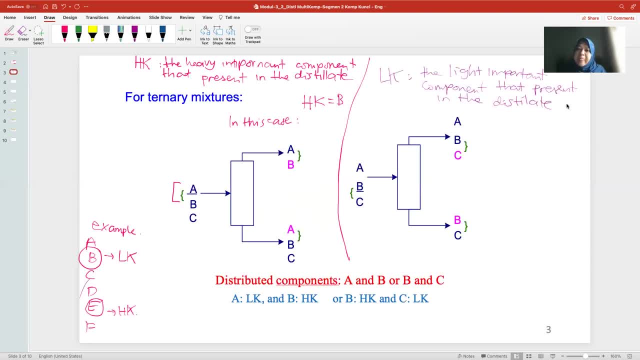 But ordinary, yes, Like this, So, yeah. so for example here: yeah, let's look at this example so you can see the big picture. So if I have five components- A, B, C, D, E and F- for some reason, for example, I want all of the B goes into the distillate. 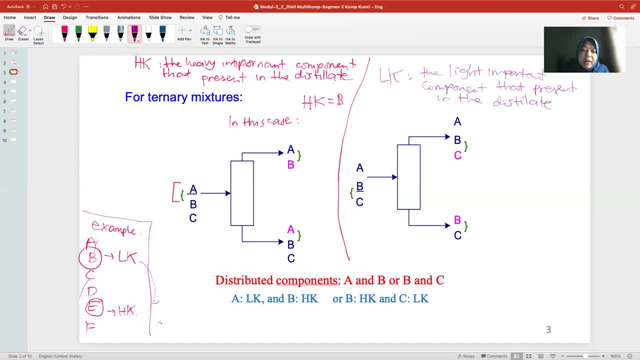 So I only want maybe 0.05 should be only left in the bottom product because this is so precious. For example, yeah, any A present in the bottom product, that's fine, I don't care. But B, I only want 0.05% of B in the bottom product and all of them should go to the distillate because it's very important. 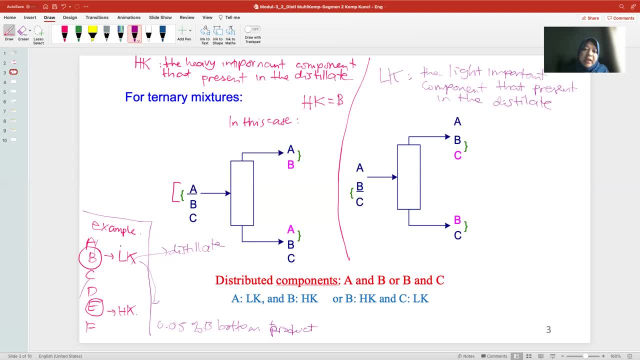 This is my valuable product, So the LK is the light key. Okay, Okay, Yeah, So this one there. Okay, Yeah, This is an example for quite more Five. Yeah, But for this case, this one here. so I'm just going to erase this. 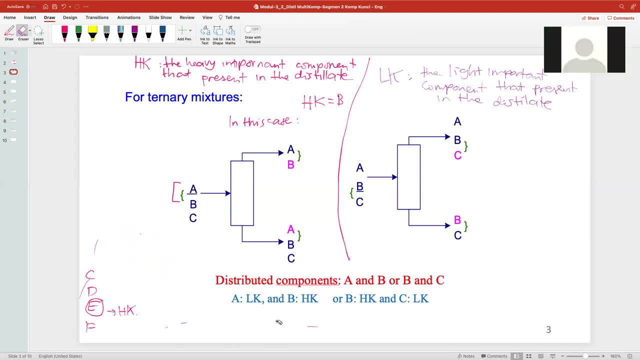 This is an example. I have a question. Yeah, yeah, So if, for example, you want B and C in the bottom product, B and C in your distillate, so it means both B and C are the light keys. is that right? 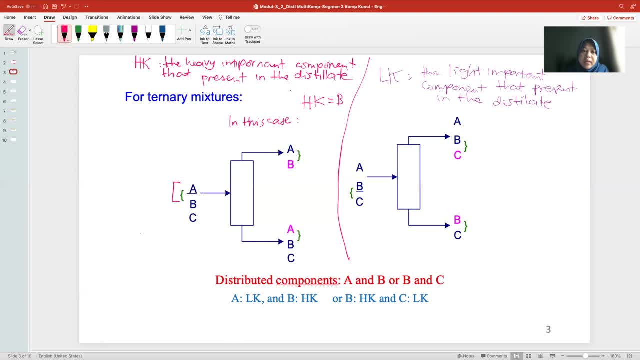 The distillate. you choose the heaviest one in the distillate. Oh, you can only choose one. Yeah, the heaviest bread. yeah, the heaviest. Okay, Yeah, good, If you want. good question: if you want A and B present in the distillate? 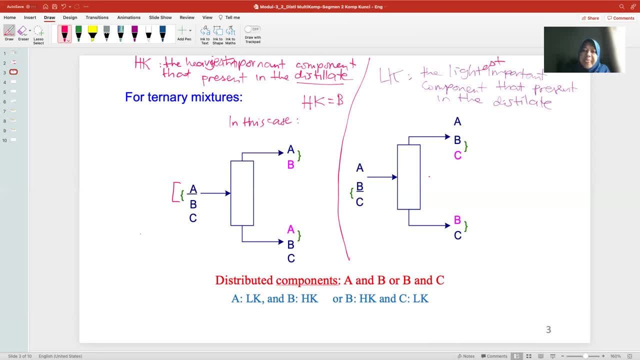 you choose. the heavy key is your heaviest one. That's what you call heavy key. That's why heavy key would be always in the distillate. Okay, so the distributed component. it can be A to B or maybe in another section, B and C is more important. 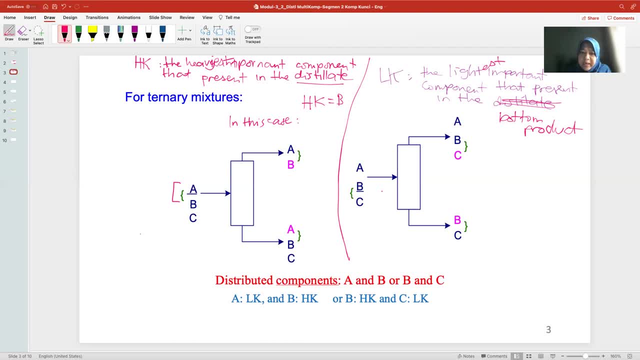 So The distributed component is A to B or maybe in other section, B and C is more important distributed component that we want is a, B and C, right? in this case, the, the heavy key is the B and the light key is a and for this case the B is the heavy, or this: 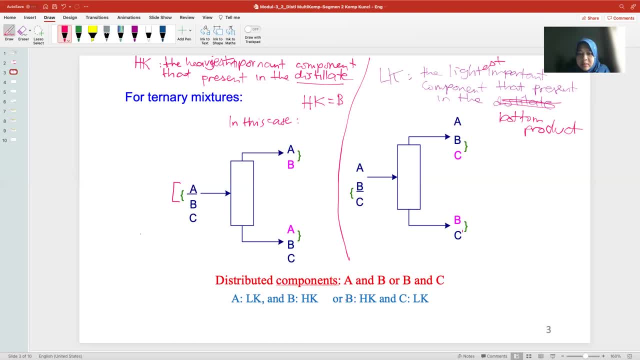 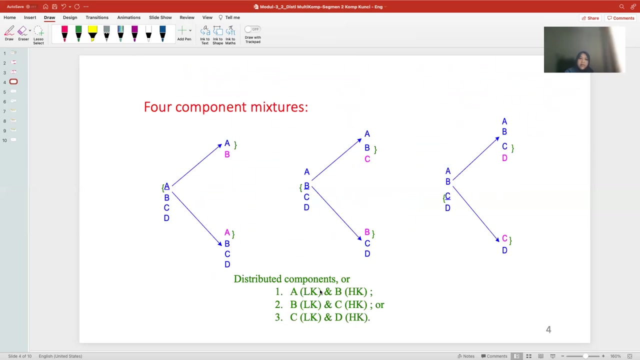 one, or should be C. yeah, C is the heavy key and then B is the light key. a is the yeah, a is the light key and B is the heavy key. right, all right, let's get one more. okay, four components. yeah, sometimes it can be also the four components here, okay. 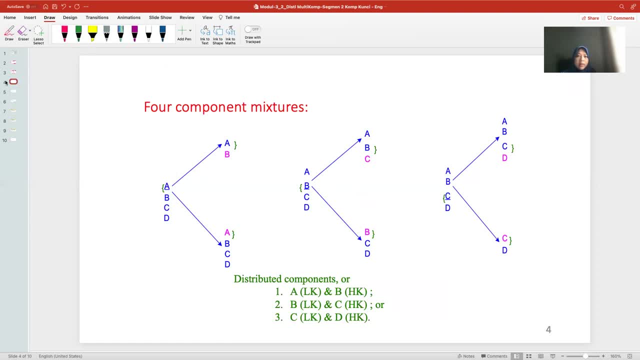 sorry, so I think looks like the heavy key and the distillate key should be the two components that should be similar. yeah, so my example before I have C 2 and C 5 looks like doesn't apply here, so so it should be correlated. yes, so the, the 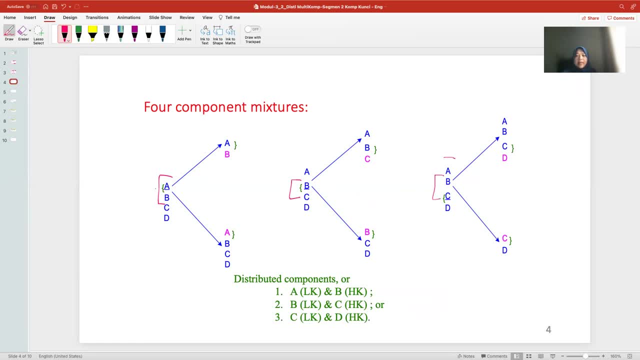 nearest one yang paling berdekatan. yeah, the, the distributed component that we want, between a, B and A, for example, or between C and B, or between D and C. so how are we gonna get that? usually it's based on the, an example. okay, and also like to answer the question as well. 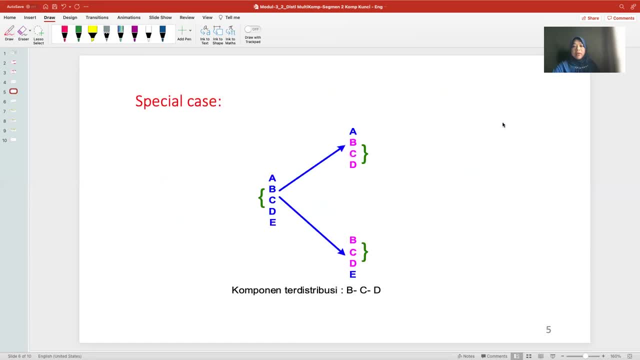 a question can also be answered onять. okay, and also like to answer the in. there are special case that where are three or more this component are distributed. usually that happen when the characteristic of those material, those components, are very, very similar, so it is usually always distributed. 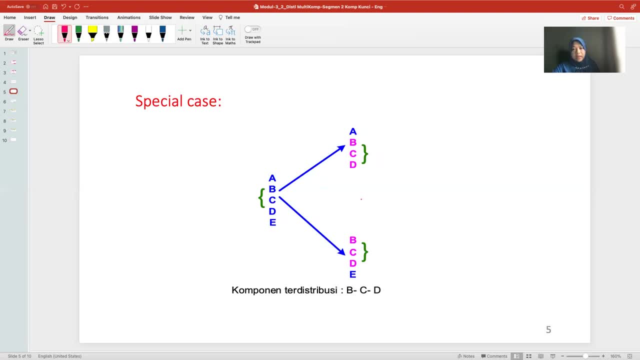 it would be present in the distillate and also in the button product, right? i have a question. yeah, okay, the other components other than the light key and the high key, how do we know which? where do they go like? instead of the distillate, or right? 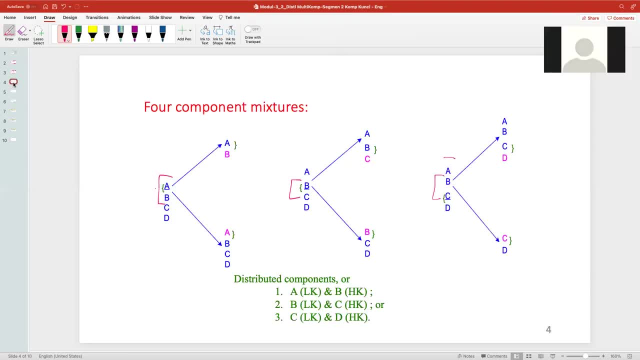 the component that is lighter than the heavy key always goes into the distillate. yeah, the component that is lighter than the heavy key, heavier than the light key, always go into the bottom. that's why, when you, we do the numbering, we have to be sure that we, um, we, we put the numbers. 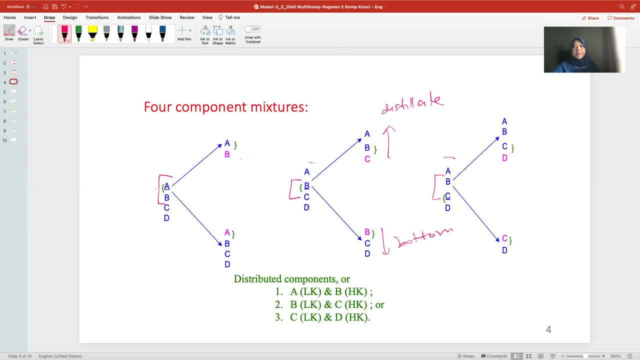 based on the relative, uh, the volatility. yeah, so a is more volatile than b, b is more volatile than c, c is more volatile than d. how we get it using those k value? yeah, check in one certain point which one is the more volatile one. yeah, for example, right, that one. 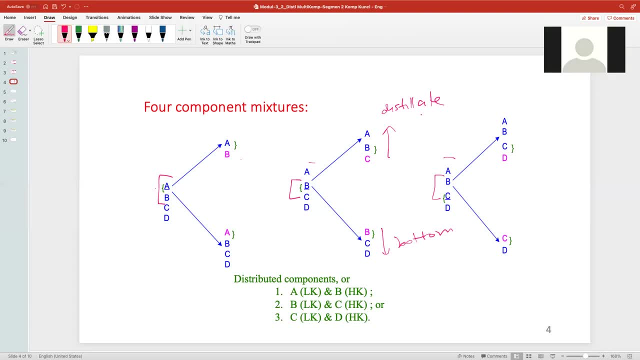 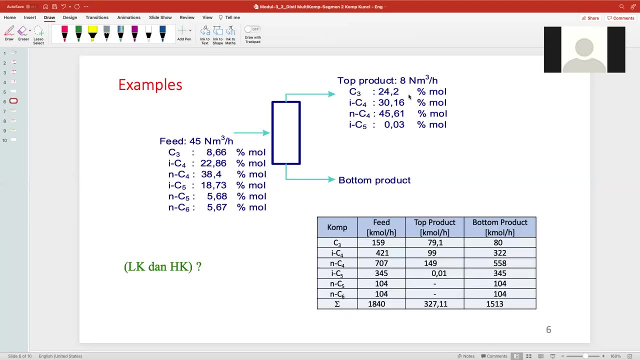 okay, is it answering your question, fatia? oh, yes, i understand. thank you, right, okay, and this is an example, okay, um, so, uh, that's very interesting. uh, this one here, um, we have a feed, yeah, we have a feed, um, which is 45 normal meter cubic per hour. 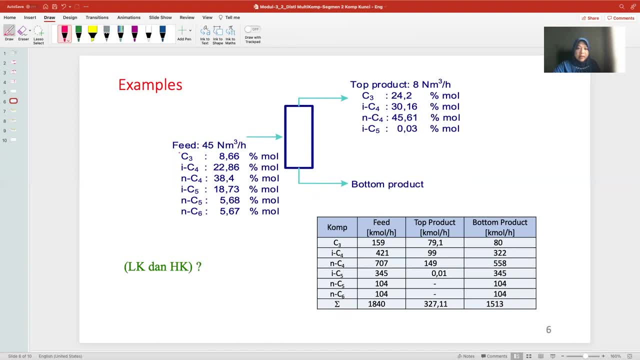 um, and then uh, this is this is the uh components. one, two, three, four, five, six, uh, from c3 to c and six, yeah, and then uh, it is a mole percent. yeah, and, and in the mole percent and this is the feed uh, usually if it is start from uh weight percent, then we have to change it into more percent. yeah, 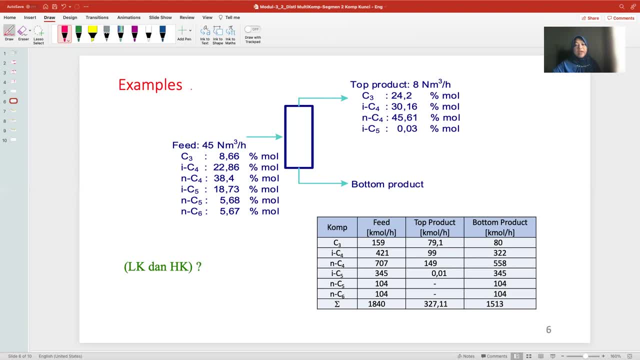 if it is known the volume, then you can convert them into the more percent or how many kilo mole per hour. yeah, so here the feed. uh, you change it to how many more, yeah, what is normal cubic hour? check again thermo: yeah, that is uh equal to how many more using pv and rt? yeah, 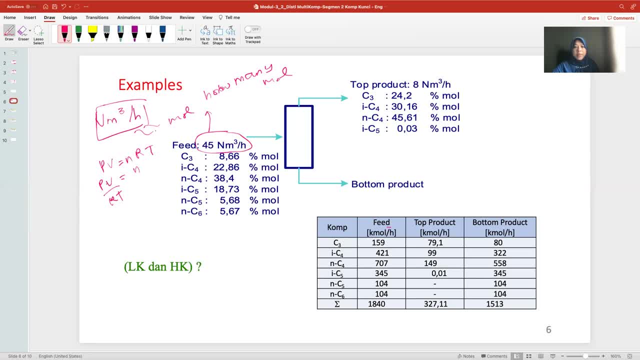 so you got the r, you got the uh p and t at the normal, and then you get the volume, and then you're gonna get the uh n, yeah, and then the feed is actually uh 1 840. yeah, based to calculate. uh, if you, if you're uh curious, you can check again the calculation. okay, based on the normal. 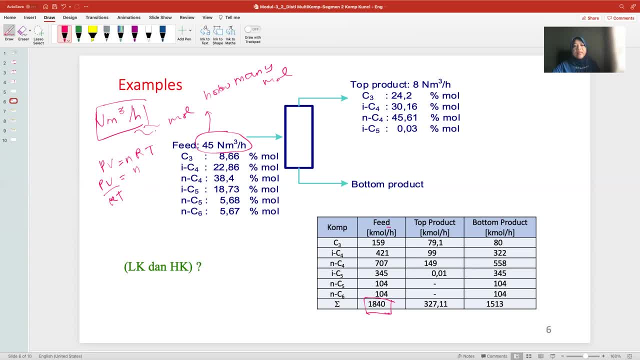 do you? uh, okay, do you remember what is the difference between standard meter cubic per hour and normal uh meter cubic per hour? what is the pressure and what is the temperature anyone remember? so the way i look at it is, even if the flow of water is 45 degrees, 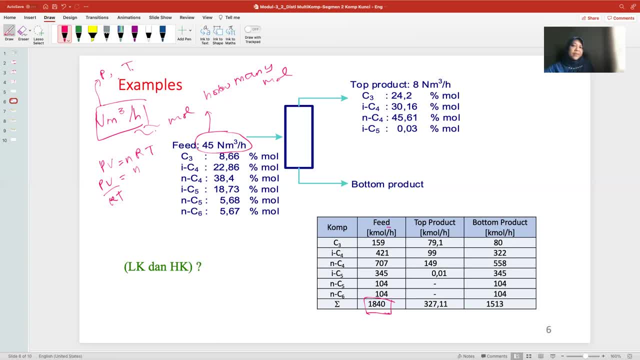 the. the flow of water is 25 degrees, right? or you can say that the flow of water is 25 degrees. it is 25 degrees for the, for the normal, or yeah. anyway, just please check. yeah, the normal normal is 20, if i'm not mistaken, 20.. yeah, if i'm not mistaken, normal is 22.. 20 or 25.. 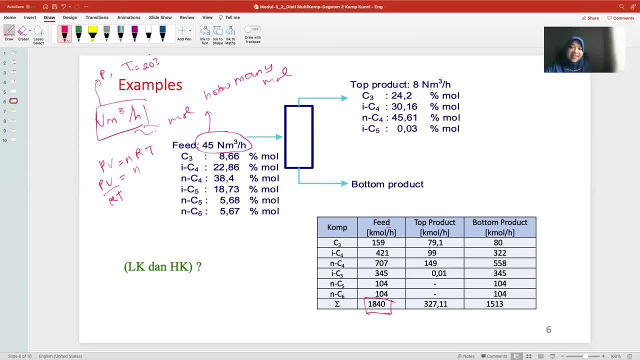 uh, yeah, uh, uh, yeah, it's been a while for me to check the thermodynamics. yeah, uh, i don't teach thermodynamics, so please, please, check that one there. but anyway, if you uh, kevin, if you want to check, uh, the total, from 45 normal cubic meter per hour it become, uh, 1 840 kilo mole per hour. 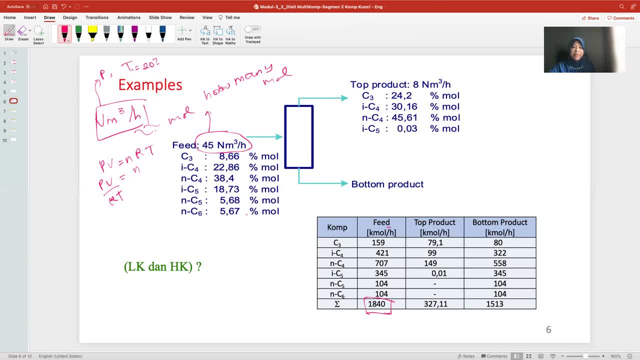 okay, and then you multiply it with the percentage of mole and then you got those feet. okay, let's say we want the product is: uh, the top product is eight normal meter cubic per hour with this percentage of mole. so using the mass balance you also can convert it. 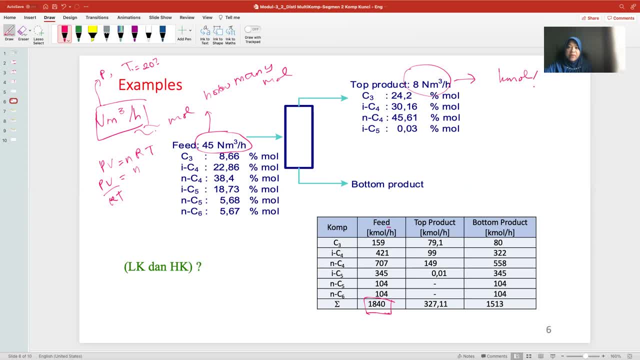 into a kilo mole per hour. and then you got here at three to seven, point uh 11, and then you multiply it with this one, so this is the top product. yeah now, um, in this case, like fatia said, or like kevin said, uh, so which one is the lk and hk? 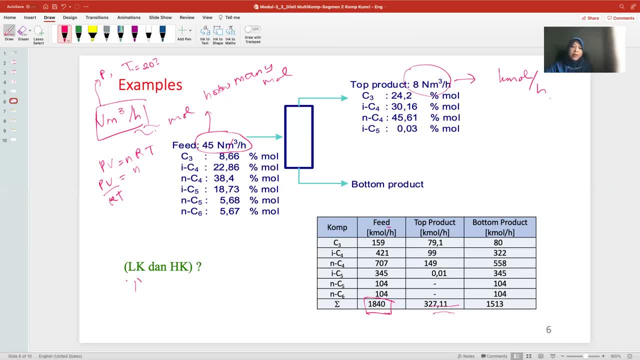 yeah, uh. so one important point: lk and hk is always distributed component. yeah, right, uh, falling the katana, yeah, for example, between a and b, uh, for example, for example, between c and d. yeah, the distributed components, okay, so uh, in here, uh, it's interesting. so uh, after this. this is from. 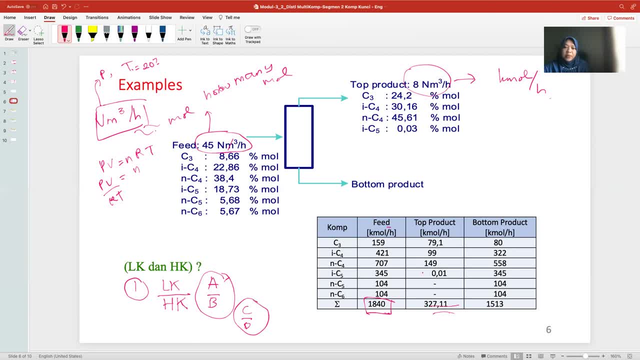 slide from pakdanu. so he calculates the top product and, based on that, and he can get the. this is the feed, this is the, the distillate, and this is the bottom. and how to get the bottom product, just uh, subtract them, yeah, from here to here. okay, okay, now, uh, the next step. so then, 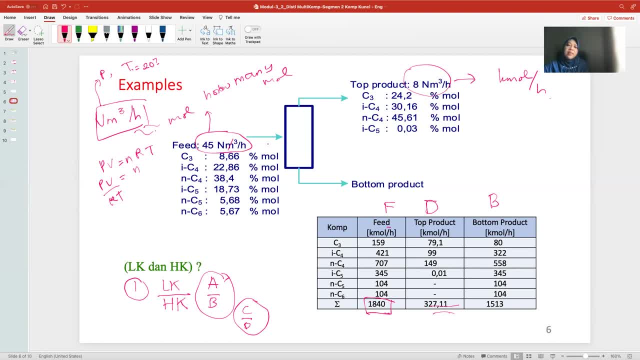 we have the bottom product, okay now. now, if in the problem it doesn't, it is not stated, uh, which one is the heavy key and the light key, then we can see: uh, so back again from: the heavy key is the heaviest important company that present in the 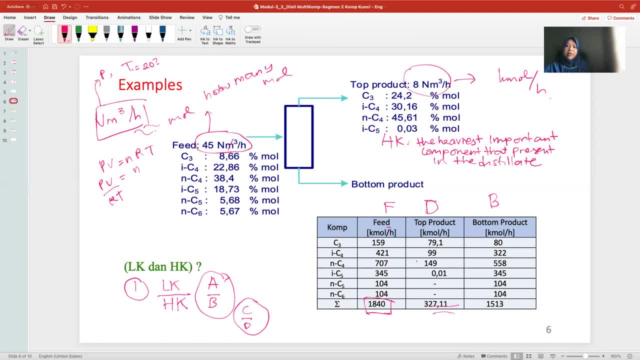 distillate. okay, so the heaviest one. so the heaviest one is between and c4, and i, uh, c5. yeah, is this a number? 0.01. this is a. this is, this is still still number. yeah, this is still quite significant. so, uh, then this. 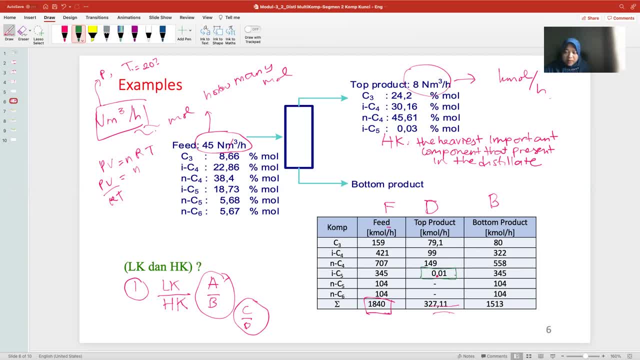 one is gonna be your heavy key. see the heavy key: the heaviest important components that present in the distillate and then in the distillate. so the heavy uh key is isopentane. okay, with that you can uh. okay, so then this is the uh heavy key. 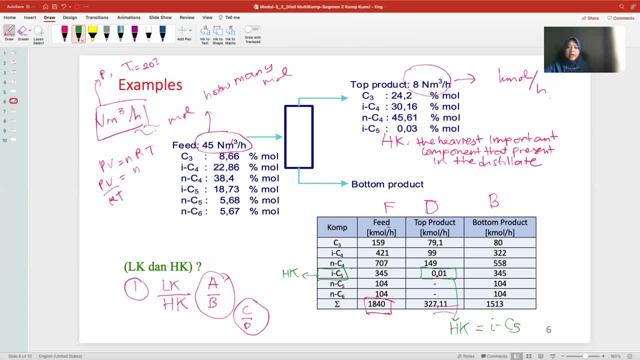 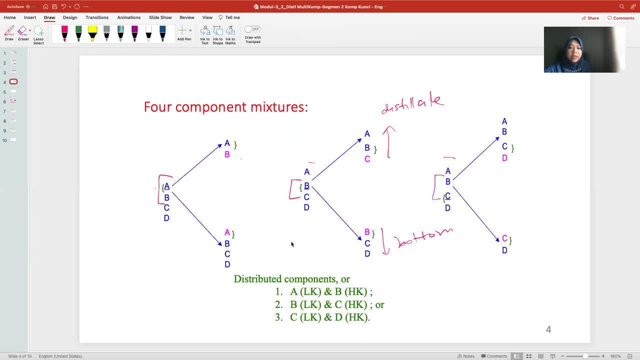 so, uh, what is the l key? of course the, the light key, is the, the one that distributed, uh, with the h key. yeah, back to here. uh, look at, just look at, uh, this one, yeah, for example, a, b, uh, it is distributed, yeah, between a and b. it is between b and c, this is e, a. uh, sorry, this is c and d. so so always heavy key. 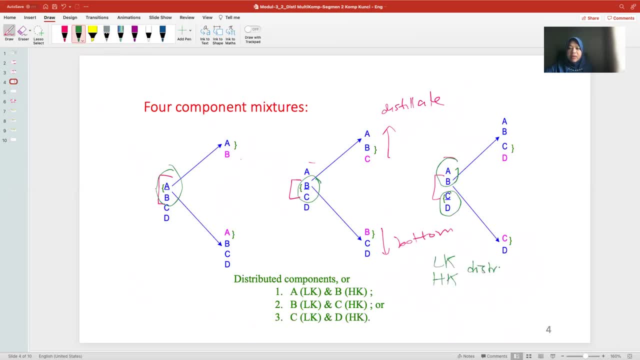 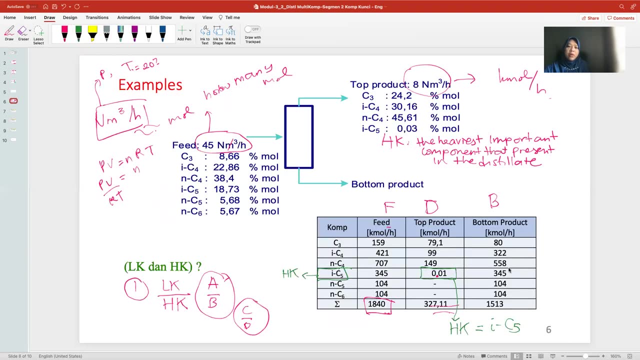 and l key is a: uh, distributed, yeah, so, again, so, uh, what is the heavy? what is the likey dhamma? can you guess which one is the light, kevin? what so? what is the likey e3? the one, the lk and hk, the, the, the most, uh, the uh. 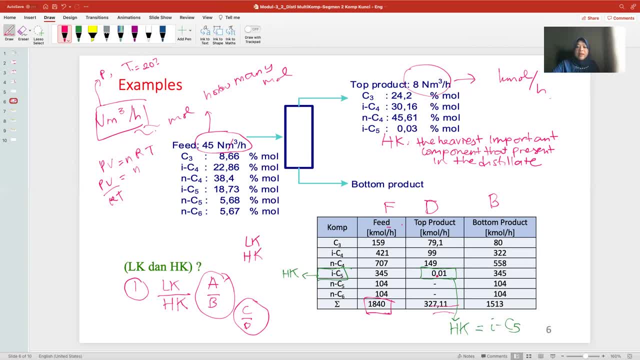 the neighboring uh that has, uh, yeah, very close, uh, volatility. fatia, which one is the light key? um, i'm not sure, miss. i still don't understand why i see five is the high key, right, okay, good, uh, why i uh i see five. why isopentane is the high key? because 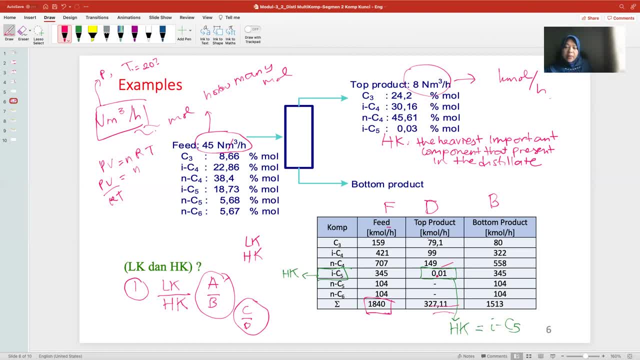 uh, so look at the top products. yeah, what are the components that present in the top product? c3 right, ic4 and c4 and i5 right, because after this there is no components. yeah, fatia, okay, it's true, yeah. and then, because we don't have any information, which one is the? 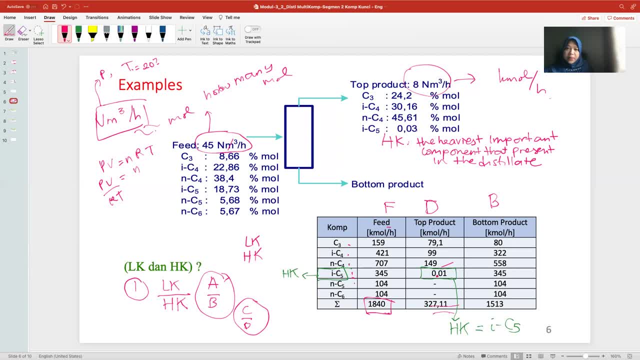 uh, all of them have the number. yeah, so all of them is important, okay, but we choose the heaviest one. so which one is the heaviest one that have a number? is this one ic5 or isopentane? uh, by heaviest you mean by its molecular weightness? yep, oh, okay, thank you. 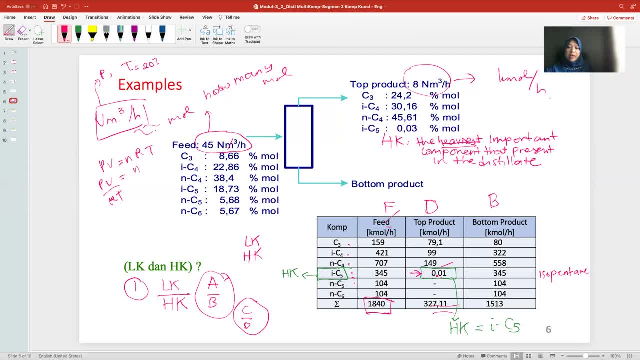 molecular weight. because, uh, why? why i did i? i didn't say nc six as the heavy key, fatia? uh, because the number is not available. yeah, because, because we don't. uh, because there should not be uh, nc6 in here. yeah, so the number that we 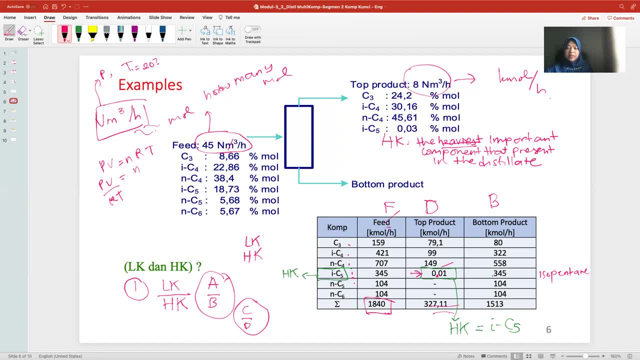 we're looking for is, uh, the one that available in the top product. okay with that. um, helena, what do you think about the uh light key? so what is the component for the light key? um, it's just to confirm. the light key is the lightest important component that is present in. 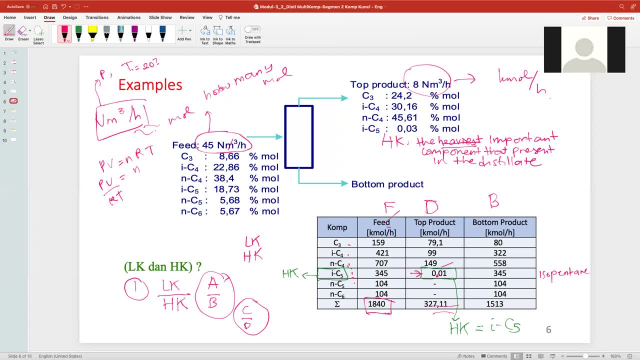 the bottom product, right? yep, would it be? i'm not sure, but maybe nc4. yeah, uh, the, uh, the, the, the, the lightest component that present in the bottom product, but it's also always paired with the light, the hey key, h key. yeah, it's always paired right. so, helena, you're right. so you're the nc4. now this: 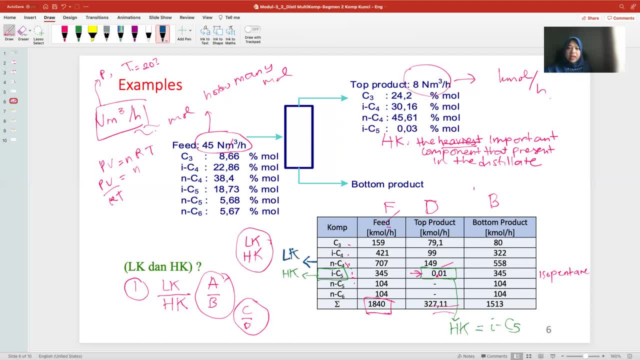 one is your light key. so see, uh light key and heavy key always paired with each other. yeah, so if you find the h key, then you can find the light key. so later this in uh, this will be distributed. uh, so, yeah, this is one is the distributed between the uh light key and the heavy. 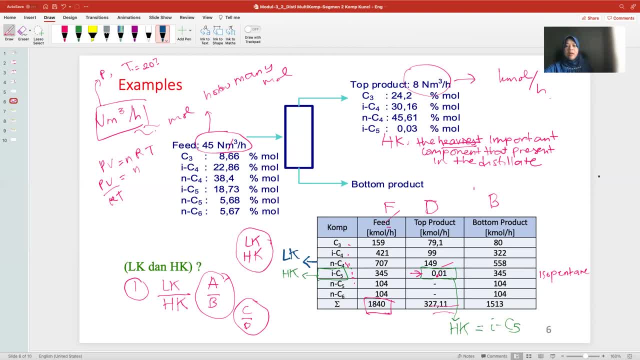 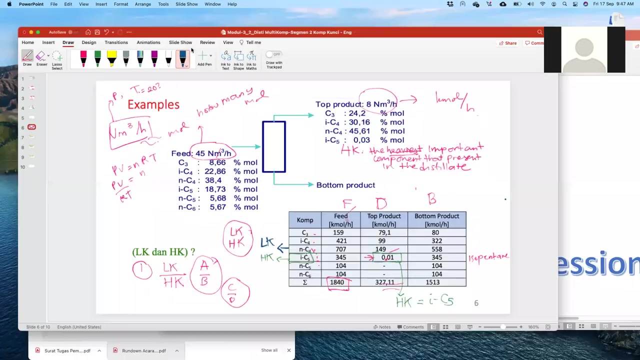 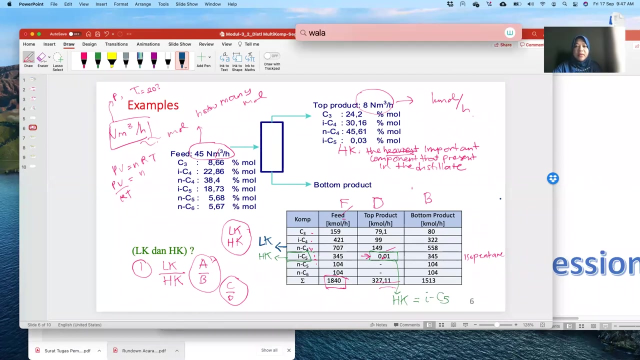 okay, okay, okay, okay. um, what do you mean by important component, like how do we know if it's important or not? uh, how to say, yeah, let's, let's open the book, let's open the book. have a look at this one. um, let's open the uh table. 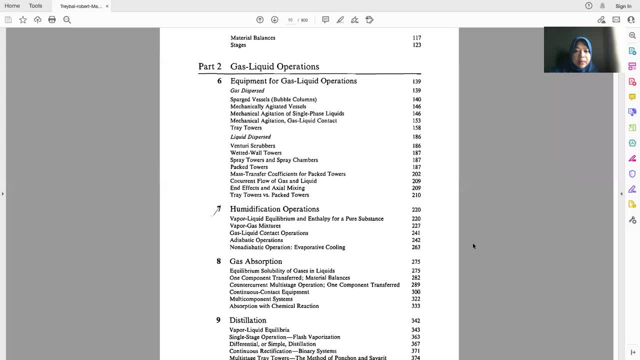 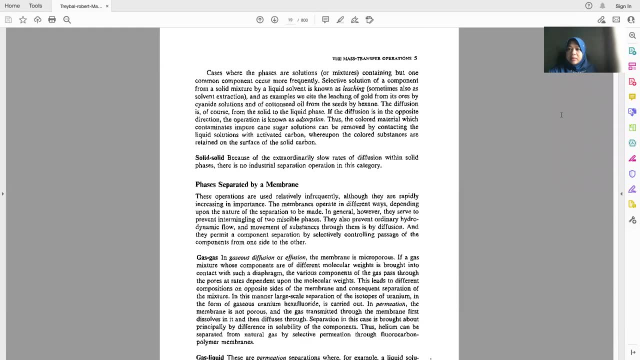 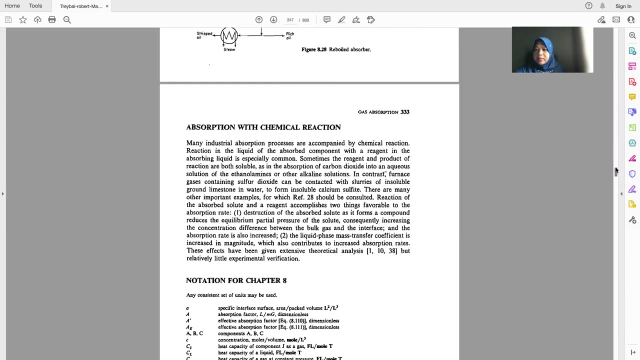 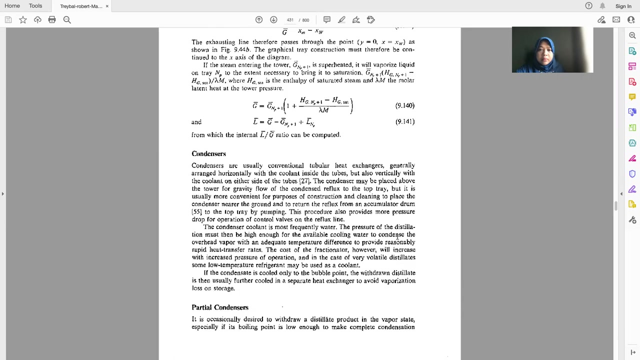 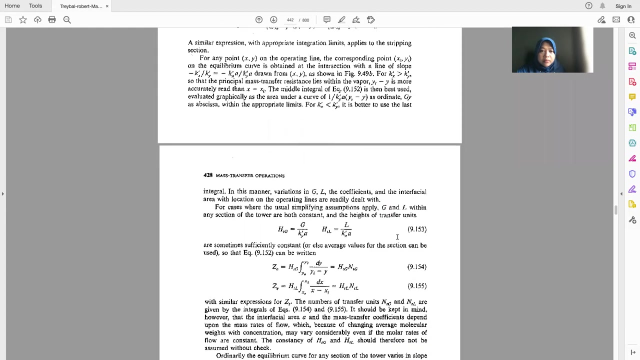 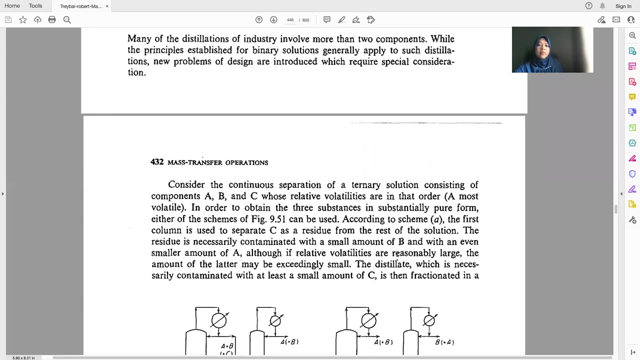 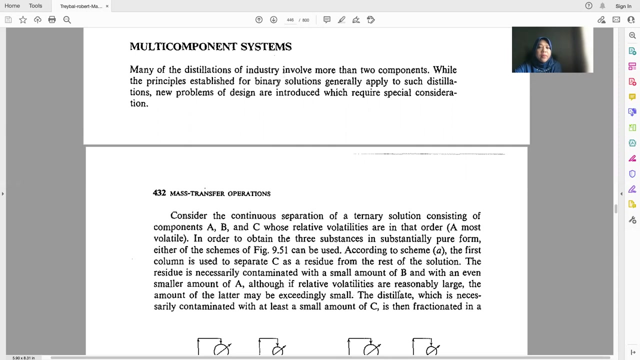 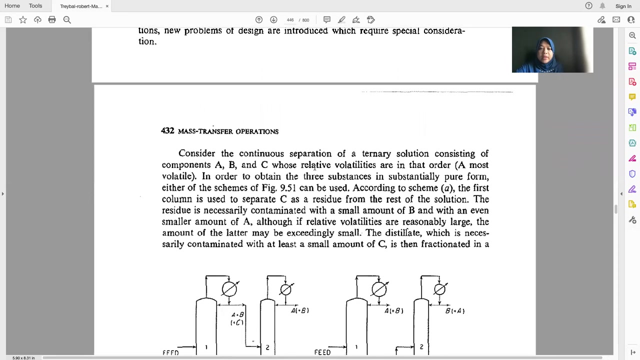 okay, let's have a look. the destination: multi component system: 431, 431, okay, so many distillation of industry involve more than two components. well, the principle of established for binary solution generally applies to such installation. the new problem of design are introduced, which requires special consideration. yeah, so uh, in ternary system it may be we separated. 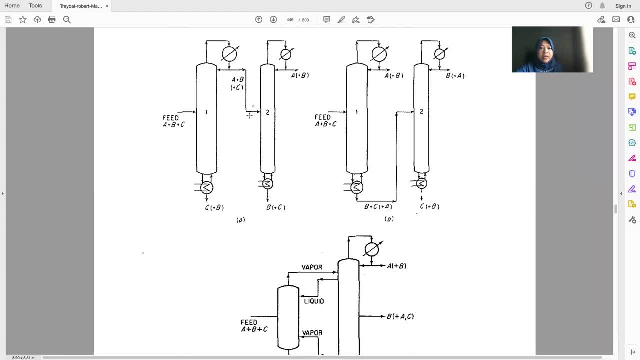 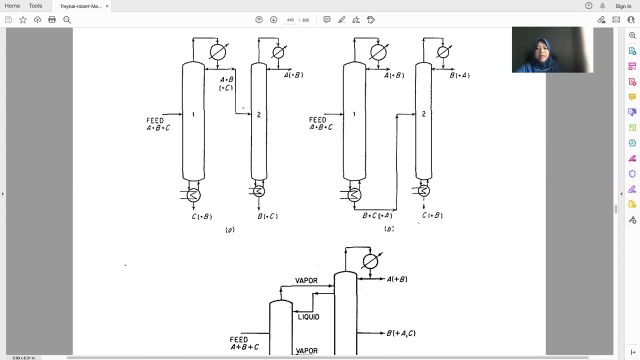 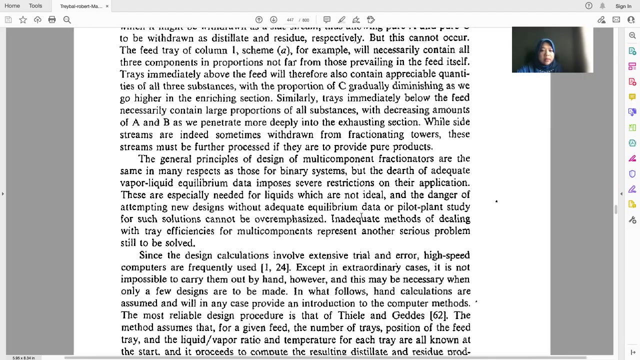 uh, a, b first, and then we separate it a and b, or maybe we have the top product, a, and then we have b and c, so this one, in this case, the distributed is between a and b. yeah, for example, a, b and c, for example here, um, let me try it, check, check, check, check. 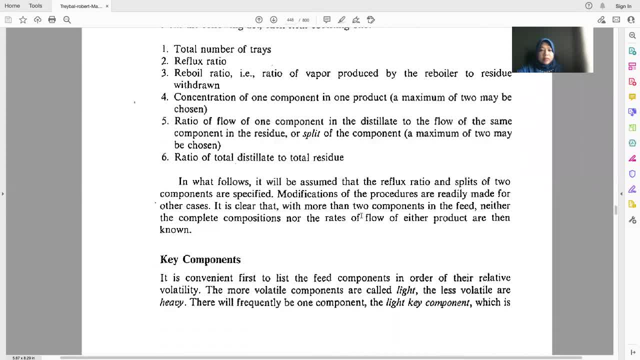 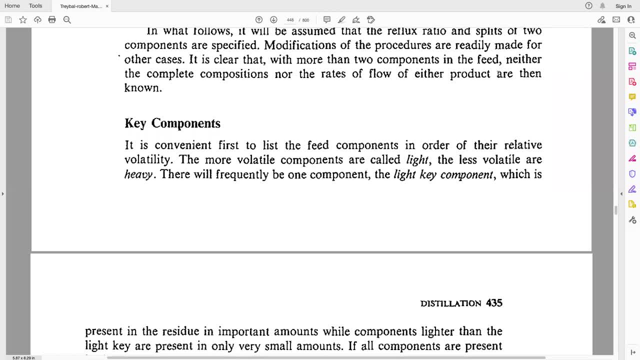 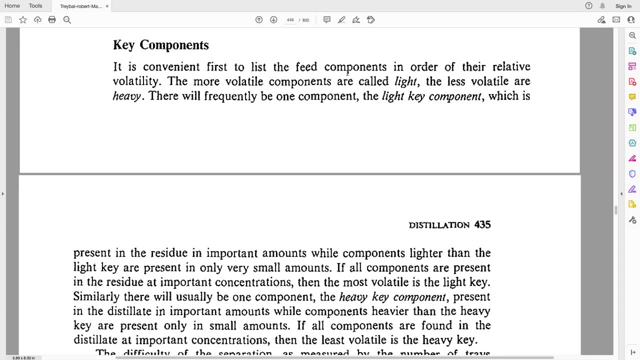 okay, let's, let's, let's, uh read this one, yeah, together. so we have some idea. so it is convenient to list the, the, the feed components, in order to for their relative volatility: the more volatile component is the light and the less volatile component is heavy. okay, there are, uh will be. 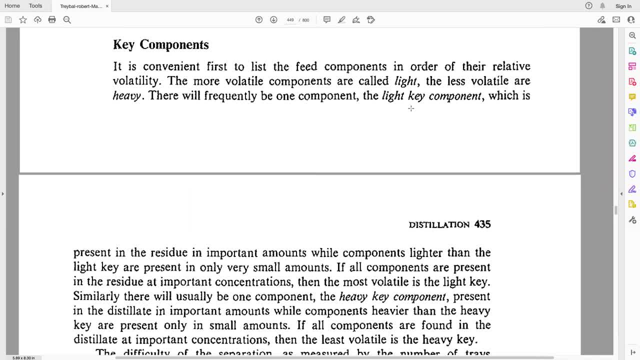 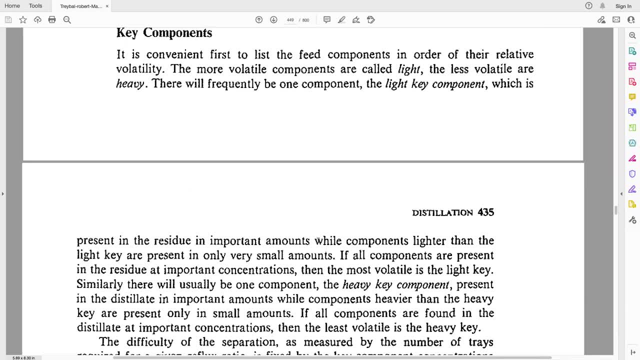 a frequently one component, which is called the light component. and the light component is the key component which is present in the residue or in a bottom product in important amounts, while the components lighter than the light key are present in the only small amount. if all components are. 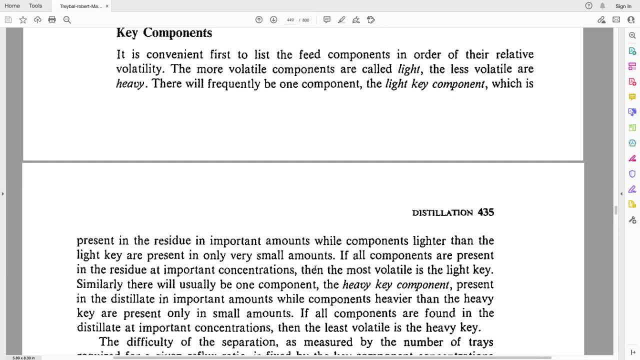 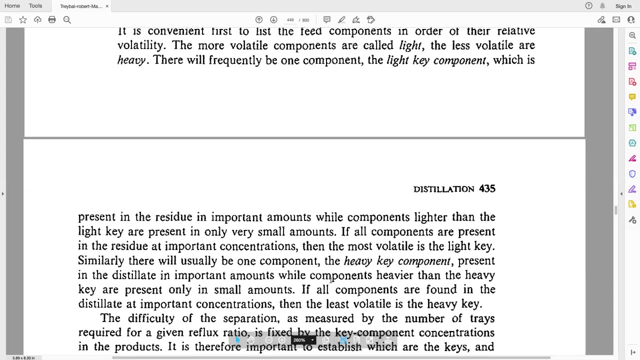 present in the residue at important concentration, then the most volatile is the light key. so see, if all components are present in the residue or important, important concentration, then the most volatile is the light key. similarly, there there will be one component, heavy key component- present in the distillate in important amount. well, components heavier than the. 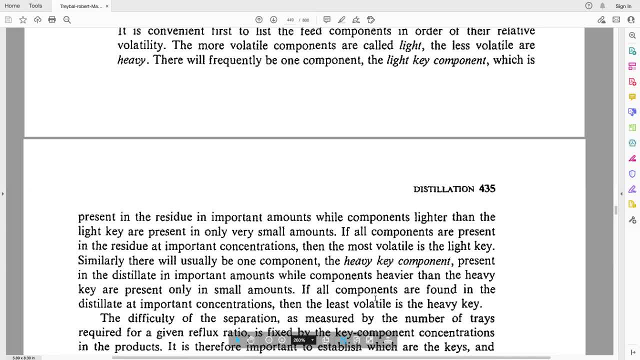 heavy key are present in only small amounts. if all components- like maybe this is, or in this case, yeah, if all components are found in the distillate at important concentration, then the least volatile is the heavy key. so, um, we have to say that all components are present in the трупол слов. 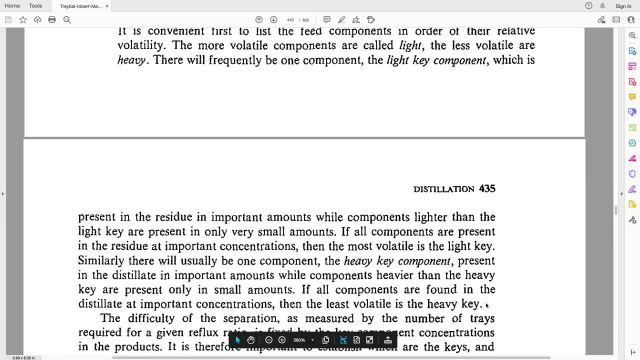 So to answer Fathia's question, so which one is important, which one is very important or not? sometimes it should be happened in the distillate, it should be happened in that problem, but if not, for example in our example here. 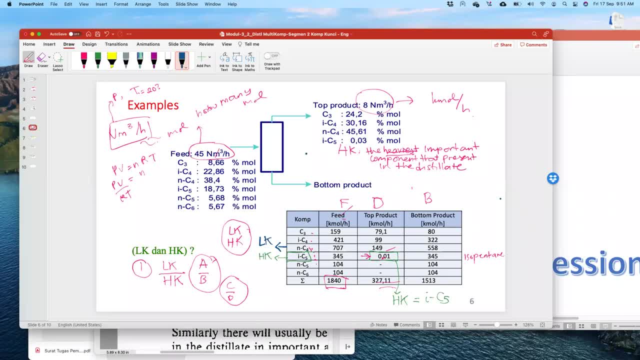 okay, in our example here we have those of them in the top product- are important. yeah, the top product is important, yeah, because there's a number here: 0.79.1,, 99,, 149, and then 0.01, so those are important or defined, yeah. 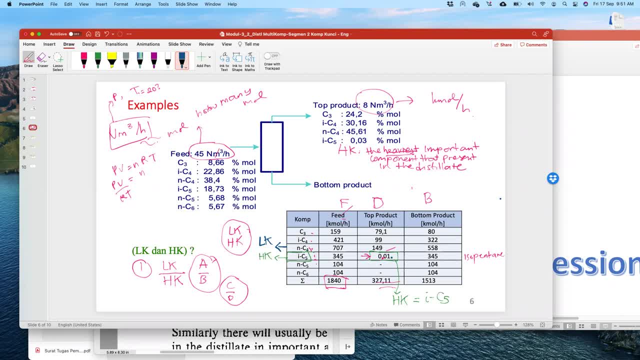 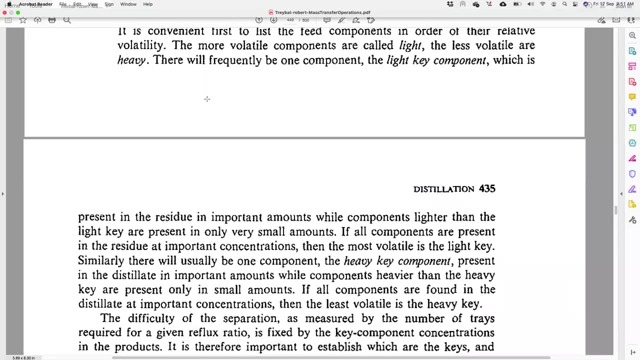 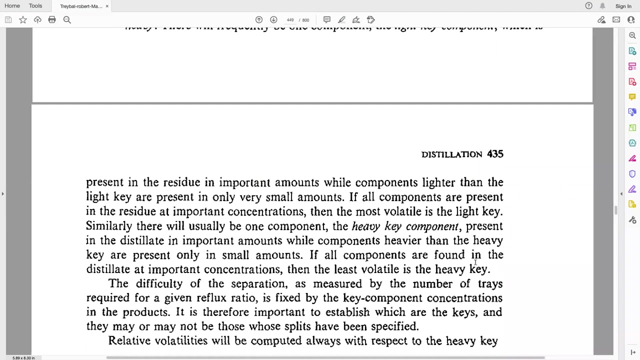 the other way to say it: maybe are defined. okay. so then, to choose, the heavy key is the one that's the heaviest one. so go back here. maybe should I okay. yeah, so if all components are found in the distillate are important concentration, like in our case. all of them are defined, the more percentage yeah. 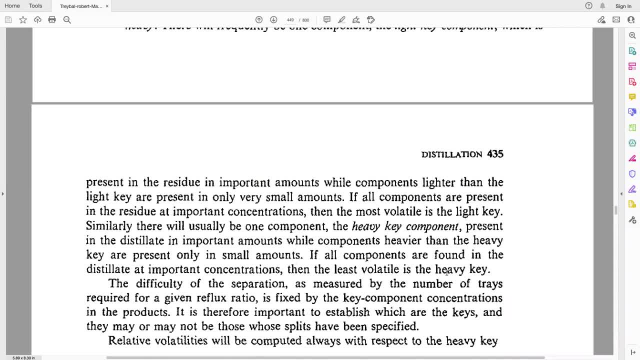 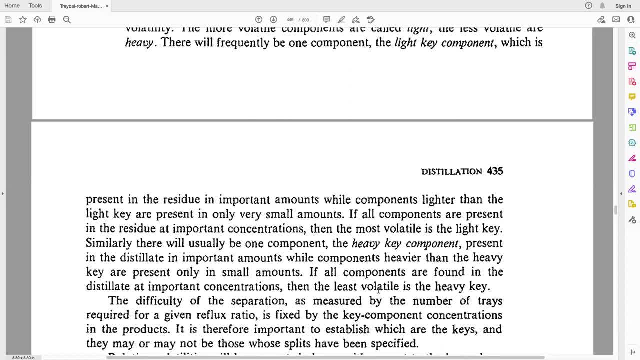 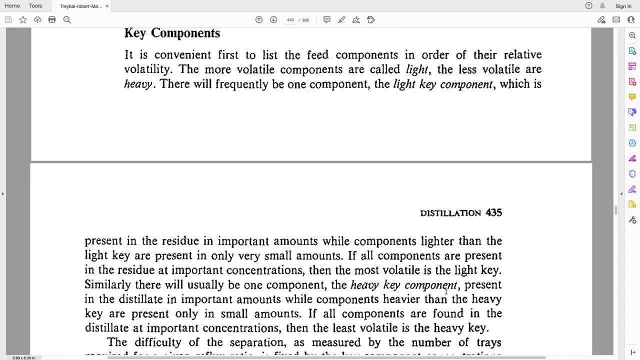 then the least volatile is the heavy key. the least volatile, which is the heaviest one? yeah, the bottom one. okay, I'll give you two or three minutes to read this one and let me know if you have any other questions. 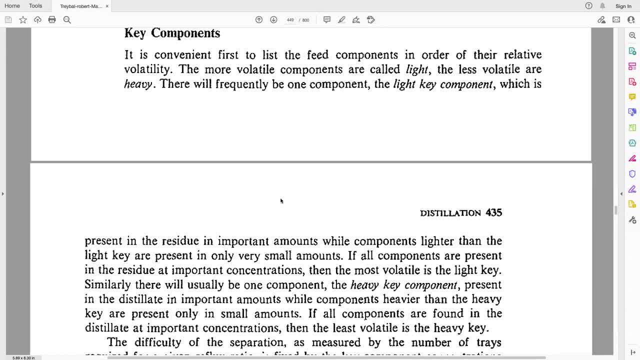 Okay, what do you think looking at the textbook, is it answering your question or still confused? I understand this Right. how about the others? Yeah, why is it that the heavy key and the light key needs to be neighboring to each other? 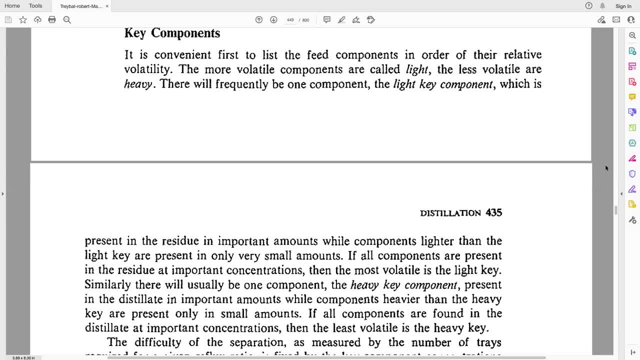 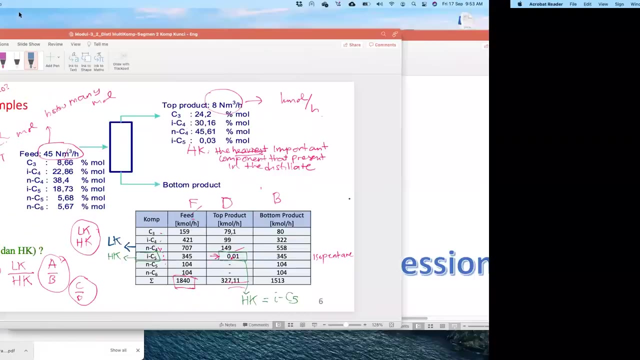 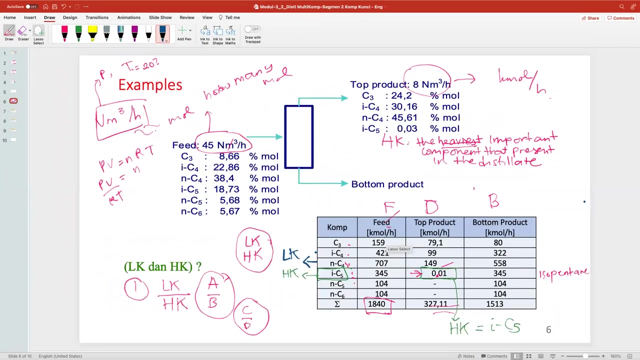 Right, because, yeah, that's my question as well- why we can't have they separated. Because light key and the heavy key is always distributed. It's always distributed one in the distillate and one in the bottom. but which one? the heavy key and the heavy key and the distillate? sorry, the which one to? that's why to choose the components and the 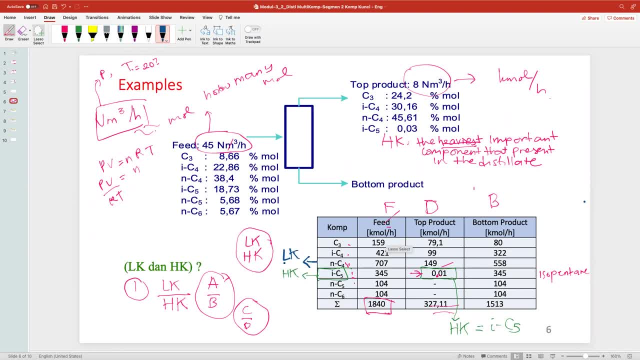 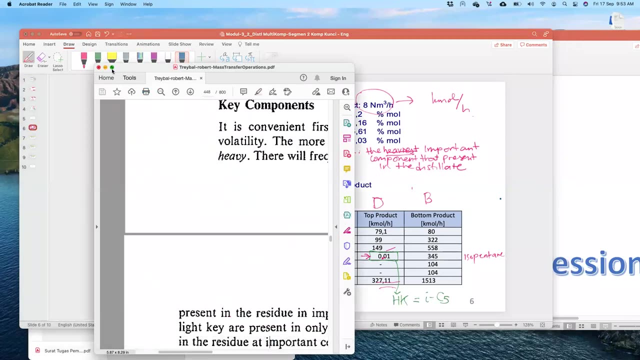 to choose which one is the, the L key and then the heavy key is actually based on our problem definition. yeah, for example, in this case, maybe, for I should put this one, maybe I'm going to put this one, and then 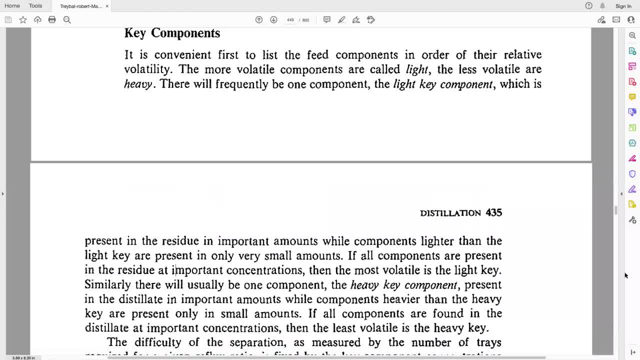 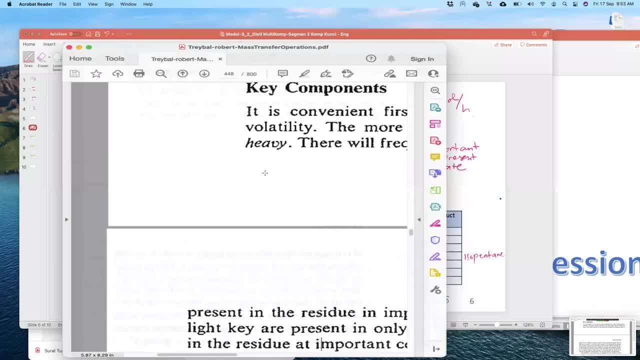 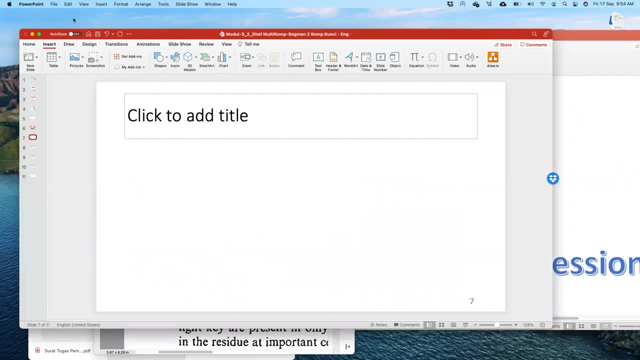 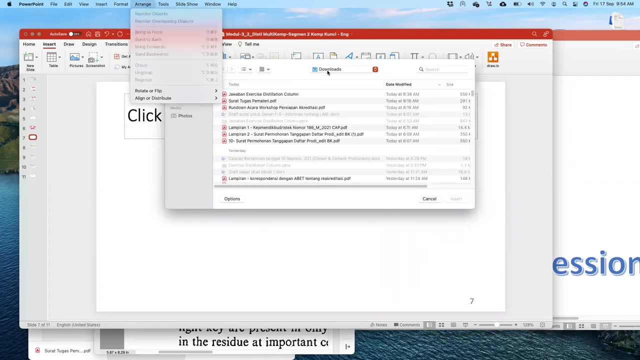 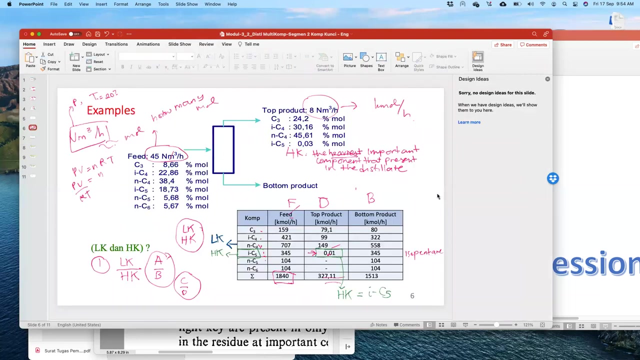 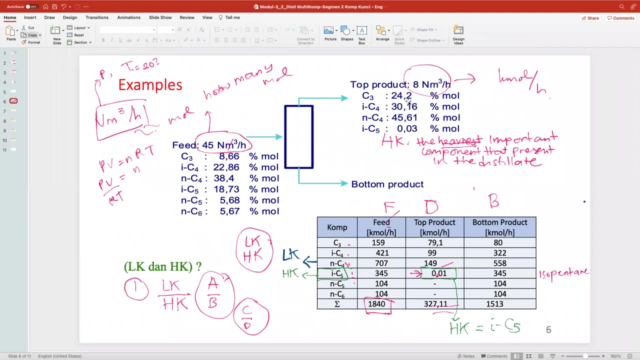 before. you don't, okay, so I can maybe put it in the okay here. so you? so we don't let me put this one first, so at least you can have a look. Okay, yeah, right, Okay, so a very good question, Kevin. so actually, this one- this will, the way we choose L key and H key- will determine the top product and the bottom product that we get. 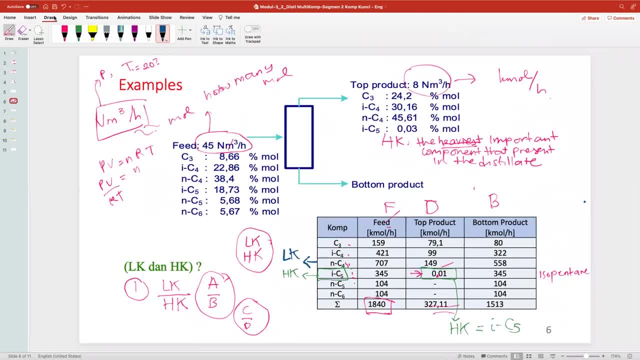 If we calculate, for example. if we calculate, for example, I want the L key is IC4.. Yeah, yeah, and also the heavy key, I want that as NC4,, for example. If I require that one for the separation, the distillate would only contain C3,, IC4, and NC4. 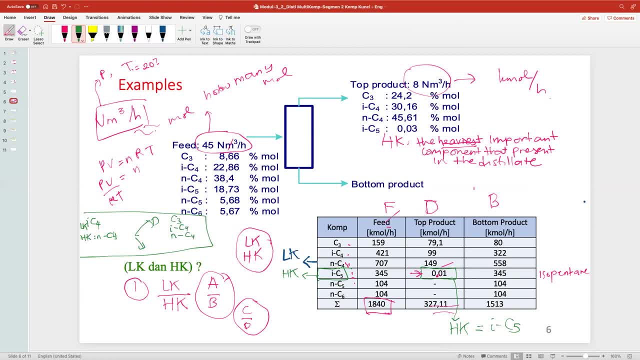 So there's no IC5 here, okay, Okay, well, in the bottom, The bottom would be maybe from the remaining. okay, so it's see the choose the option to get which one is the heavy key and the light key is actually going to be impacted on the result of the product. 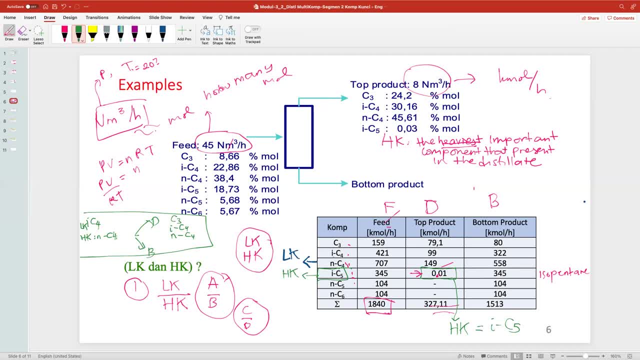 If you choose the heavy key and for example, NC4, then your top product only up to this one. So then you don't, You don't specify the last one and sometimes, usually the amount of the heavy key is quite small. yeah, the composition, the important amount, doesn't mean that it should have to be very big one, so usually it's present in a small amount. 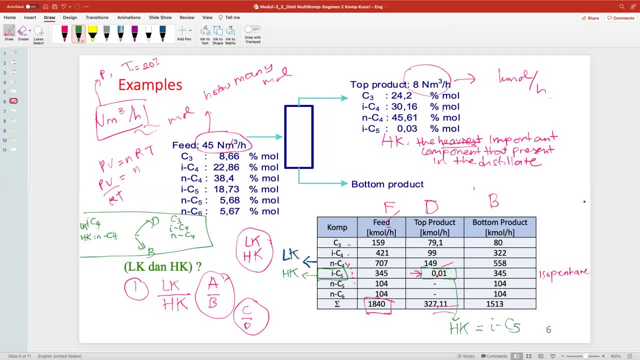 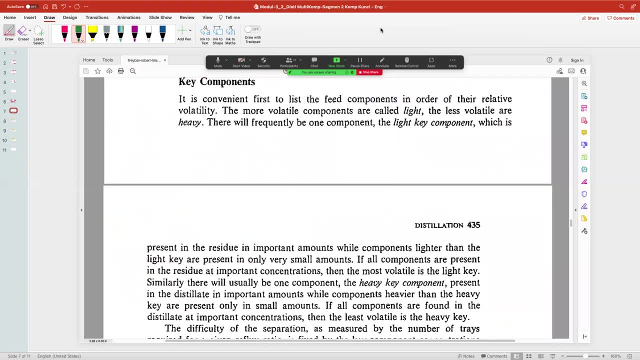 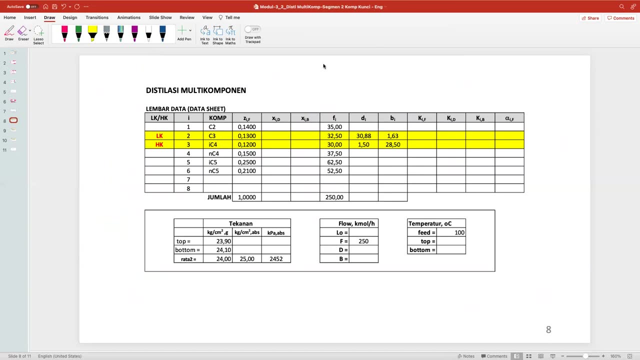 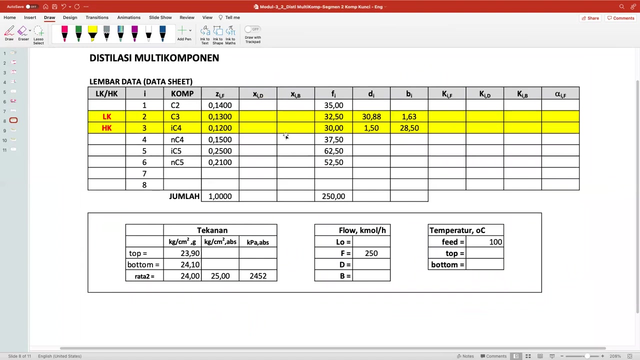 How about that, Kevin? Yeah, I kind of understand this, Bu. Yeah, let's have a look at the next slide. yeah, About a practice. Right, Let's have a look about this one. okay, This one is actually ideally, you have to open Excel. yeah, you have to open Excel, so I think let's check this one. 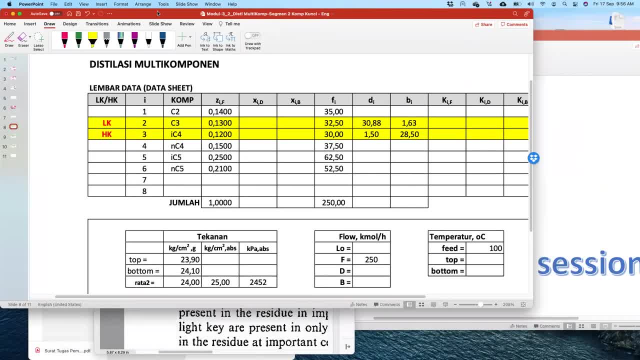 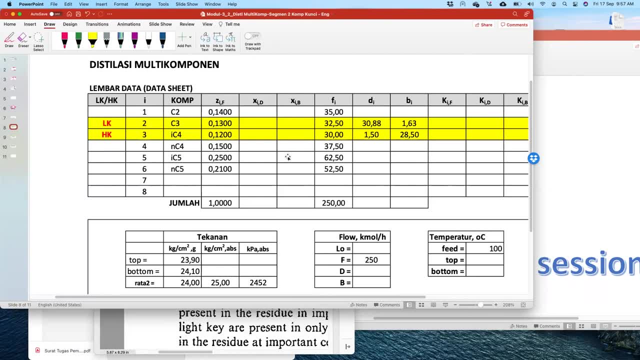 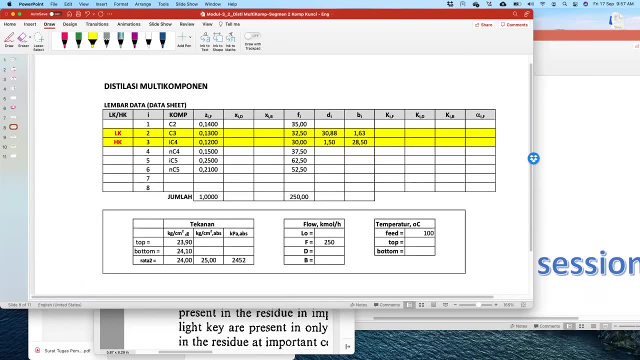 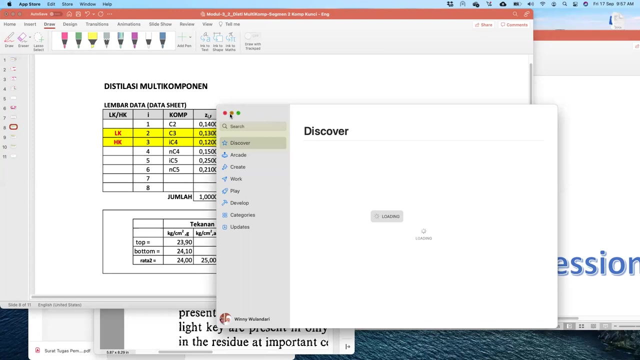 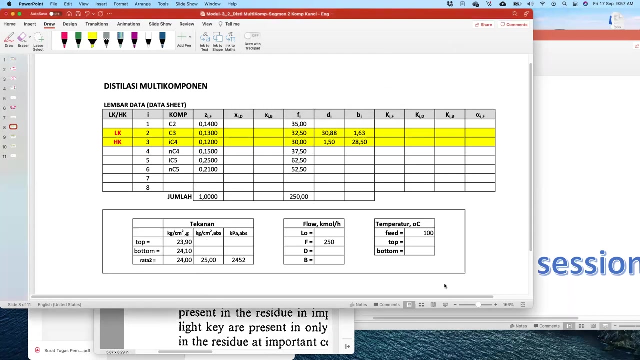 I'm gonna open Excel, Okay Now. So let's have maybe 10 minutes break to copy this one to your Excel. So you have your own Excel. So this one should be in the Excel. So we're going to continue. That's my Excel. 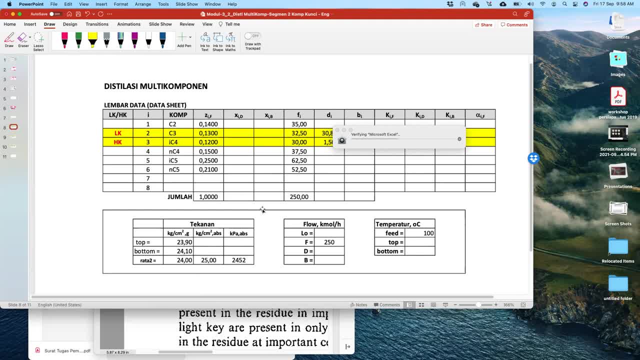 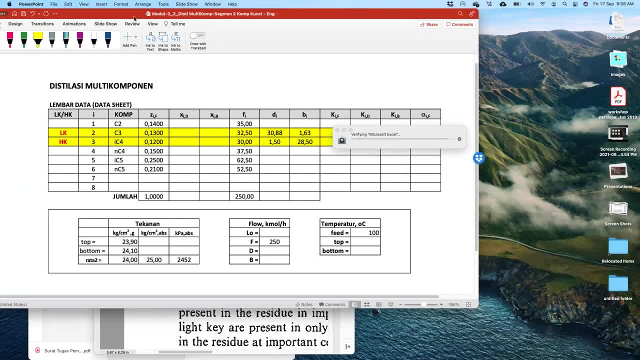 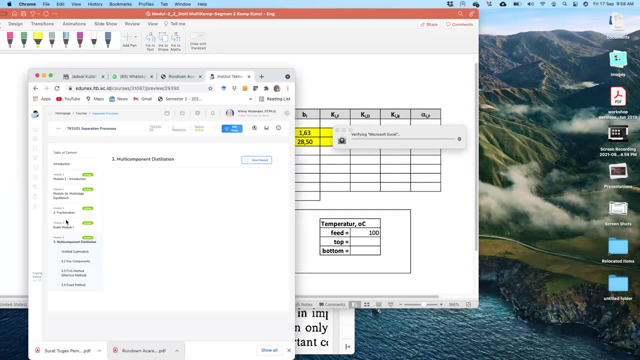 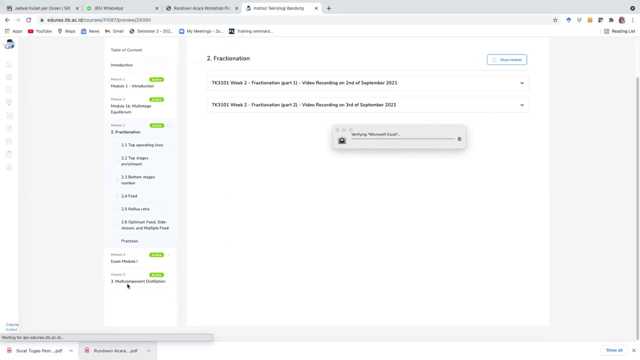 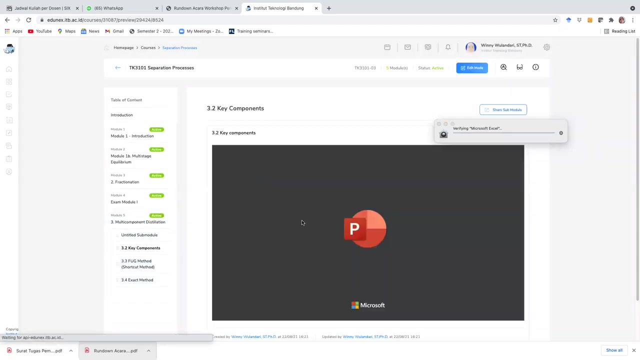 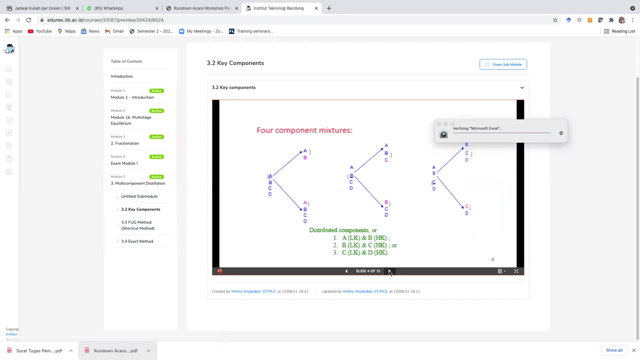 Okay, Meanwhile you can check the module on Edunex. Yeah Well, I'll try to copy them. So it is in the multi-component distillation, Yeah, Meanwhile, Okay, Multi-component distillation. Okay, And then look at the. I think the key component should be here. Yeah, The key components there. And and okay, Yeah, This one there And then this one. I don't know this one or the next one. I think there should be some assignments about this. 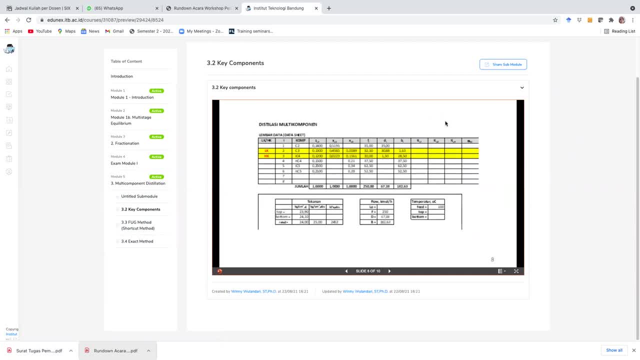 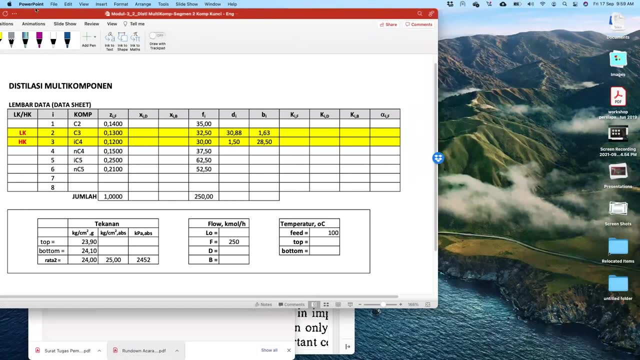 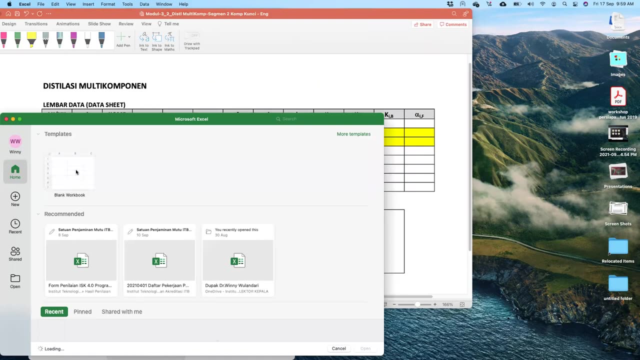 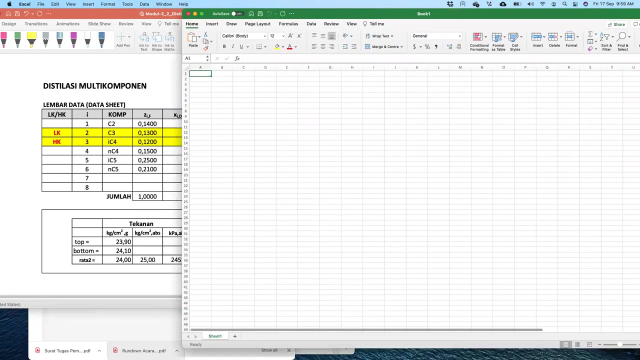 So it would be good idea if you can copy this one on the You you make again the table on the Excel, because our Excel is a very powerful, very powerful tool. Yeah, For us. as a chemical engineer, I always using Excel for many, many steps. Yeah, Algorithms. 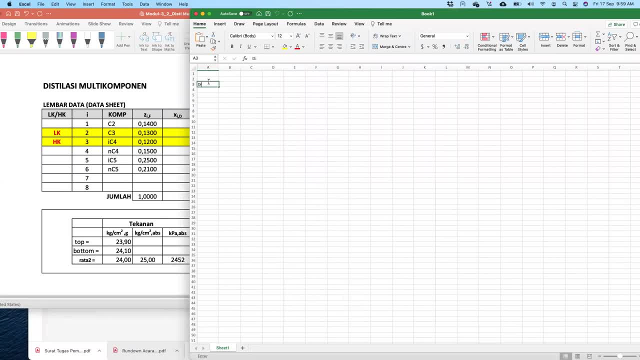 So that's right. This is distillation component. This is- we have to change Which one is L, T and a heavy key, And this is the component I. this is the component that I F. and then let me have a very quick one. 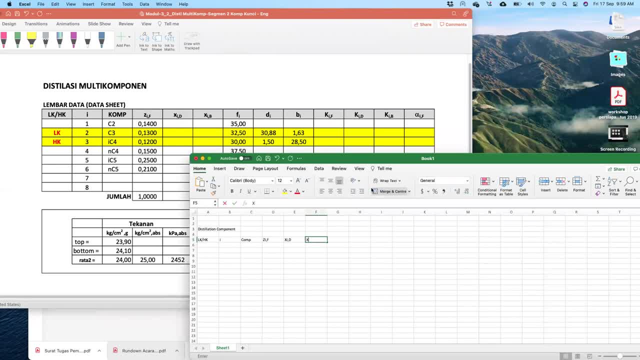 X I D X I B, F I D I X I D X I B, F I D I X I D, I E Di D I K I F, K I T, K I B. alpha int F. 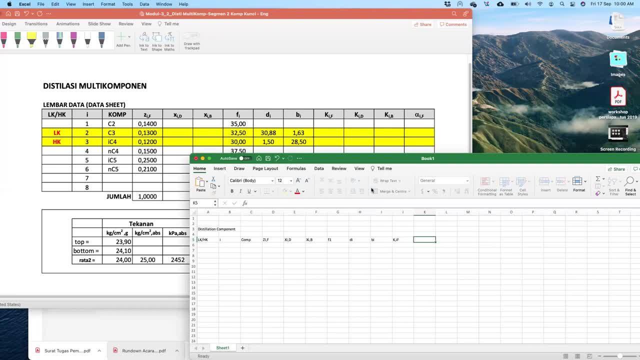 Di, Di, D, I, K, I, F, K, I T, K, I B And alpha int F. One, two, three, four, five, six, seven, eight, nine. Okay, one, two, three, four, five, six, seven, eight, nine. 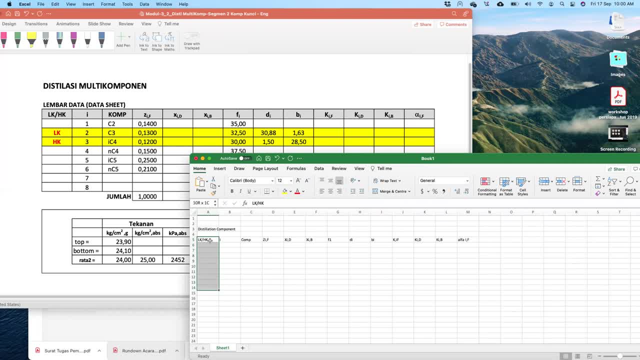 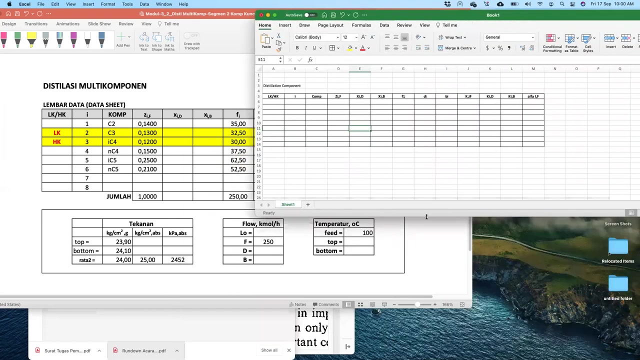 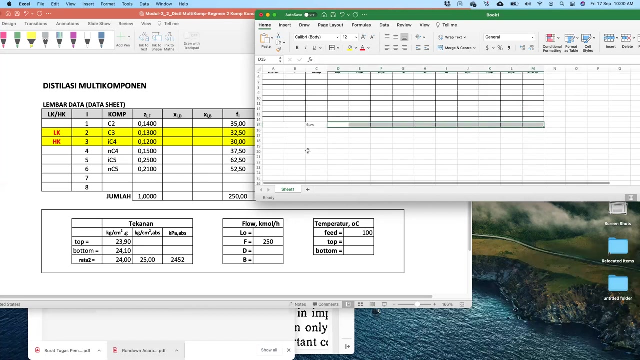 Okay, make it bigger this one, put it in the center and make it bold, okay, right. And then we also need to find the component. so sum and this one. we have pressure at the top, the bottom. you can try to do it by yourself too. yeah, and average, okay. 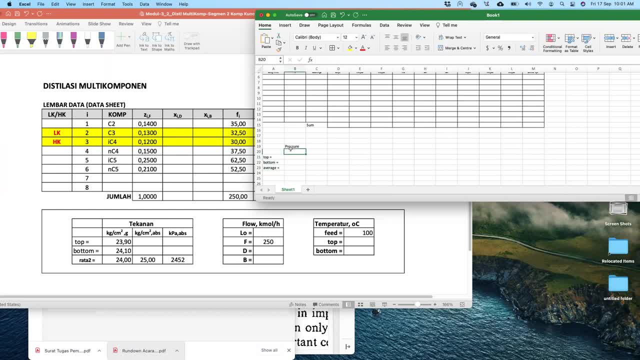 Because this is going to be our spreadsheet. Okay, look around. Okay, this is the flow. the flow is in km per hour and also we have temperature, which is tpc: feed, pop, pop. ok, you will have a lot of spreadsheet during your student life. 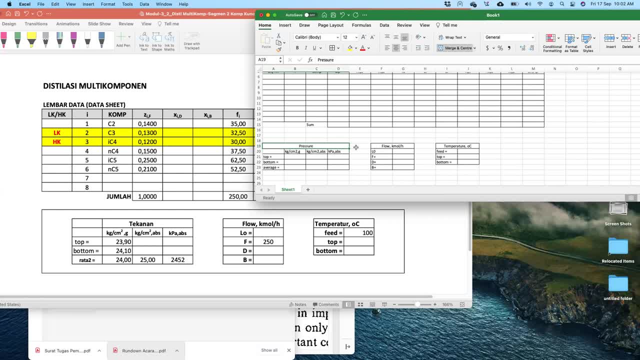 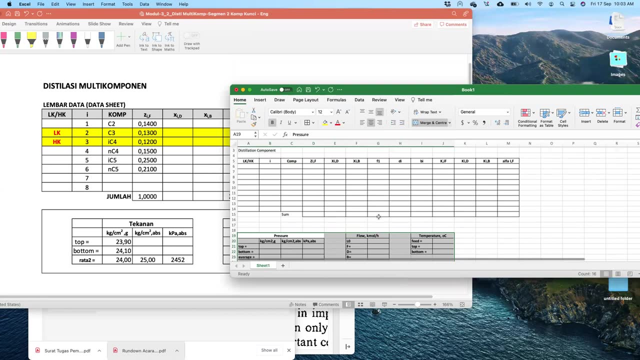 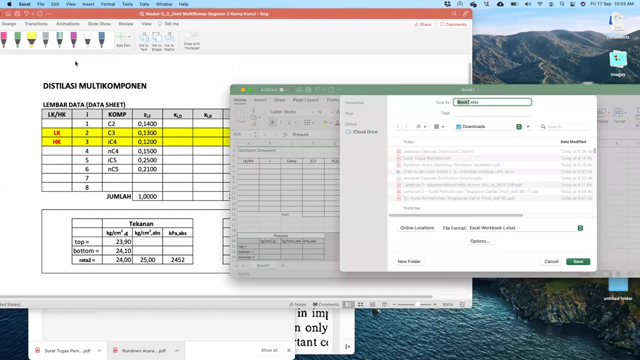 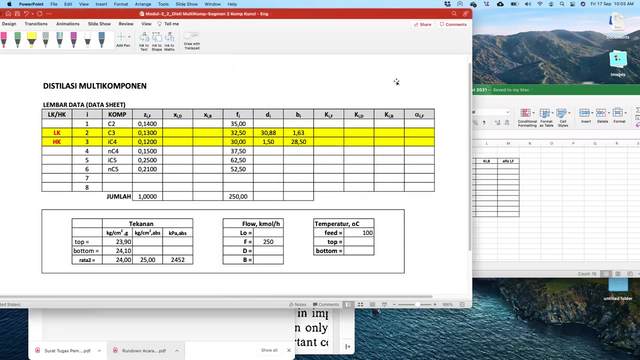 make it bigger there. to read this one here, you have to do it one by one. for example, save as xh1. ok, ok, let's have a look about this one, and then I'm gonna do it in the bottom product. so this is called: 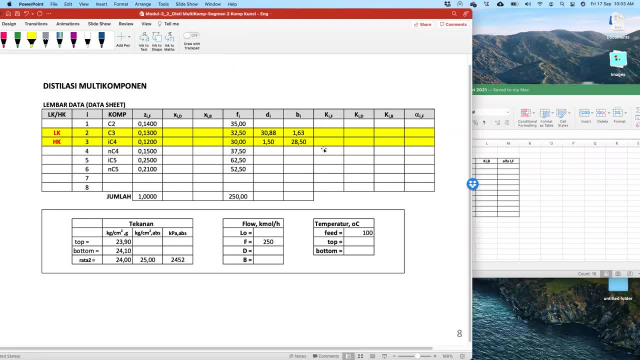 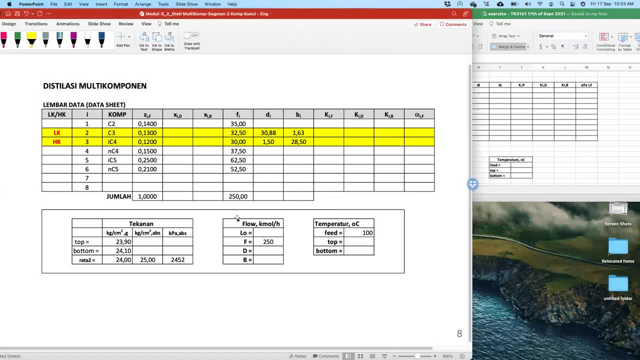 data sheet. we choose the. we put all of the information on the data sheet one. so, uh, so look at the uh, the data sheet first. uh, i think that this one. there should be some uh or the problem uh section, so but anyway, from here we see that uh, there is um. 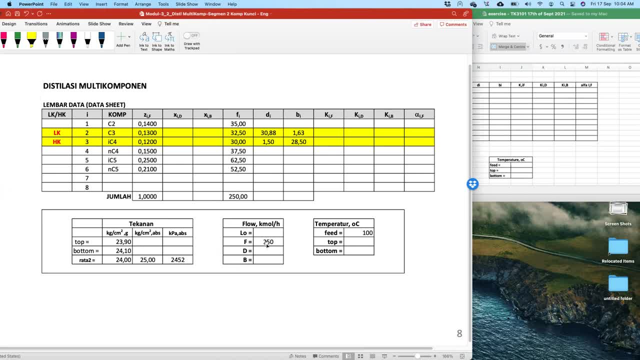 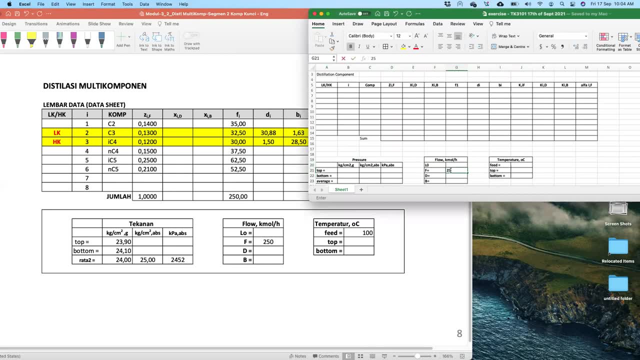 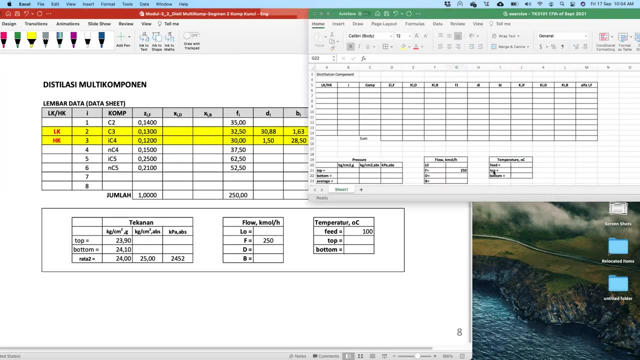 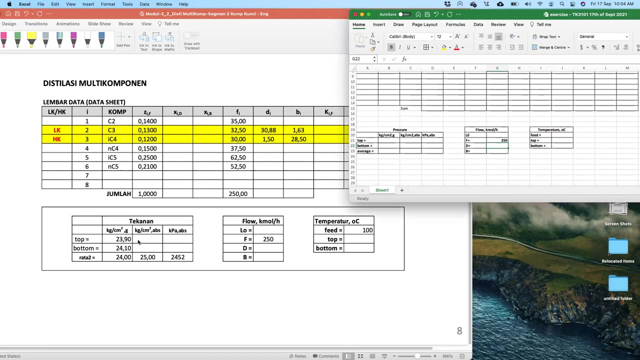 feed. yeah, the feed is about uh 250 kilo mole per hour. yeah, feed, so let's put it here. and then um, also the the the top product is uh, so the it's defined as uh 23.9 uh kilograms per uh square centimeter gauge: yeah, g is gauge. 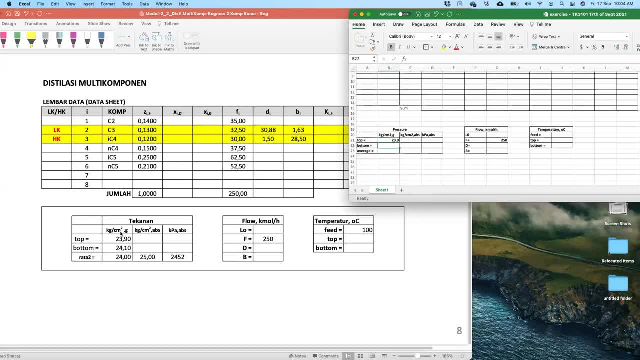 okay, do you know? uh, kilogram per centimeter, uh, square gauge is equal to what is the, the conversion unit um? so let's set up the conversion unit um and then i can make it. uh, check it, yeah, in the, uh in the conversion sheet, uh, in the conversion. 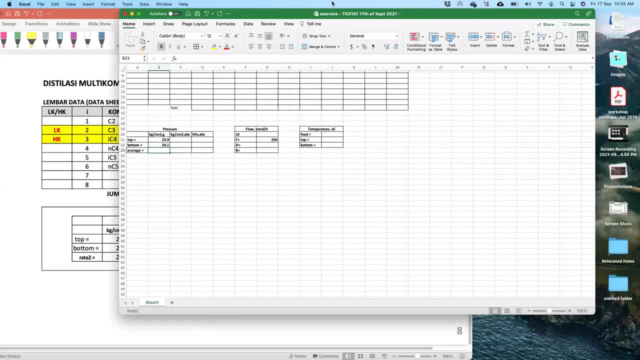 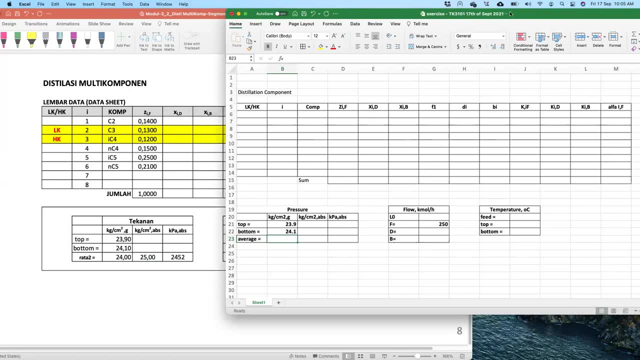 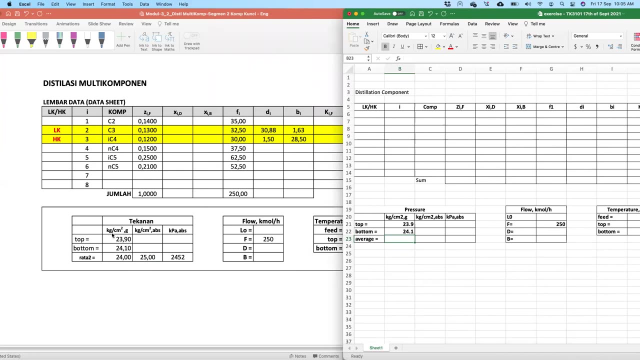 unit, uh, what is the? maybe, maybe let's make it big, okay, yeah, kilogram per centimeter square gauge is equal to about, uh, about bar. yeah, maybe about about bar or about atm. so this is about 23.9 bar, and then, uh, usually the top is less compared to the bottom. 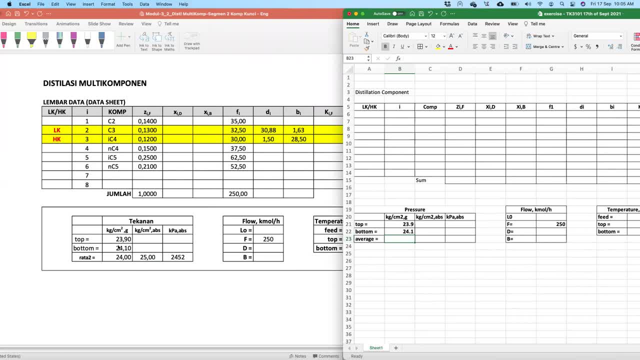 so, because there's a, there would be some a pressure drop, yeah, so then, uh, you want to have. so here we have the average. let's say the average, uh, for the for the pressure for our calculation is around 24. okay, this is the if. if the problem is defined as the gauge, the pressure in gauge. 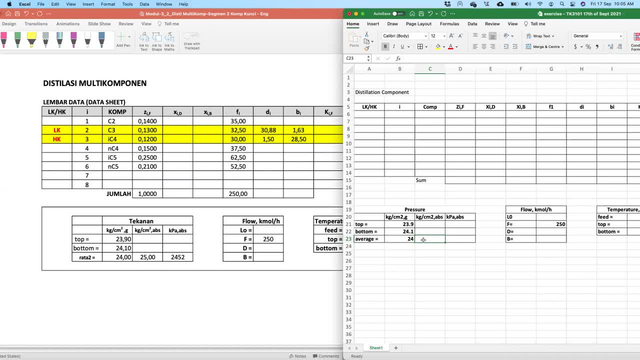 then, to check the absolute, we have to add one more, one bar more, yeah, yeah. so, uh, 180 m is about one kilogram, uh, per square square. uh, yeah, per square centimeters. yeah, so then we add one for this, one plus one, okay, so that's about 25, okay, and after that, uh, we also need to change. 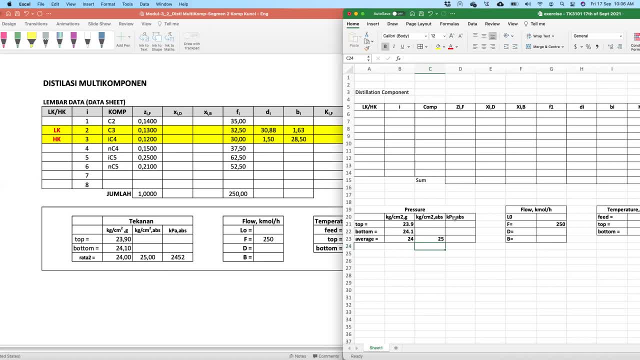 it into kilopascal absolute. yeah, check uh how to the conversion between kilogram uh, same square centimeters, to the kpa uh, and then maybe this one here is up to- let's just write it down right- the conversion about 2452. okay, why you need pressure? 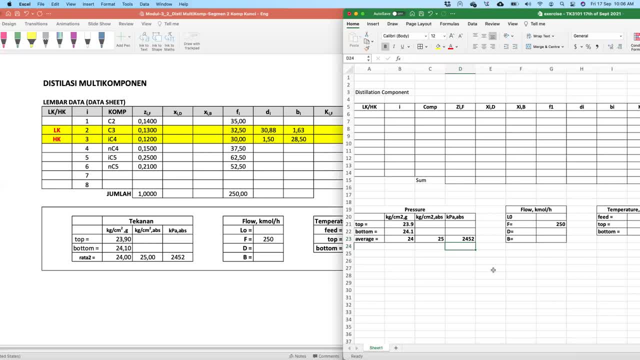 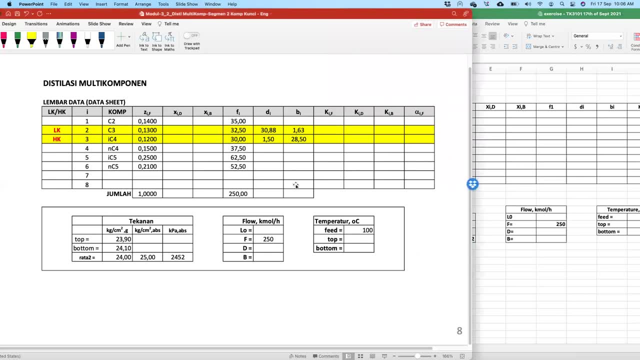 why we need pressure? because we need to find the k value. yeah, we need to later on. we need to find the k value, so we need the information of pressure and also the temperature, right, okay, the next uh question is: also: we know the flow. here is written as: 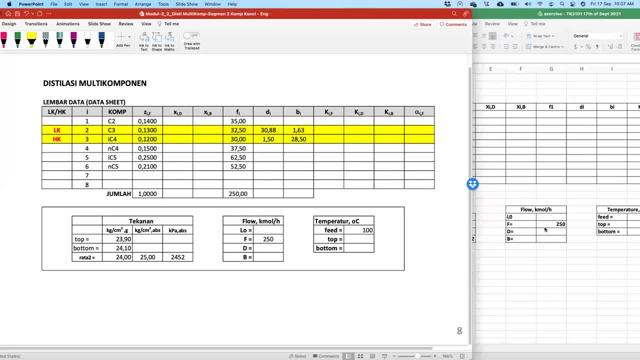 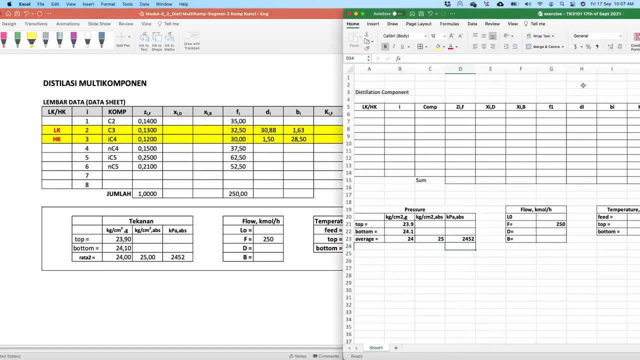 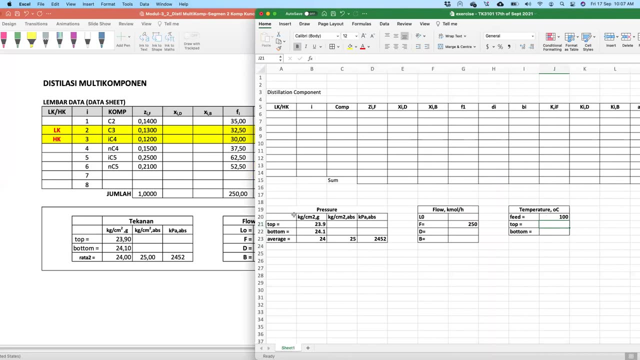 250. so i'm gonna use uh 250 kilomole per hour. and also, here we have the temperature of the feed, which is uh 100 degrees celsius, so let's put it into uh 100, okay, okay, um, in the problem. uh, we know. 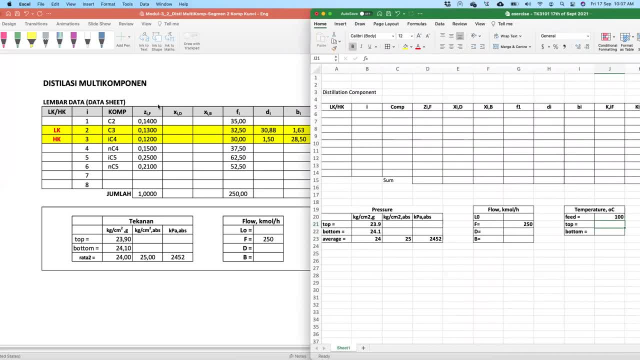 the feed is actually comprised of this component, so let's write it just: the component one, two, three, four, five, six, seven, eight, oops, seven eight, and the components are uh, c2, c3, ic4, c2, c3, ic4, mc4. so there are six components, yeah, and then uh. here, uh, we have also the composition of the. 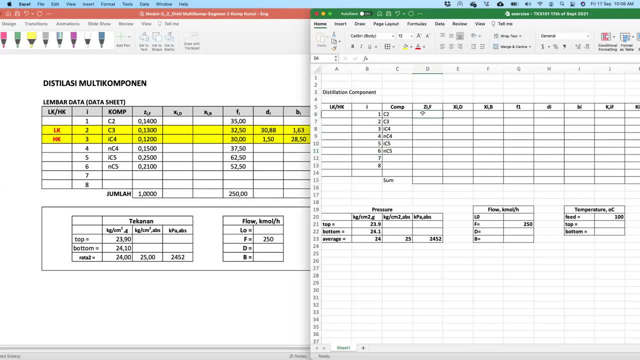 feed. yeah, so that i f we have the composition, so then we can put it there also. let's take these two Birds so that we can make it bigger, and then i also want to make it small. let's, uh, just put this one into the middle and also also that we can make it. uhThat woman is. we need this next toų. 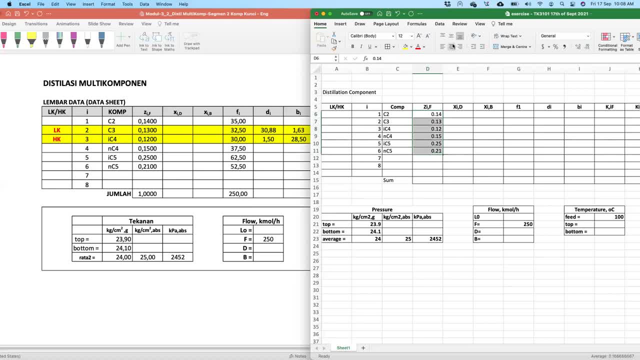 going to make this really large finale like this. so if we call it align, it looks like this. there you go. yeah, so we have four complex levels like this and now we're going to did it, so we're gonna leave it. so let's okay, let's leave this text box. 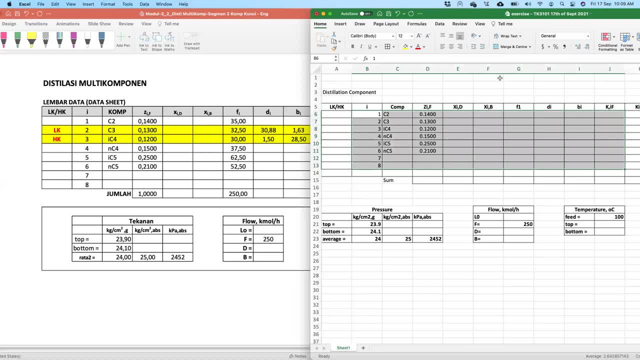 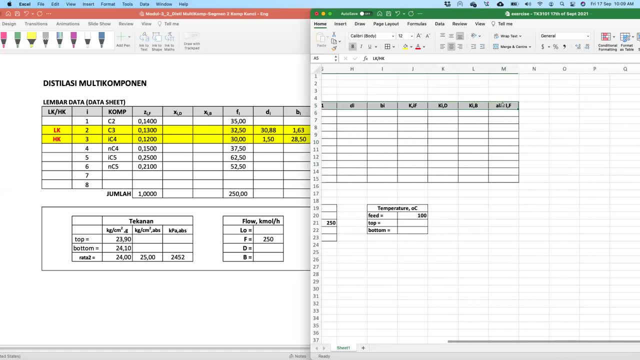 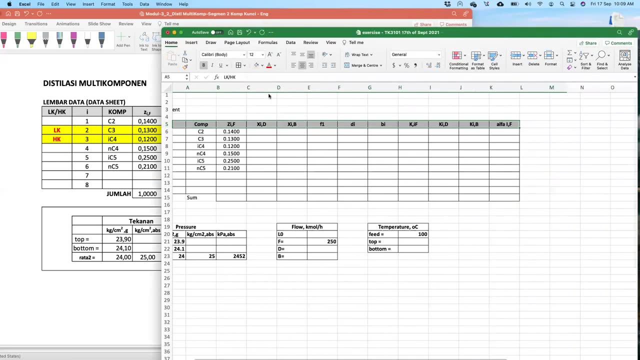 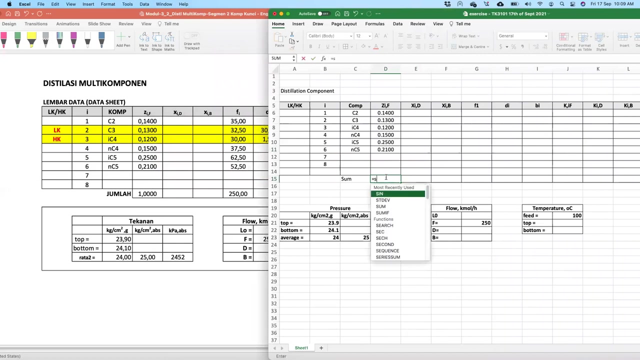 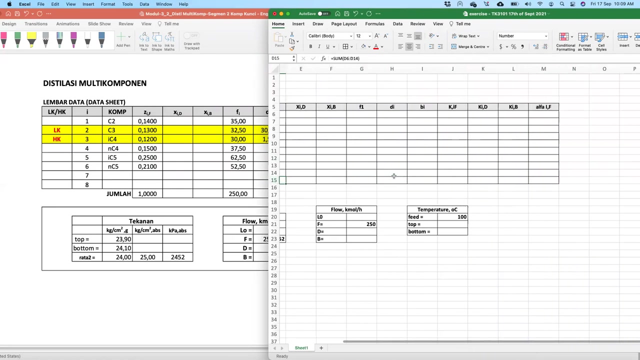 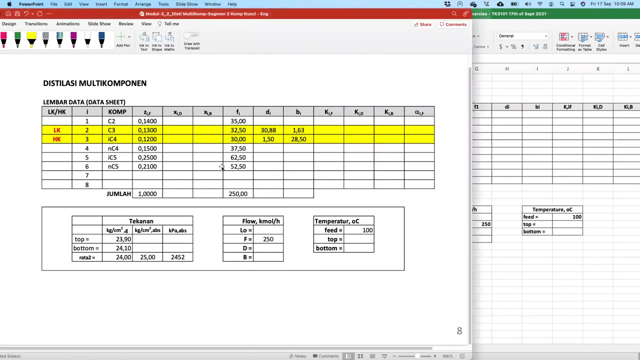 let's just é. let's say, I want to make aôle, okay, OK, in the center, right. so let's just check it from it, from it up, is it? this should be up to one. okay, so this one is one. okay, now let's say so here: the FI, yeah, the FI. 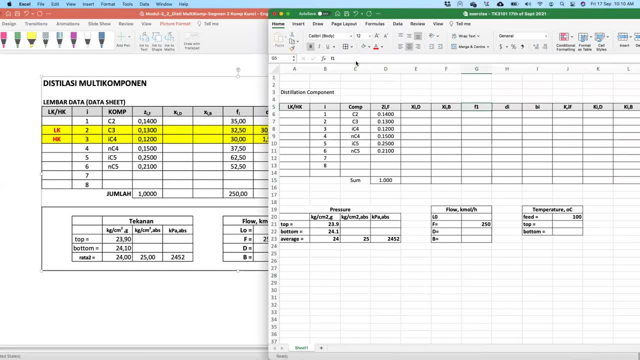 is the feet of the component, yeah, feet of the component. feet of each component, which is should be the. the total should be all of the F, yet 250. so how to get the feet of each component? we have to multiply the component with the feet. yeah, and then use this one. 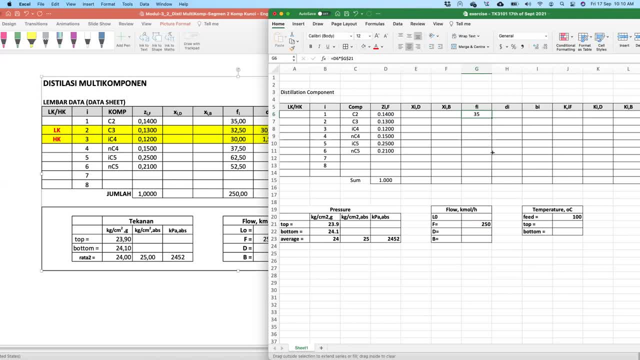 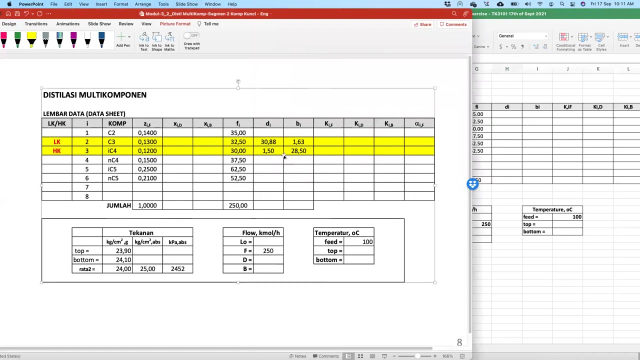 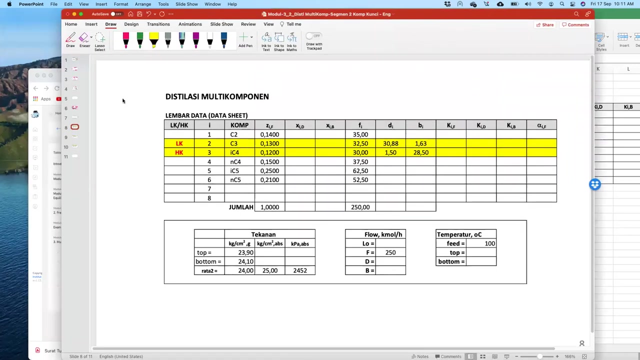 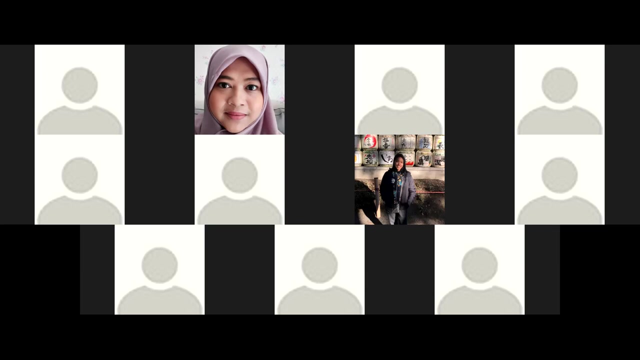 don't forget to sum it up: okay, yeah, okay, like that, and then maybe put this one to number. okay, that's the feet. I want this one to get this one. I have to check the. an example. let me, let me stop share. and then I have looked the the problem. yeah, it's. 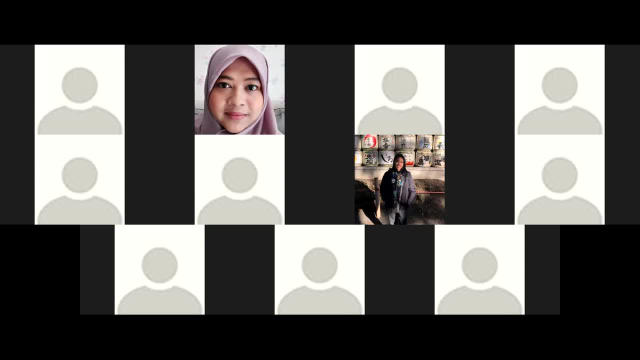 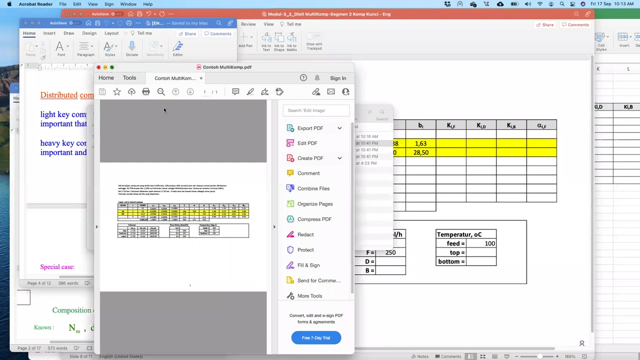 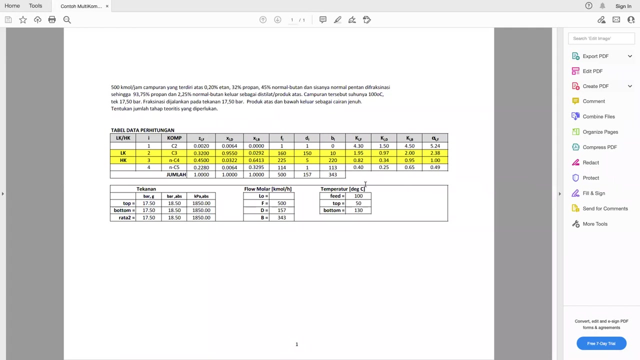 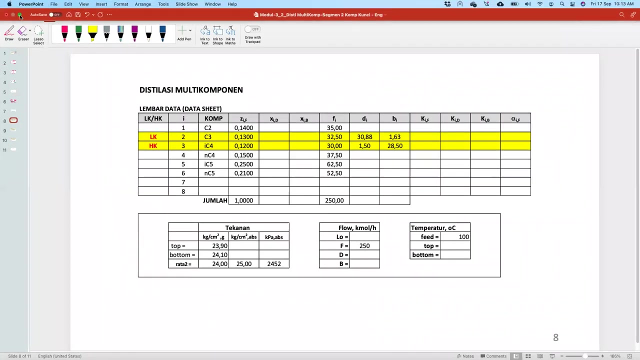 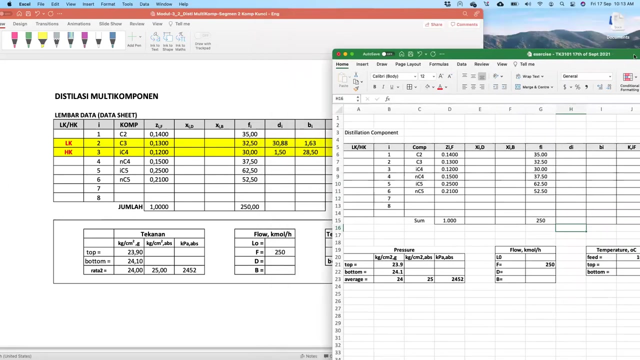 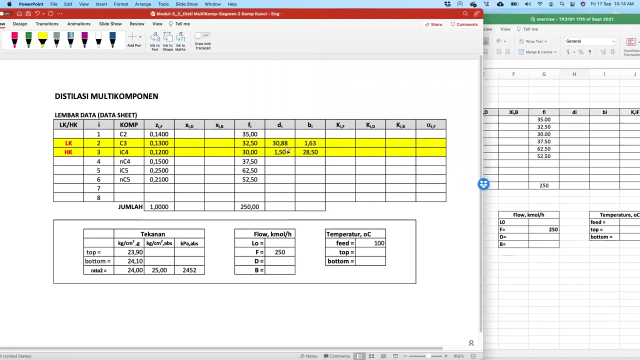 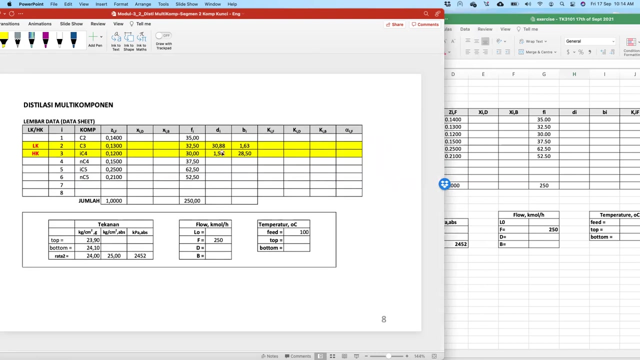 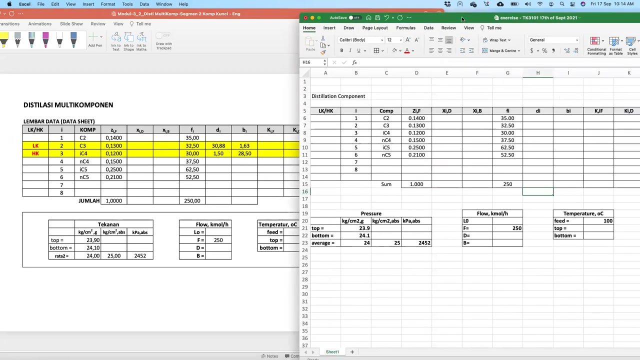 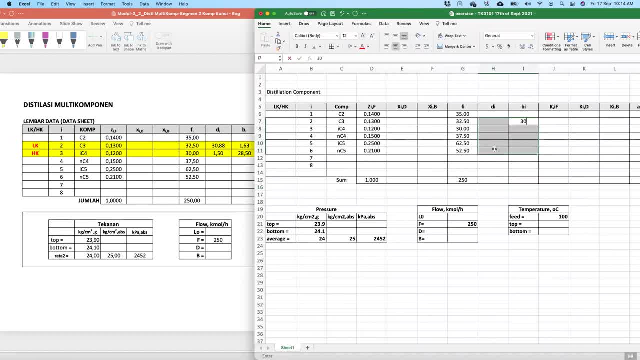 Just let's say, put it just the number there: Okay, 10.88.. Okay, So Okay, 1.63.. Let's say, let's say, this one is defined just from the, from the problems, yeah. 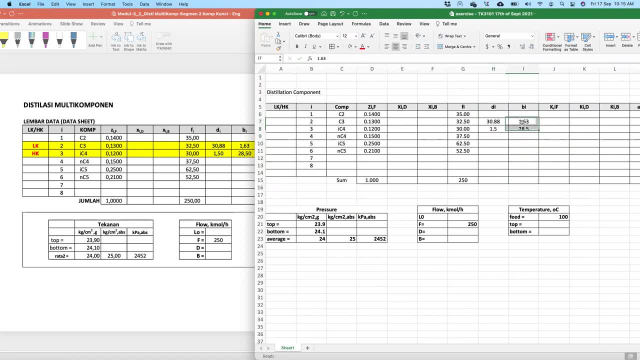 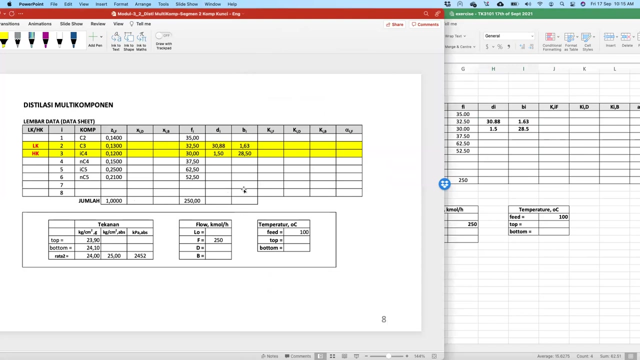 I got it from the teaching, Okay, anyway. Okay, I'm going to put it, maybe both, so it is based on the teaching. Okay, Okay, Okay, Okay On the problem. Okay, Now the next steps. what we're going to do is to to solve the mass balance. yeah, 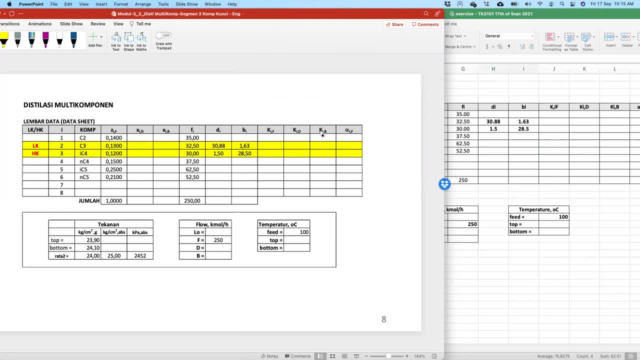 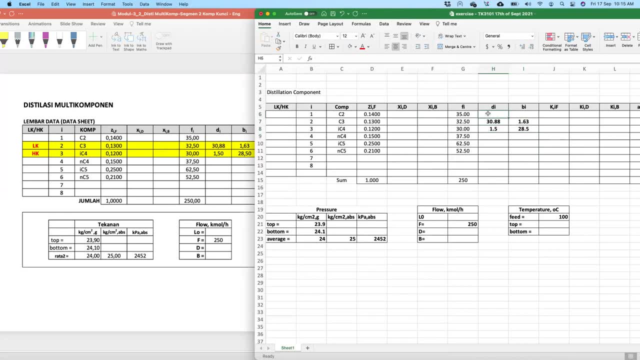 We have to solve the mass balance first. So by to what does it mean to solve the mass balance? Then we have to find all the components in the distillate and in the bottom. In this case they don't. they don't specify which one goes to distillate and which one goes to distillate. 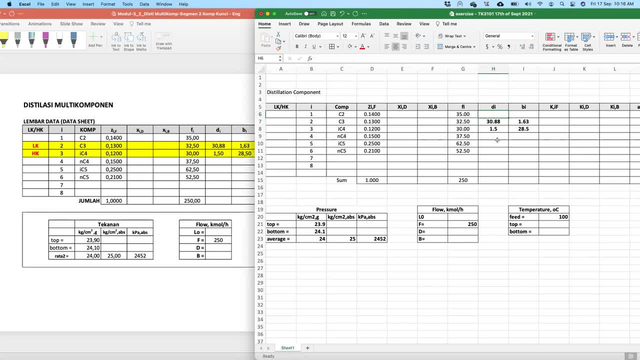 Okay, To the bottom. Okay, So what should we do? Okay, Okay. So what should we do? First looking back, and then this is written as the light key and this one is written as the heavy key. 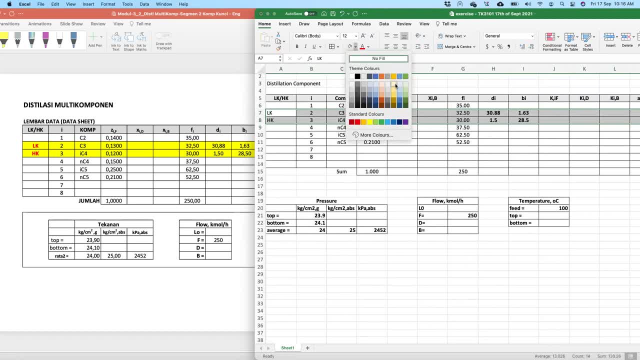 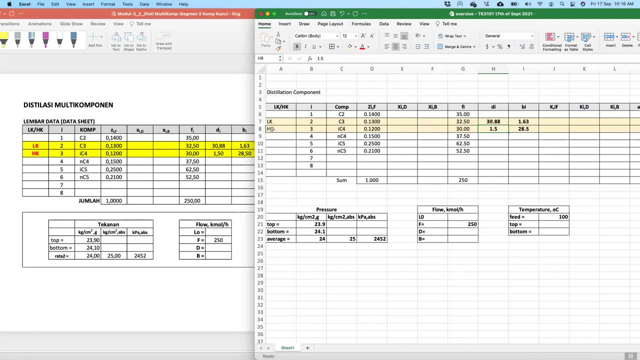 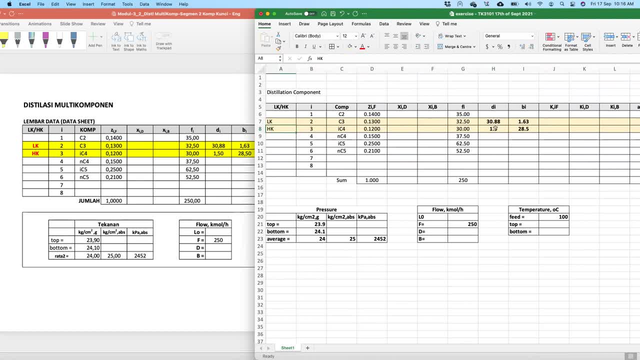 again, the most important component, uh, that present in the distillate. yeah, so, because it, and also uh, and it happens in small amount, so because of that we can uh the. the other heavier than uh heavy key is not important here. so we can assume, see, we can assume, that, uh, this actually become zero, which is 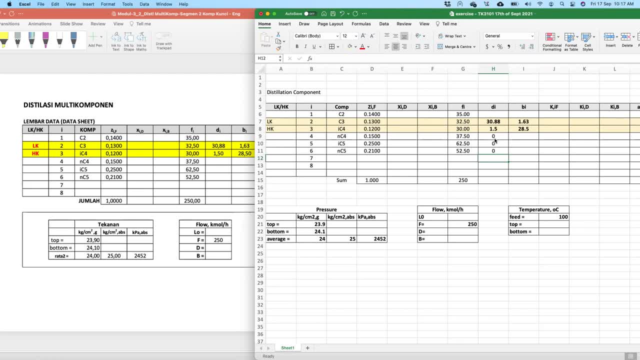 um, uh, this is an assumption. yeah, which is it met? it might not be, uh, right, okay, so i'm just gonna put this one as assumption, but uh, maybe put it with uh a red one, because we don't know. yeah, okay, we don't know. okay, and this one. 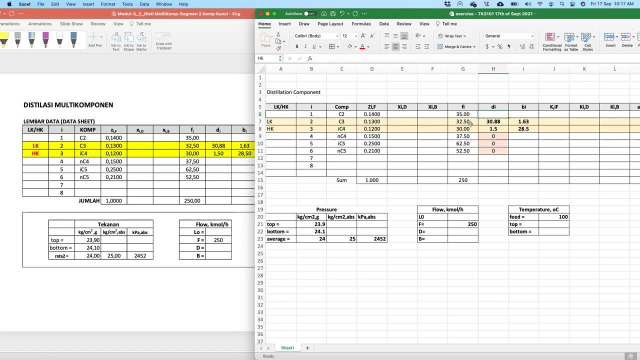 because on uh, here, from here, uh, 32.5, 30 goes to distillate. uh, it is, uh, some of them go to the bottom. so, in logically, if we have a component which is lighter than this one, so all of them should goes into the distillate. yeah, so i'm gonna write: this is s35. 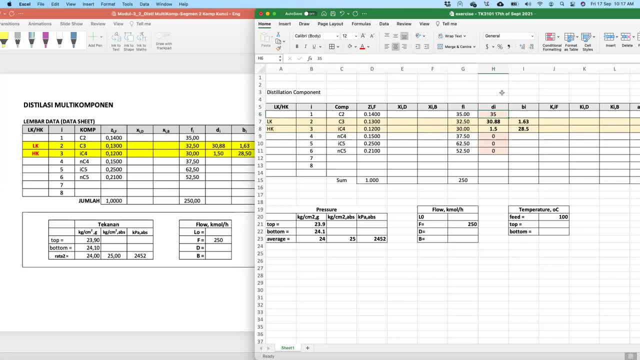 again with uh assumption and maybe, so there is nothing in the bottom- for the very uh, the situ, the, the lightest component, yeah, uh, so again, this is uh, i mean, this is gonna be the uh assumption, okay, and to get the uh d, uh, b, i, so then of course, uh, that's equal to b, uh, uh, the equal of the. 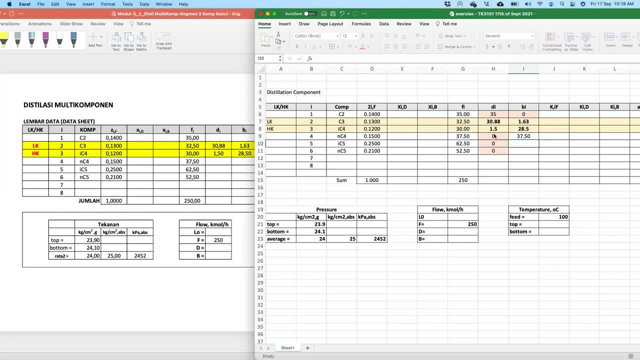 component in the feed minus the component in the distillate. so this is my, uh, my assumption. okay, the assumption can be right, can be wrong. yeah, uh with. so now we know the uh amount of distillate and the bottom yeah uh for each phase, and then we can sum it up. 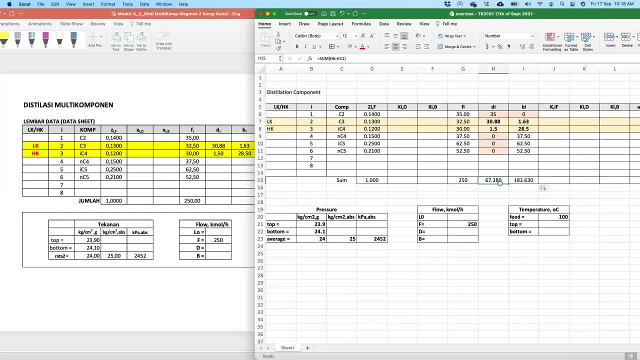 okay. so then we have uh 67.3, 80 and in the distillate and also 182 in the bottom. okay, the next step is to find the xid, which is the composition of the distillate. can you do that using the composition of the, the amount of distillate? 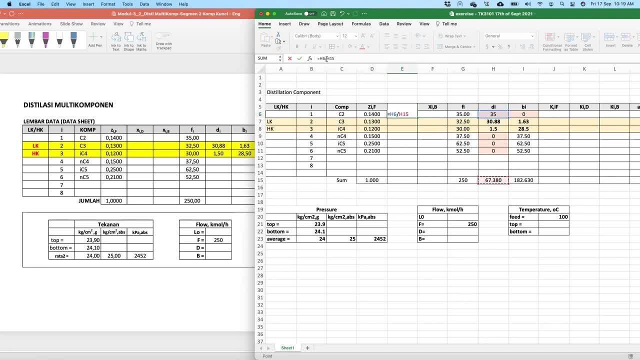 divided by the total in the distillate. okay, and then put it there, thing, and then this is the one, and then maybe make it easy. this is nice, okay. with similar question, with similar approach also, we can find the composition of the bottom by, uh, dividing the bi with the total. 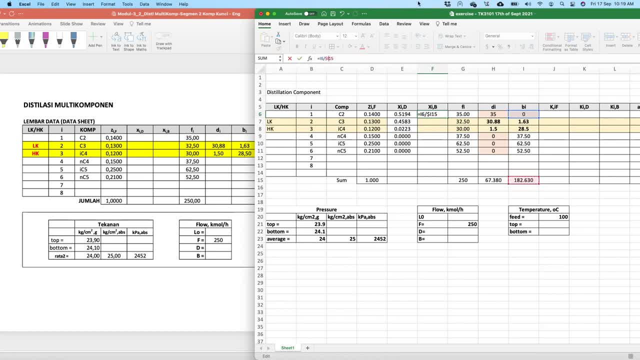 of the bi with again with the dollar. so, uh, we can have that one there, okay. so all of those uh numbers there, the one that is right, maybe only the heavy key and the light key, but the others is uh would be an example. uh, would be some assumption, okay to make to check it. let's sum it up. 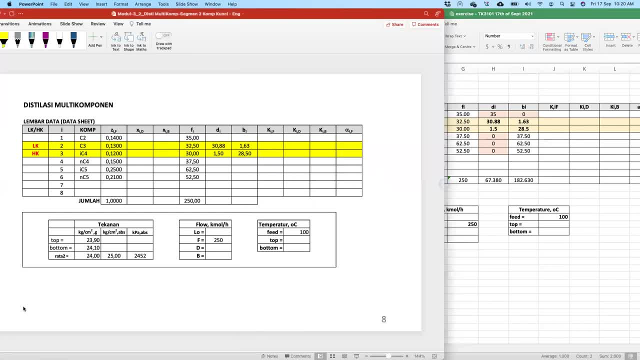 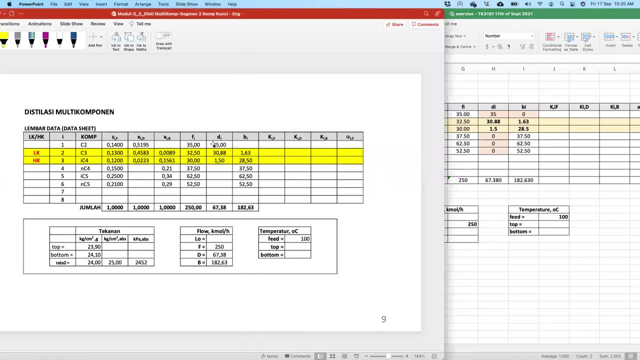 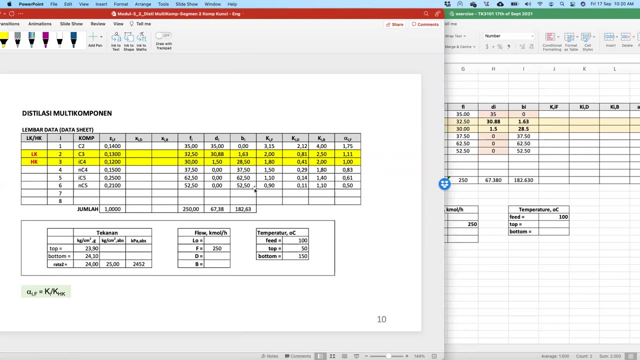 there, okay, so here your mass balance is finished. okay, see, so we put the uh, the distillate up to here, and then we have, uh, those compositions. okay, now, uh, the next step, this one, okay, the next step to get this one here. then you want to find the uh, the k. 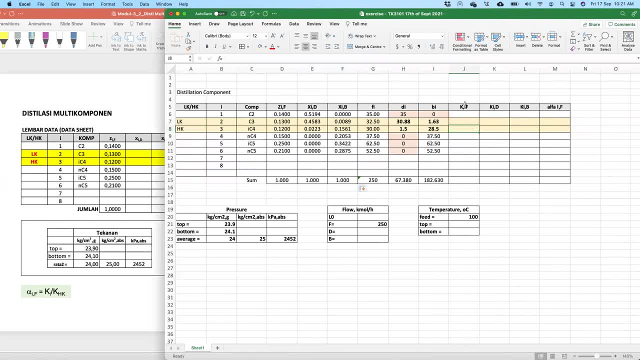 uh, the k fit. yeah, you want to find the k. what is the composition of k and what is the? the formula for k? it's actually y divided by x. yeah, but to get the y to uh and x, you have to um to find k. what should we do? 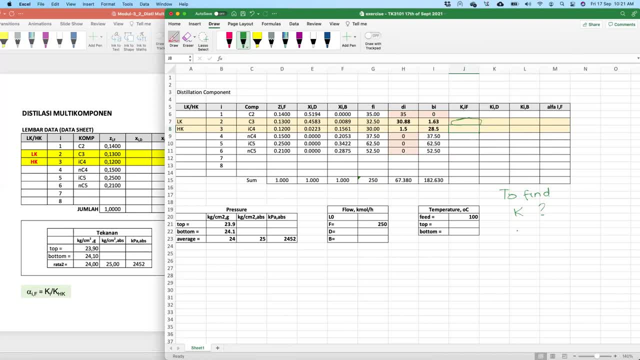 the k of component- example, this one- we have to check the nomogram. yeah, because k is a function of pressure and temperature. yeah, so that's why we have to find the the k i feed, which is k at a temperature. in the temperature of feet. we have to find the temperature. 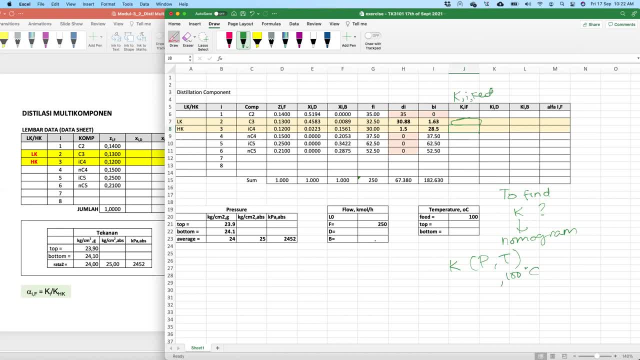 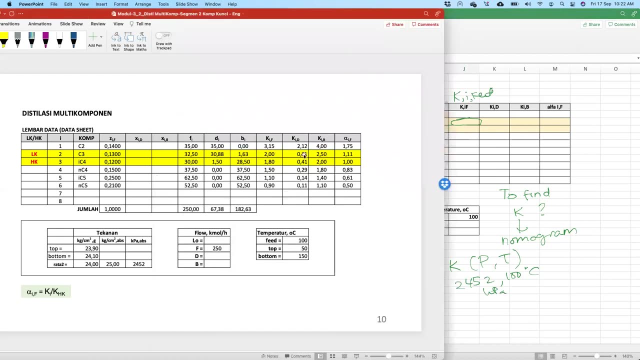 for example, 100 degrees celsius, and then the pressure around uh, two, four, five, two, yeah, uh, kilopascal, uh, and then find it, uh, the k value, yeah, and then uh, here, uh, they find the k value is around, uh, this, this part there, okay, and then uh, so it is, it is. i know this is gonna be time consuming, so from here then you. 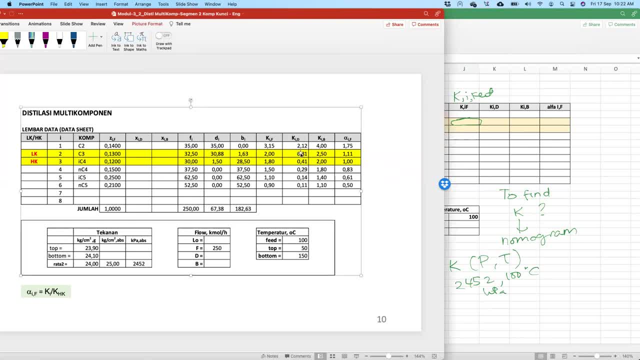 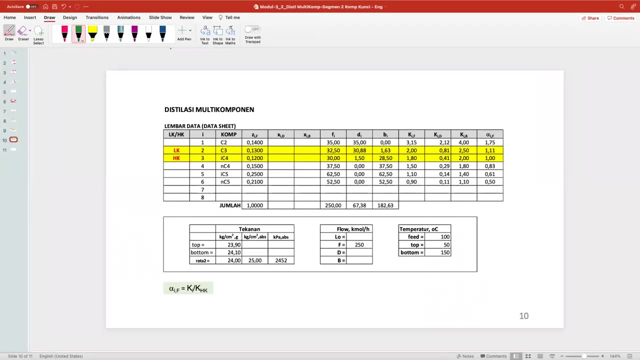 can find, uh, the all of the k value. uh, for each component. yeah, for each component. uh, which is the? i'm gonna go back here. okay, um, and the component here. so find the component at, for example, the pressure is 2452 when temperature is 100 degrees celsius. okay, how about the distillate? 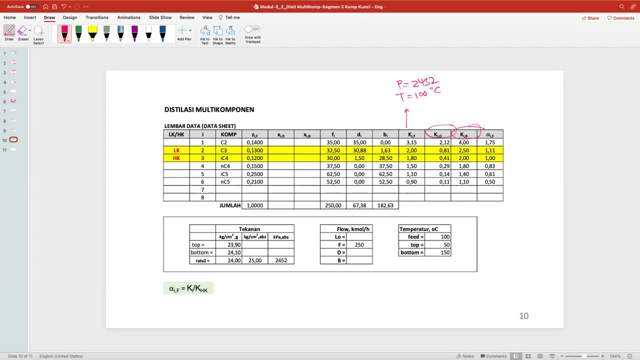 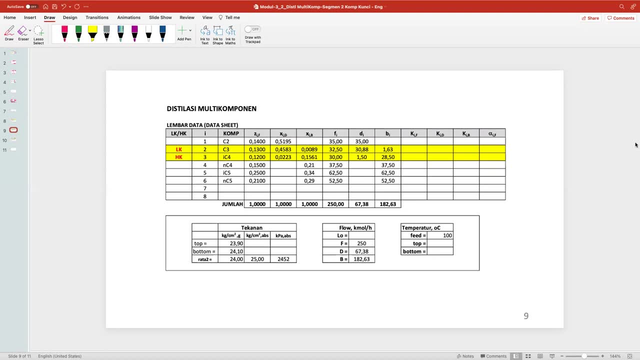 can you? can you know the, the, the pressure? uh, can you know the temperature of distillate and the bottom based from here? can you get it, the temperature? anyone? do we have temperature in the problem? of course not. yeah, we don't know which one is the temperature, top and also with. 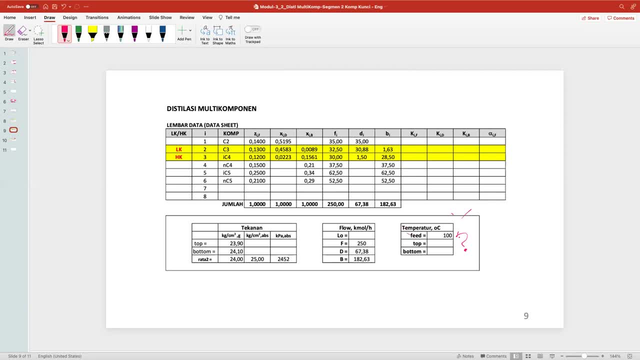 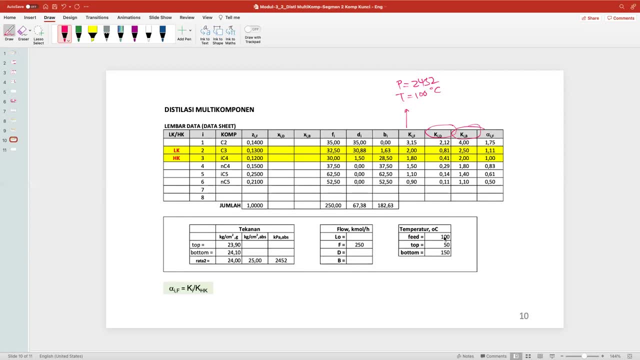 uh, which one is the temperature of the bottom, you see? okay, so again, this also is uh assumption. okay, so again, this also is uh assumption. okay, so again, this also is uh assumption. that's why later the process is very, that's why later the process is very. 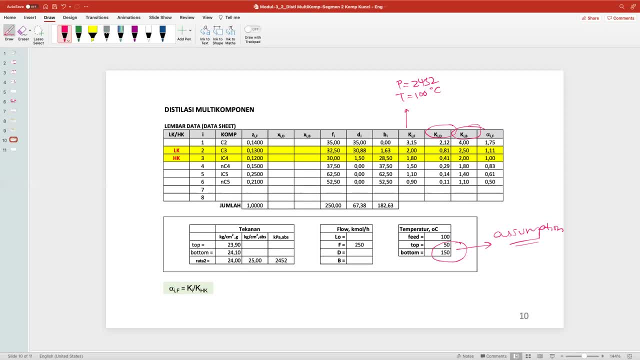 that's why later the process is very attractive. yeah, that's why we attractive. yeah, that's why we attractive. yeah, that's why we we're not going to use it as an exam. yeah, you, we're not going to use it as an exam. yeah, you, we're not going to use it as an exam. yeah, you can just only a good group assignment. 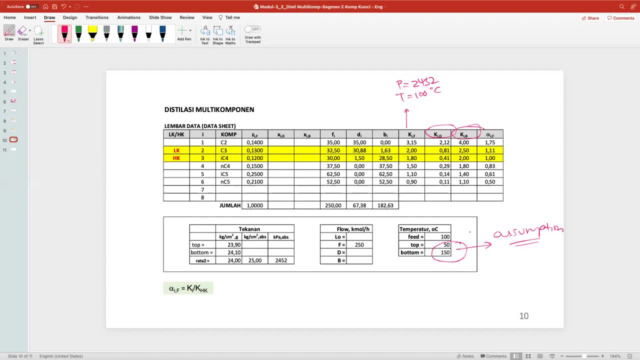 can just only a good group assignment, can just only a good group assignment- basically gonna take long time. yeah, uh, basically gonna take long time. yeah, uh, basically gonna take long time. yeah, uh, big uh, if we don't uh, of course we don't. big uh, if we don't uh, of course we don't. 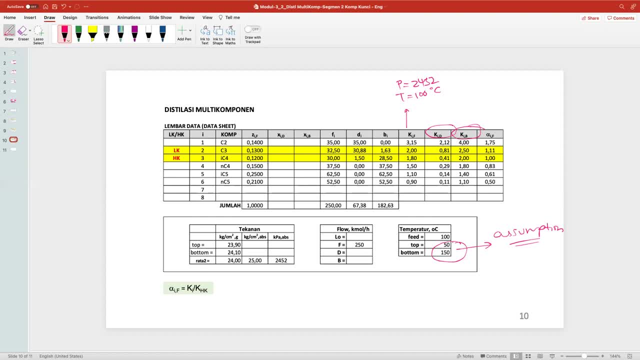 big. uh, if we don't, uh, of course we don't know which one is the top and which is know which one is the top and which is know which one is the top and which is in the bottom, in the bottom, in the bottom, uh, then we can do some assumption, uh. 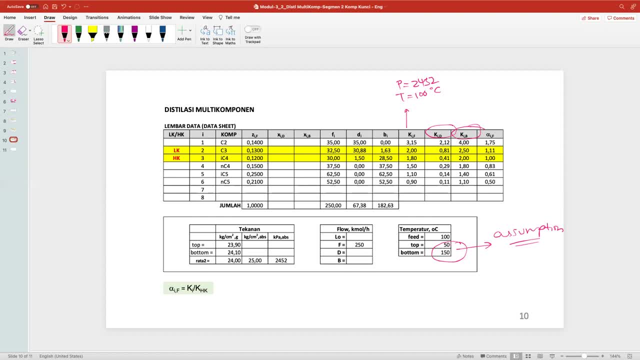 uh, then we can do some assumption. uh. uh, then we can do some assumption. uh, this assumption 50 is also usually based. this assumption 50 is also usually based. this assumption 50 is also usually based on the, on the, on the cooling water, so let's say the cooling. 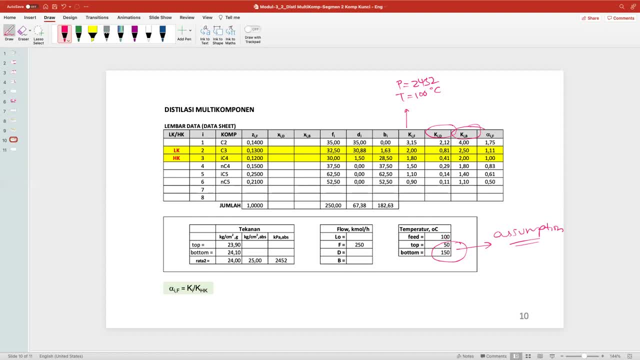 cooling water, so let's say the cooling cooling water. so let's say the cooling water is up to water is up to, water is up to 25 degree to 35 degree. so the top one: 25 degree to 35 degree. so the top one: 25 degree to 35 degree. so the top one should be, uh yeah, around 10 to 15 after. 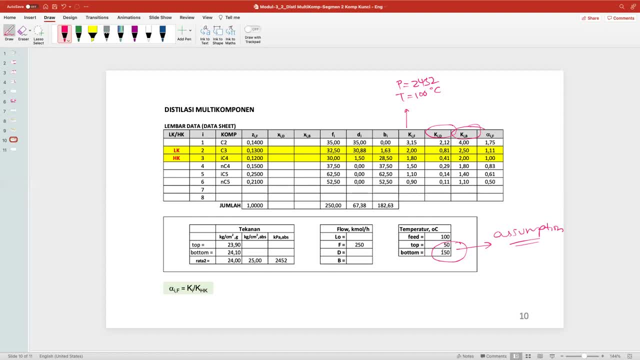 should be: uh, yeah, around 10 to 15 after. should be: uh, yeah, around 10 to 15 after that, so around 50 degrees, i shift okay that. so around 50 degrees, i shift, okay that. so around 50 degrees, i shift okay. and the bottom we also assume, uh, it. 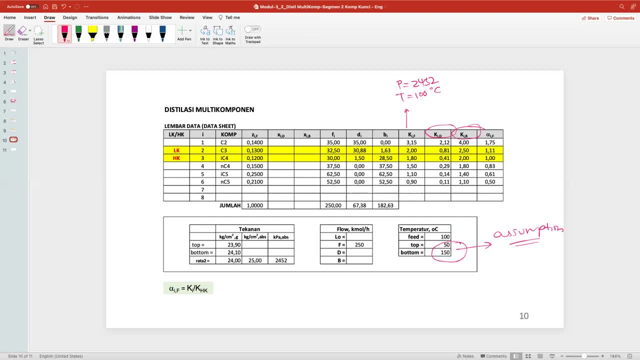 and the bottom. we also assume uh it and the bottom. we also assume uh it should be more than 100. uh should be more than 100. uh should be more than 100. uh should be long enough. maybe so if uh the should be long enough, maybe so if uh the. 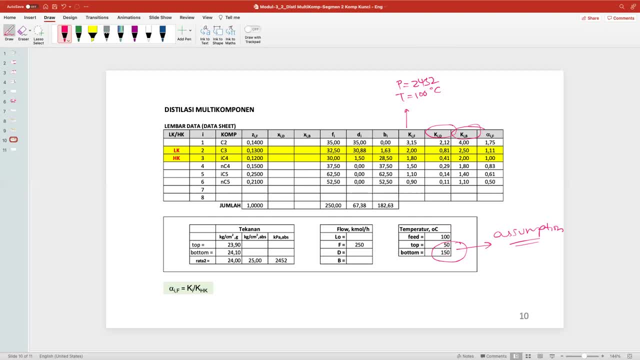 should be long enough, maybe. so if, uh, the delta between here is 50, so maybe we delta between here is 50, so maybe we delta between here is 50, so maybe we also add 50 from the, also add 50 from the, also add 50 from the feed temperature, so around 150 degrees. 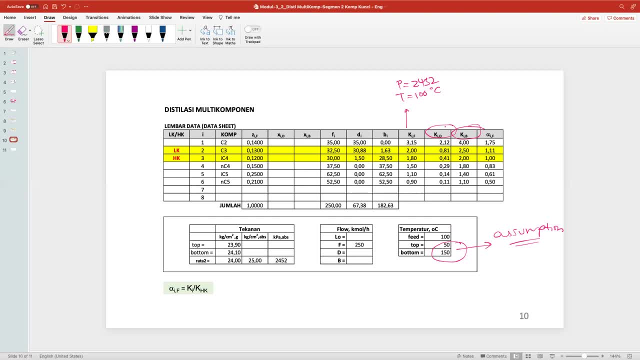 feed temperature, so around 150 degrees. feed temperature, so around 150 degrees celsius. right. so then, with that, uh, we celsius, right. so then, with that, uh, we celsius, right. so then, with that, uh, we assume, uh, assume, assume, assume. t distillate is uh. 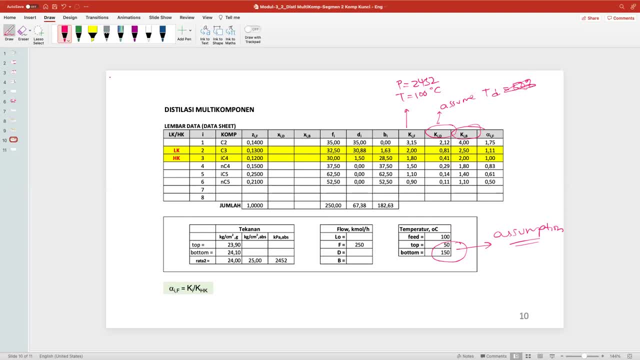 t distillate is uh, t distillate is uh. 50 degrees celsius, 50 degrees celsius, 50 degrees celsius, sorry, 50 degrees celsius and also um 50 degrees celsius, while the t bottom of 50 degrees celsius, while the t bottom of. 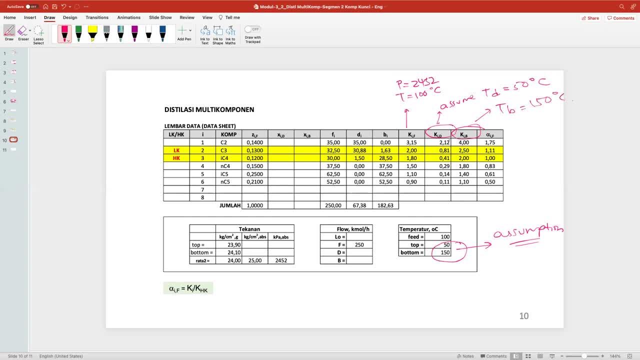 50 degrees celsius, while the t bottom of 150 degrees celsius, okay. once you know 150 degrees celsius, okay, once you know 150 degrees celsius, okay. once you know the k, the k, the k, uh, all of them, then you can find the. 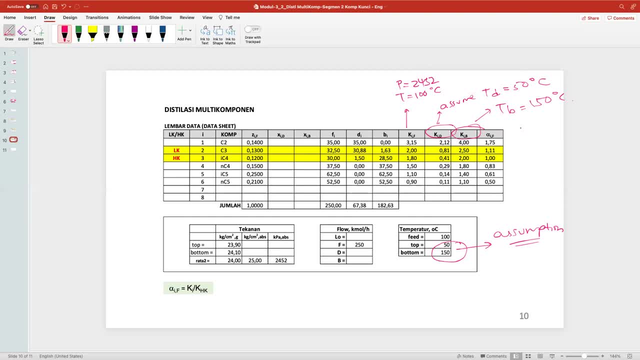 uh, all of them, then you can find the. uh, all of them, then you can find the. alpha, alpha, alpha- yeah, why we need alpha alpha is, yeah, why we need alpha alpha is, yeah, why we need alpha. alpha is defined as defined as defined as a k of the: i, the component i divide by: 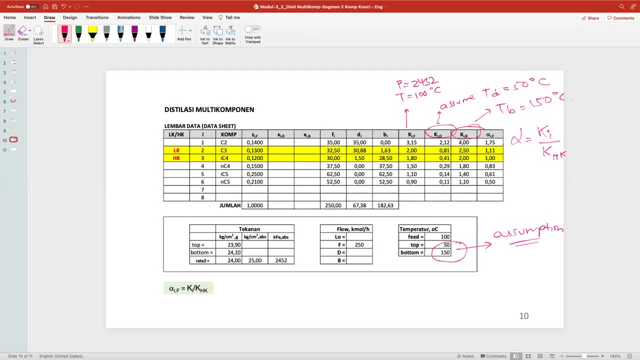 a k of the i, the component i divide by a k of the i, the component i divide by k, h, k, k, h, k, k, h k. this is just to to check the uh. this is just to to check the uh. this is just to to check the uh. to check the relative volatility. 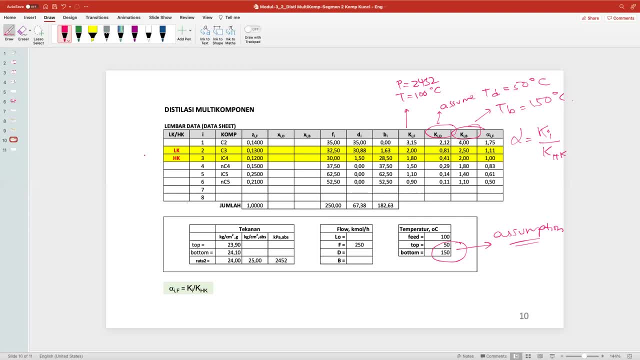 to check the relative volatility. to check the relative volatility, uh to the heavy key. yeah, because the uh to the heavy key. yeah, because the uh to the heavy key. yeah, because the heavy key that we heavy key, that we heavy key that we define is the ic4. 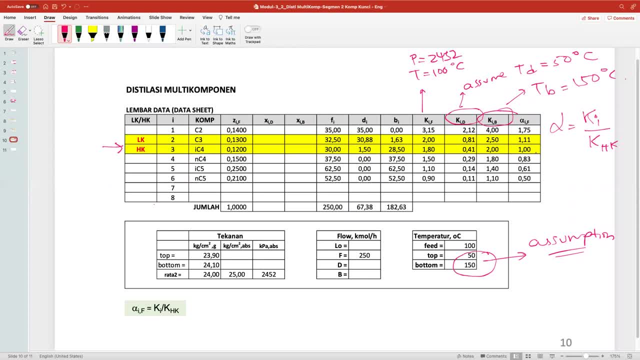 define is the ic4. define: is the ic4, then uh for ic4, the volatility relative, then uh for ic4, the volatility relative, then uh for ic4, the volatility relative. volatility is one, volatility is one, volatility is one and then uh, so this one as the component. 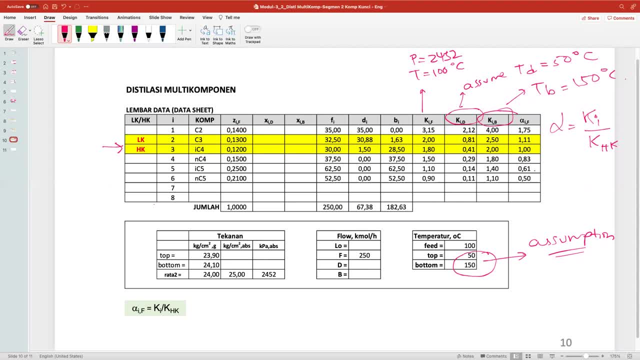 and then uh, so this one as the component, and then uh, so this one as the component is 1.75, is 1.75, is 1.75, 1.11, and then 2: 1, so this one is the 1.11, and then 2: 1, so this one is the. 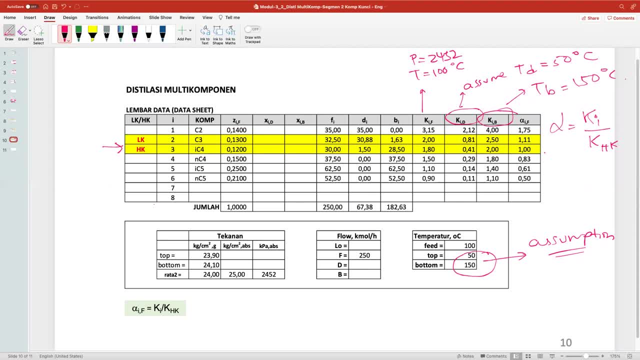 1.11 and then 2: 1, so this one is the- uh the key. uh sorry, the components that uh the key. uh sorry, the components that uh the key. uh sorry, the components that is heavier than the heavy key is heavier than the heavy key. 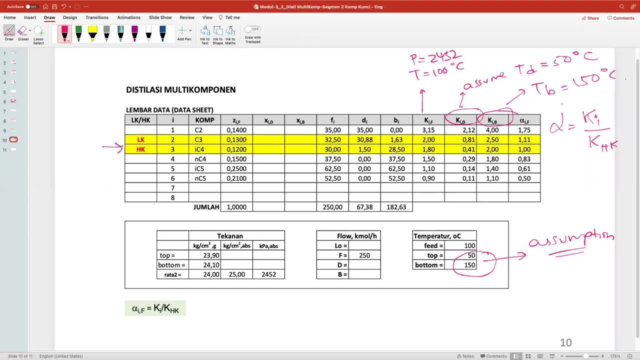 is heavier than the heavy key, and this one is the component that, and this one is the component that, and this one is the component that: lighter from the heavy key, lighter from the heavy key, lighter from the heavy key. all right, i'm gonna uh, stop it here and 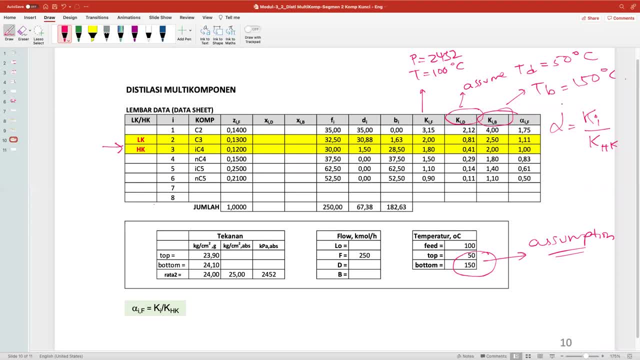 all right, i'm gonna uh stop it here, and all right, i'm gonna uh stop it here and then uh, then uh, then uh, maybe uh, and then let you uh, maybe uh, and then let you uh, maybe uh, and then let you uh digest this, and then let me know if you. 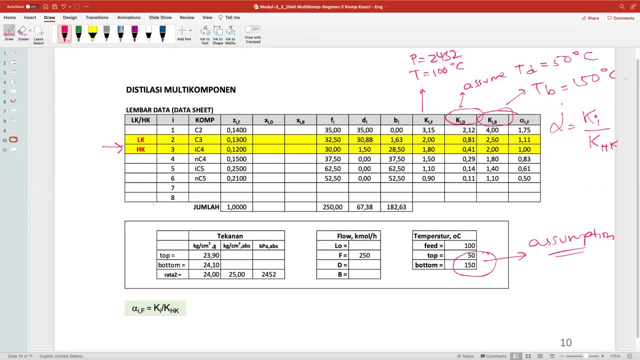 digest this, and then let me know if you digest this, and then let me know if you have any questions. okay, any questions, okay, any questions. everyone's quiet, still trying to digest. hello, yes, good digesting book, all right then. yes, good digesting book, all right then. 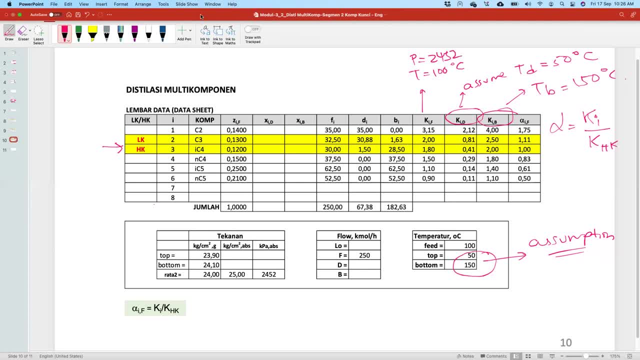 yes, good digesting book. all right then, uh right, uh anyway, uh right, uh anyway, uh right, uh anyway, uh. so what is why we have to calculate, uh so? what is why we have to calculate, uh? so? what is why we have to calculate this one, this one? 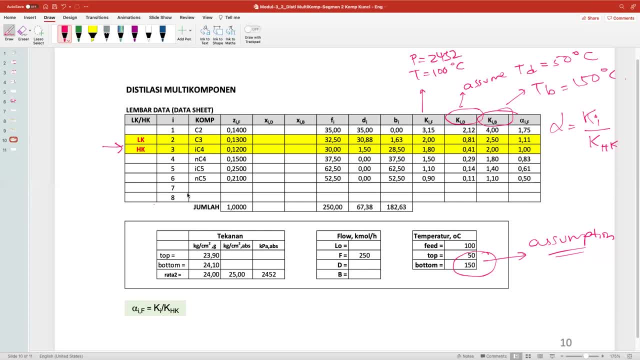 this one, uh, uh, because we want to calculate the number. uh, because we want to calculate the number, uh, because we want to calculate the number of equilibrium stages, of equilibrium stages, of equilibrium stages like in the binary. uh, uh, like in the binary, uh, uh, like in the binary. uh uh, distillation, right uh. 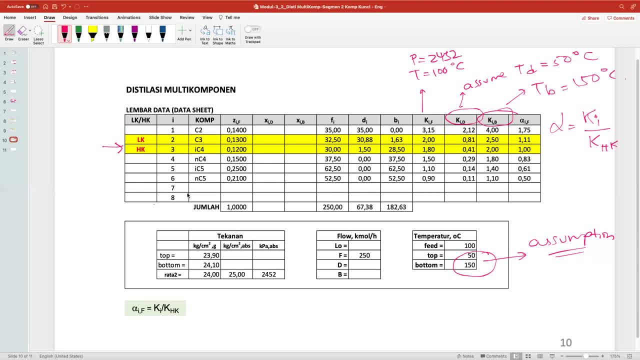 distillation right, uh. distillation right, uh, no, but. but i don't know why you have to no but. but i don't know why you have to no but. but i don't know why you have to find the k, why you have to find the. find the k, why you have to find the. 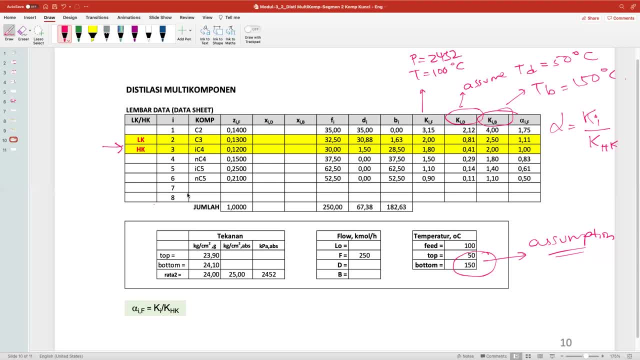 find the k, why you have to find the relative volatility, why you have to do relative volatility, why you have to do relative volatility, why you have to do a lot of assumption? why, if our a lot of assumption? why, if our a lot of assumption? why, if our assumption is wrong? of course, your 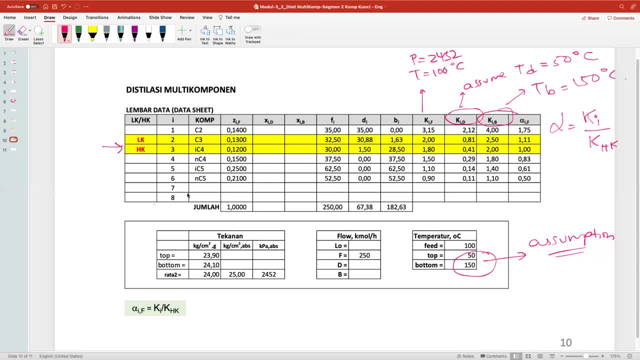 assumption is wrong. of course your assumption is wrong. of course your assumption will be wrong, okay, and then assumption will be wrong, okay, and then assumption will be wrong, okay, and then you have to do the iteration again, so you have to do the iteration again, so you have to do the iteration again. so it's going to be very, very painful. 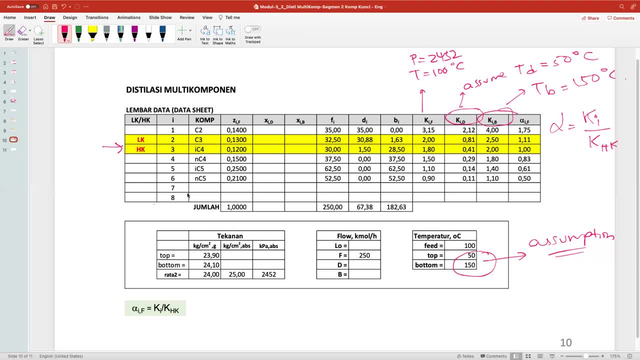 it's going to be very, very painful. it's going to be very, very painful anyway. um, i think there would be anyway. um, i think there would be anyway. um, i think there would be questions later. so i'm gonna continue to questions later. so i'm gonna continue to. 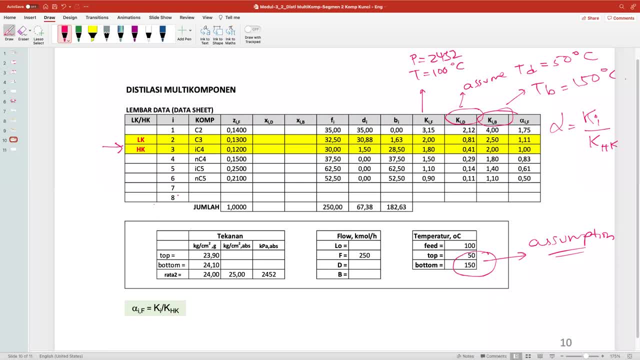 questions later, so i'm gonna continue to the next, the next, the next module. how to uh start module? how to uh start module? how to uh start calculating the the equilibrium? yeah, calculating the the equilibrium? yeah. calculating the the equilibrium, yeah, the equilibrium stage, uh for the equilibrium stage, uh for. 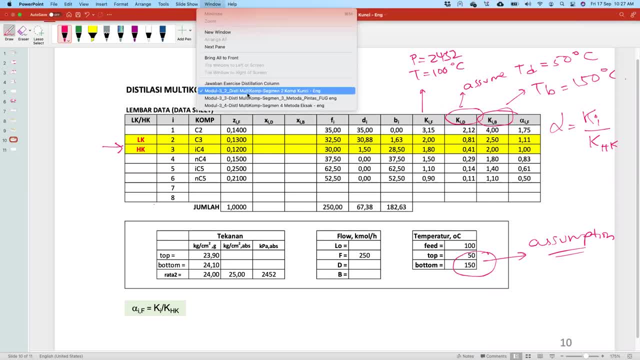 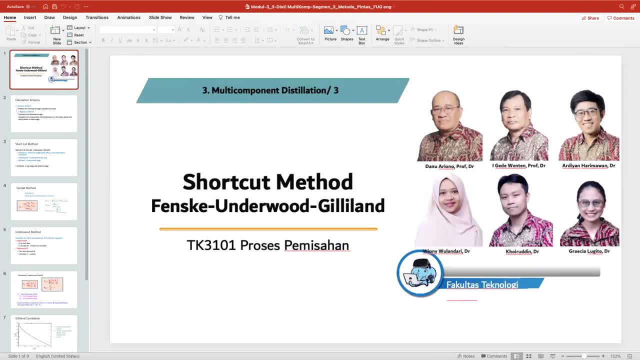 the equilibrium stage. uh, for multi-component distillation. okay, let's go to the next stage. uh, for okay, let's go to the next stage. uh, for okay, let's go to the next stage. uh, for we called it. uh, we called it, uh, we called it uh. method of pin pass or shortcut method. 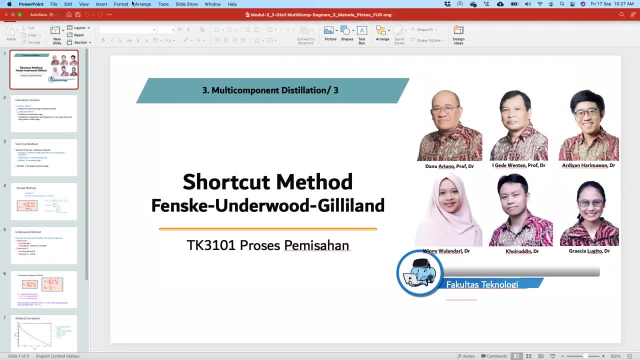 method of pin pass or shortcut method. method of pin pass or shortcut method: right, right, right, okay, but before that looks like i need a okay, but before that looks like i need a okay, but before that looks like i need a drink, drink, drink. so i'm gonna pause a few minutes and 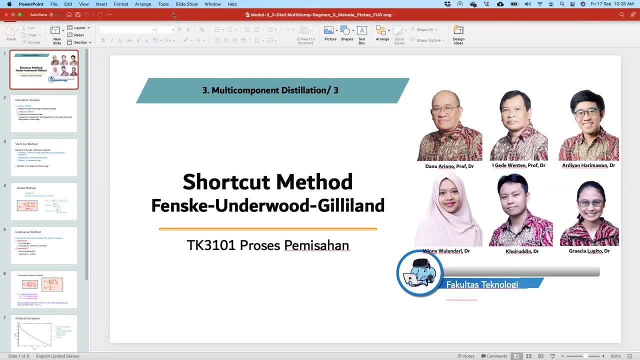 so i'm gonna pause a few minutes, and so i'm gonna pause a few minutes and then i'll get back to you, then i'll get back to you, then i'll get back to you. okay, uh, let's okay, uh, let's okay. uh, let's continue. 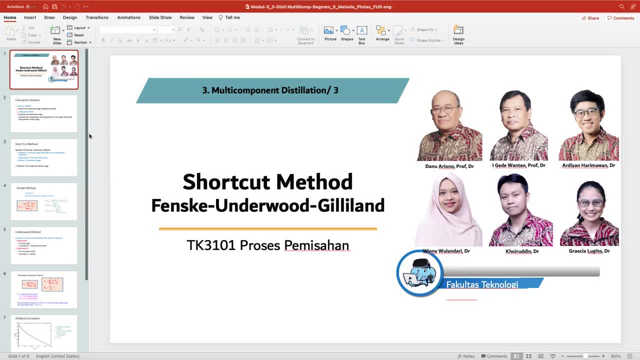 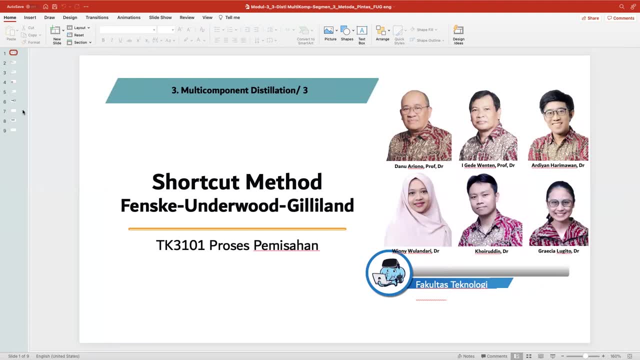 continue the shortcut method. uh, why? why it's called the shortcut method? because of method of pintas? uh, it's because, uh, we uh it is not accurate. yeah, it is not accurate, but it can give you some valuable information that's uh not mentioned in the problems. okay, uh, so later we're gonna. 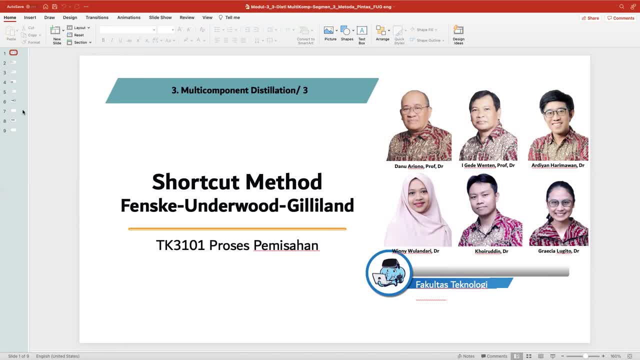 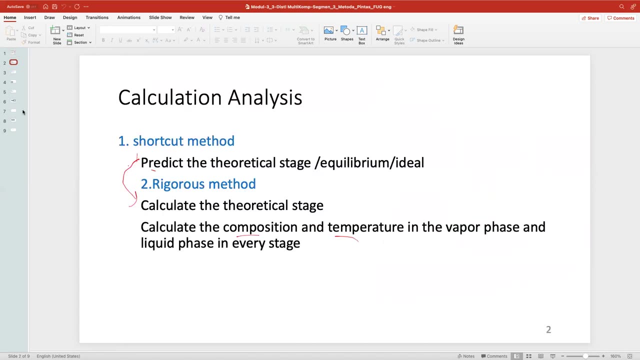 continue about. uh, there are shortcut method and next week, uh also, then we're gonna continue with, or next week is exam for the next week after, uh, is the uh rigorous method or the exact method, right, uh, okay, so, uh, what is the, the, the propose of the shortcut method? 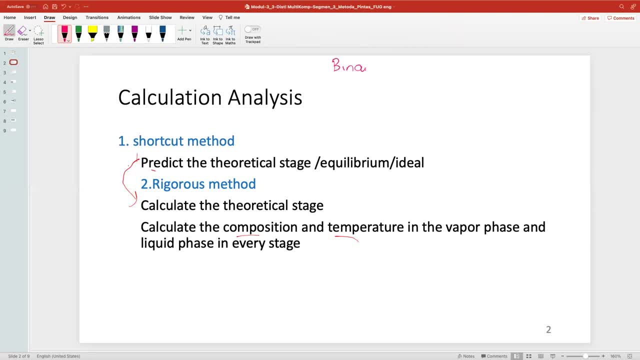 uh, just to recall, in binary distillation now, because we're gonna have the exam so in Nedim, if you're just like wait one minute, no, I'm gonna talk about the Q law and we have a question from whoreway. that is, what do we need to? uh, to. 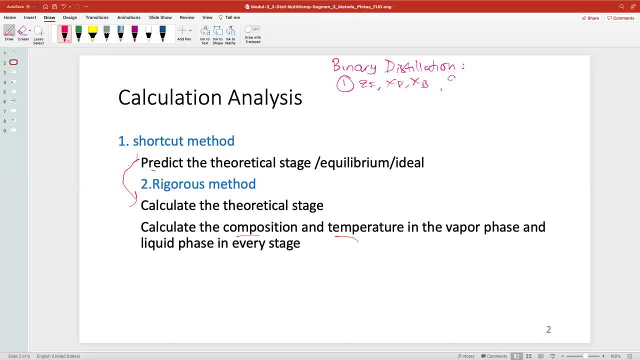 to build the, the equilibrium stages we need to find. once we know the zx, f, uh, xd and xb. yeah, Once we know the RM, we can find the R, and once we find the R, we can find the intercept and then we can find the stages or the end. okay, 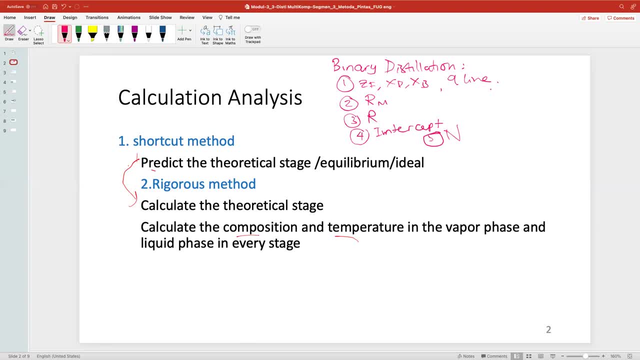 Now this also happens in the multi-component distillation. We need to find the RM, yeah, We want to find also the R, and then we also want to find the N, okay, So this shortcut method is to find these things okay. 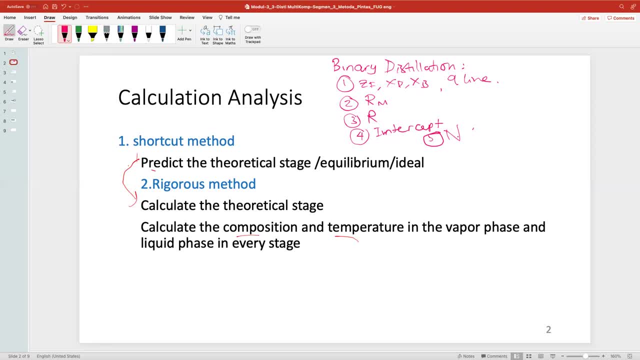 But this only you know, only the shortcut way. yeah, So it only predicts the theoretical stage on the equilibrium of ideal. However, in the multi-component distillation, we want to know in each stage what is the composition in each stage. 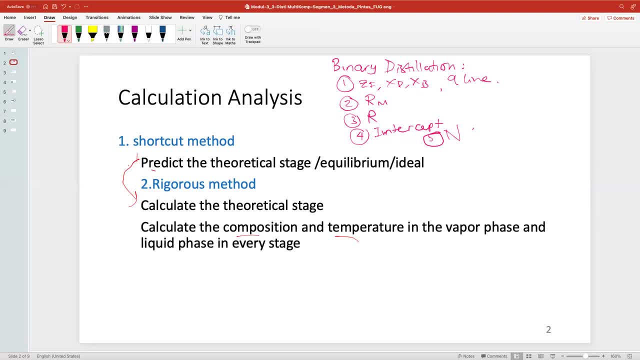 So if we want to do a side-by-side drawing, yeah, or we want to add multiple feet, we can understand where we have to put it right. For example, we have a crude oil distillation and then if we have so many components to deal with, 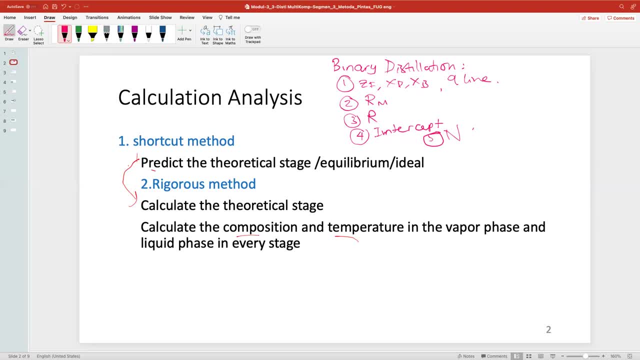 in which stage that we can withdraw propane, for example. In which stage we can propane we can withdraw pentane, yeah, or maybe hexane, for example. Where is it Then? we have to check with the composition, okay. 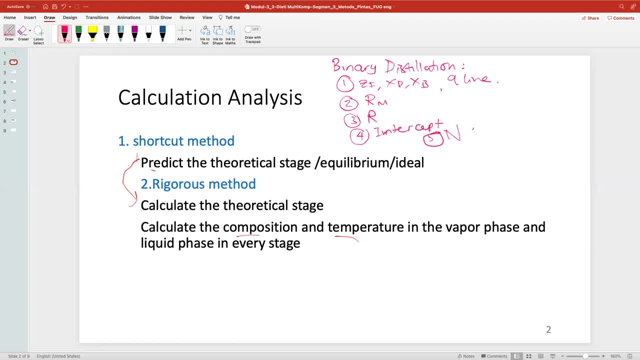 So the shortcut method is to predict the theoretical stage, or equilibrium, or the ideal Well, later on. the second one is the rigorous method, or the exact method is to recalculate the theoretical stage. Sometimes our assumption here can be maybe deviated about one to three stages. 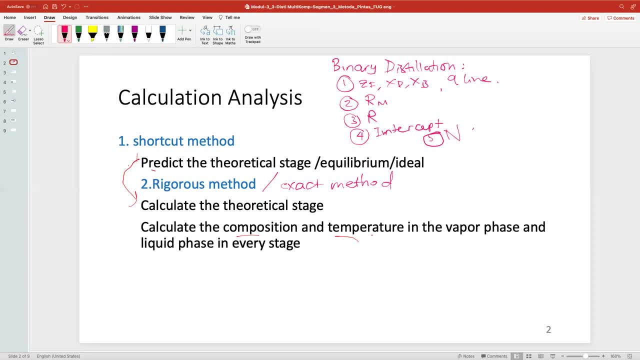 And then also we want to calculate the composition and temperature in the vapor phase and liquid phase at every stage. So we can do that. okay, We will do that using some, using the spreadsheet, the Excel, And later, maybe the next two weeks or three weeks after we're going to also complement that with so high-seas yeah. 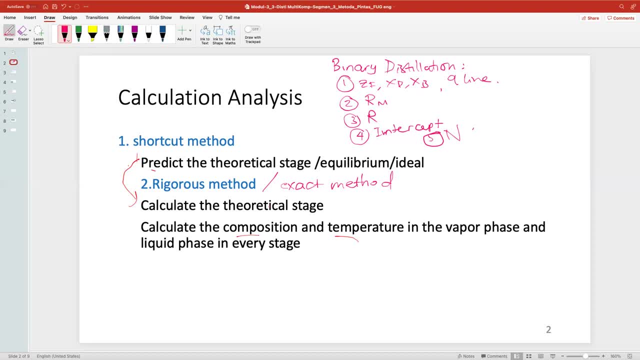 So if you can install high-seas from the program study, you can do so. There would be some yeah. so that because I will also explain to you how to do it in high-seas. Of course that's going to be much faster, but because we're training, yeah, to understand the design process and then, of course, this one. 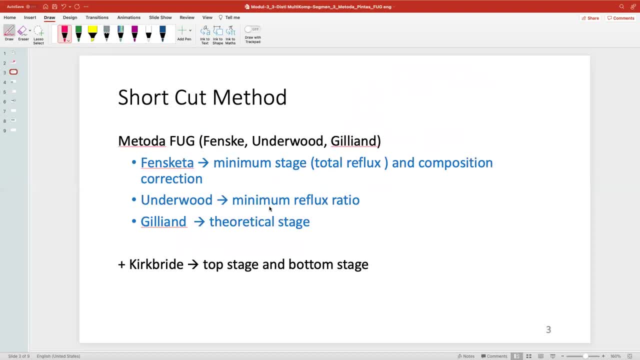 is the one that we need to pass on. Okay, The shortcut method is called FUG or the Fast-Cut Method. Fenske, Underwood and Gilliland, Gilliland or Gillian, I think Gilliland yeah. 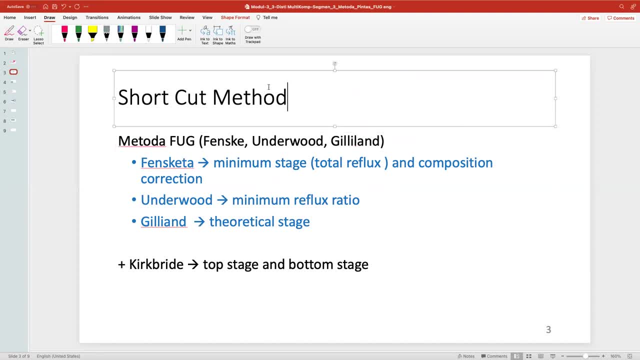 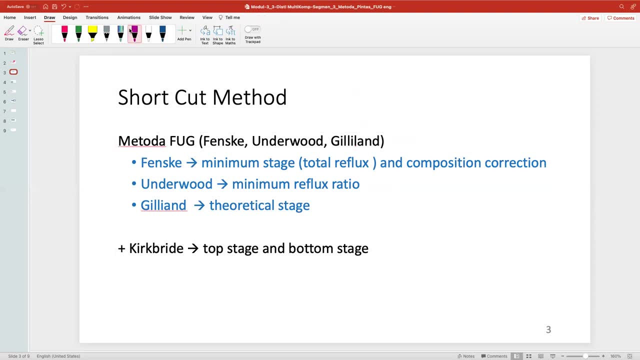 Gilliland, Gilliland, Right, Fenske. Okay, So the Fenske is to find the minimum stage of stage. So Fenske is to find the minimum stage or NM, the total reflux And also the composition. 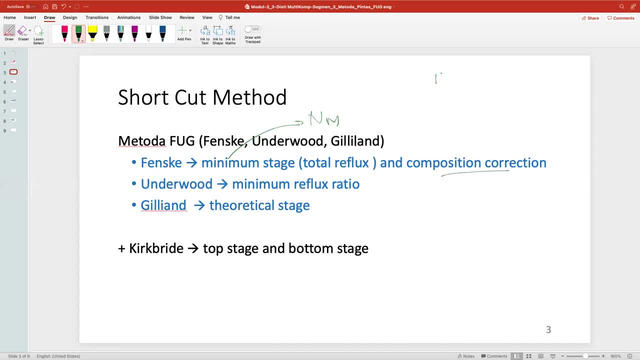 So the composition correction, Remember from our mass balance that we do before mass balance. we put some, we put some assumptions right, We put that, okay, there's nothing heavier than the heavy key There's. All of the C2 goes through the distillate. 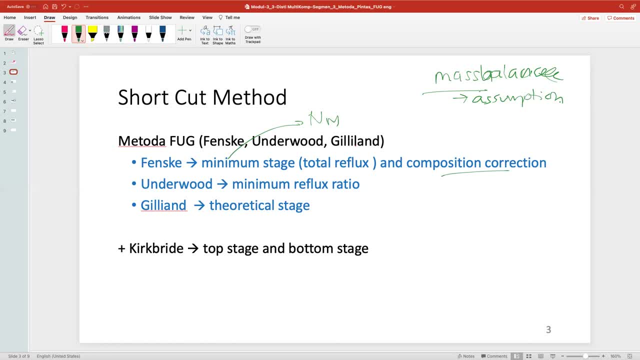 That is just assumption, But is it right or not? have to check it first and then we have to done the composition correction. The second one is the Underwood, or to find the minimum reflux ratio. This one is to find DRM and the Gilliland. 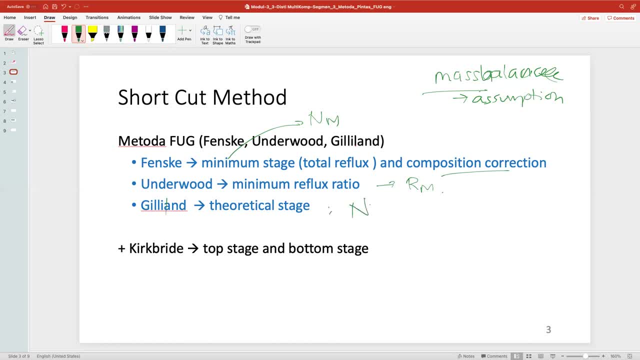 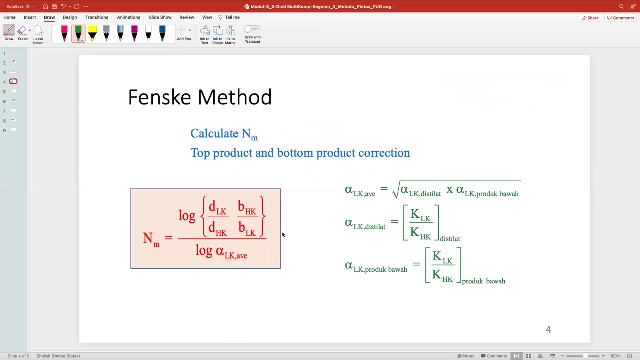 to find the tertic of H or N. There's one more correlation, which is Kirkbride. This is to find which one goes to the top stage and which one goes to the bottom stage. but sometimes it's not really accurate. So then, sometimes we can leave it, sometimes we can use it. Let's check one by one. 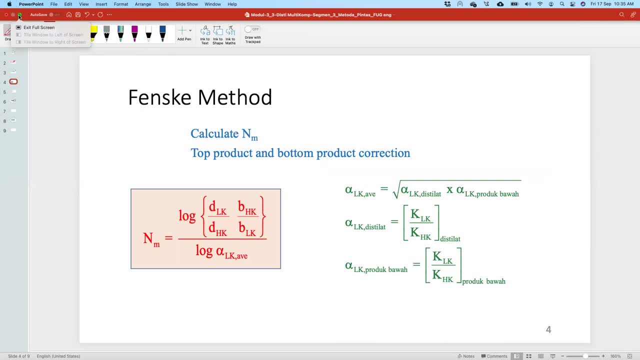 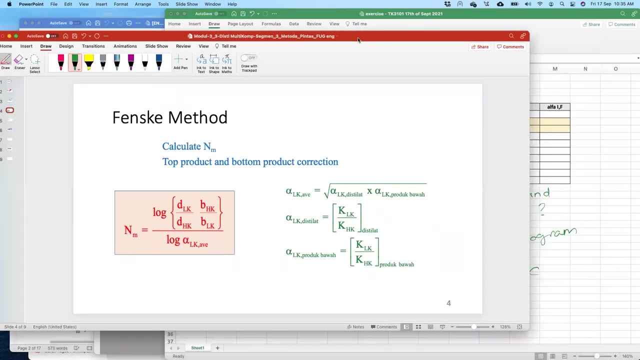 To calculate this one. we have to. so this is the Fenske method, that is, to calculate NM with the top and bottom product correction. The Fenske. I'm gonna make it smaller there because I'm gonna go back to here. 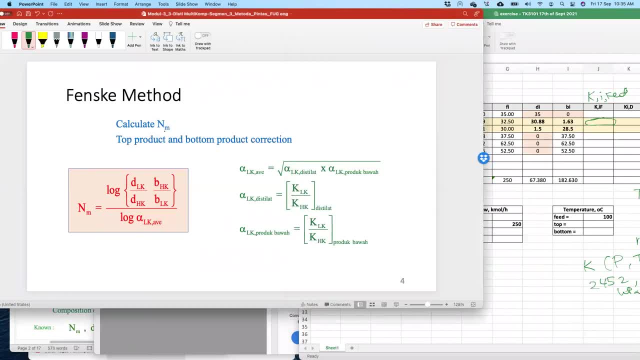 The Fenske method is to calculate NM and the NM is defined as log of DRM. NM is defined as the LK and BHK divided by DHK, multiplied with the clk, so the decilate, yeah, and divided by log alpha LK average. So this is how to get the alpha LK average. 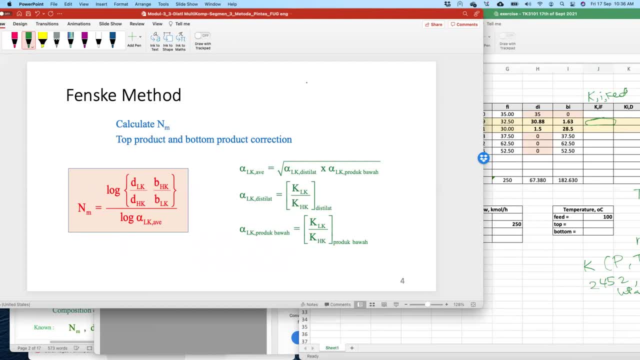 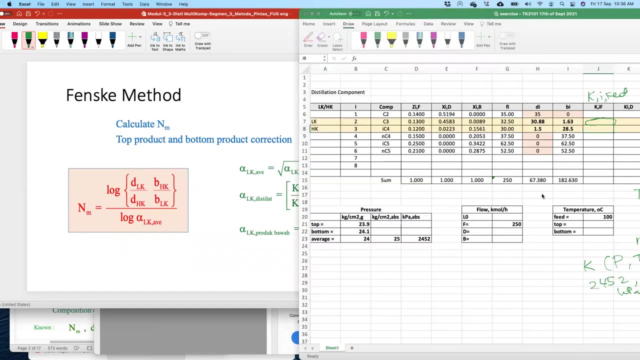 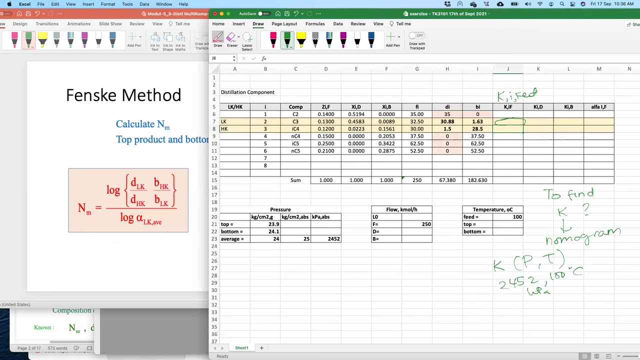 So that means we have to find K, LK, KHK and so on. okay, so that's why we have to use this one there. yeah, that's why we have to fill this one before we use the transfer method. let's erase this one to make it easier. and then let's say: I do the nomograms, I'm checking the K value. 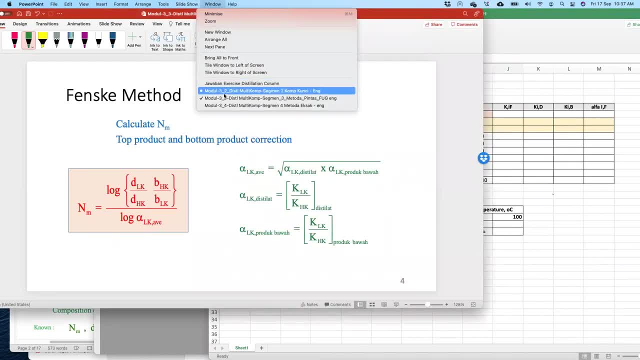 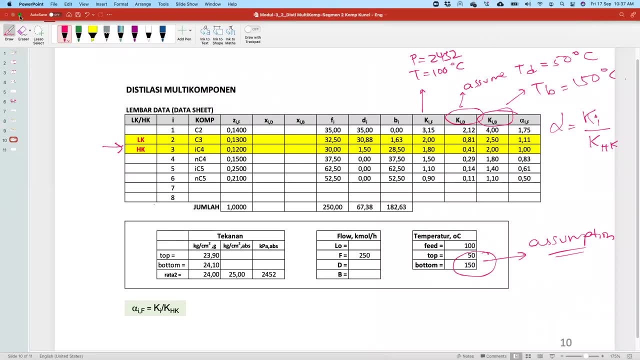 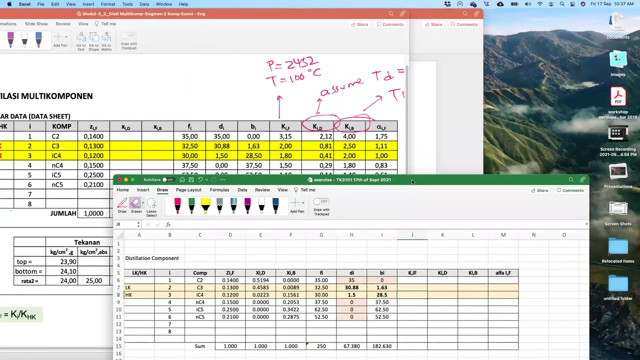 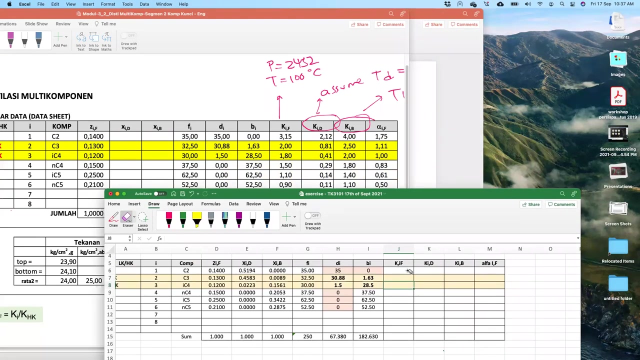 and I got the perfect one. yeah, yeah, this one. let's just put it back, okay, just to make sure. okay, let's say I copy them. and then I got: this is K. I took 135. for example, this is 315. I got this one s2, and then 1.8, and then 1.5. 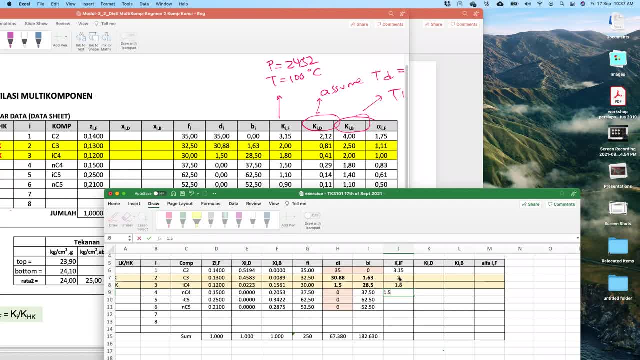 two: 1.8, 1.5, 110 and 0.1. i got it from, uh, my calculation, yeah, trying to find it, and i got the kip: it's 4, 2.5, 2.0, 1.8, 1.4 and 1.. 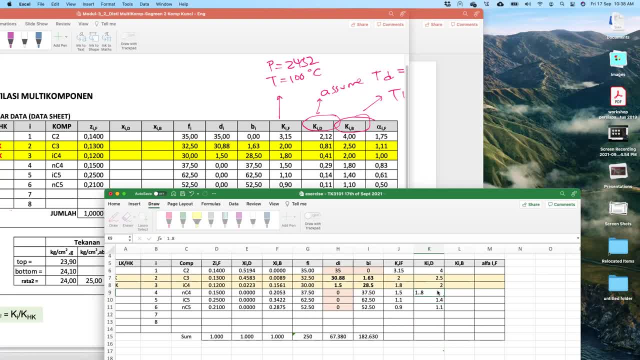 okay, and oh, sorry, this is the distillate. yeah, okay, and this is four point. uh, the distillate is 2.11, 0.81, 0.41, 0.29, 0.41, 0.41, 0.14. 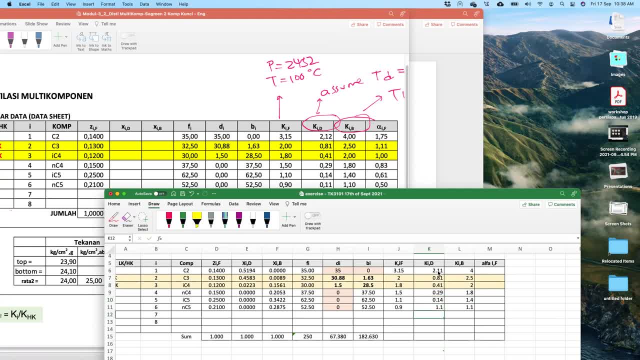 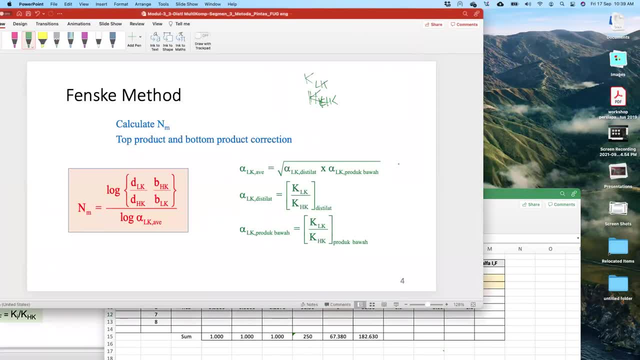 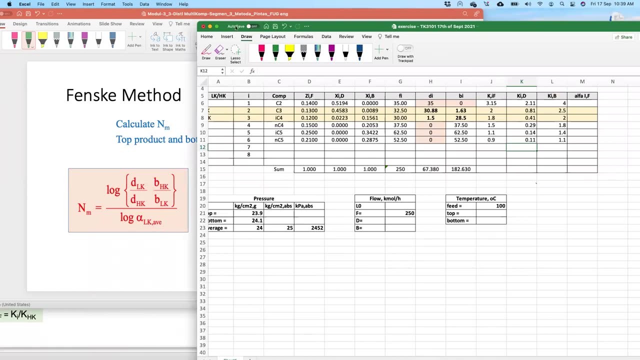 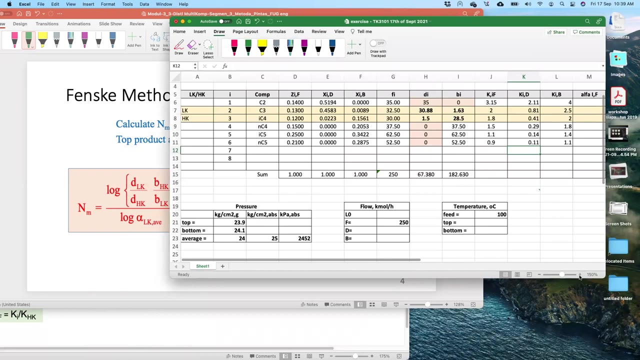 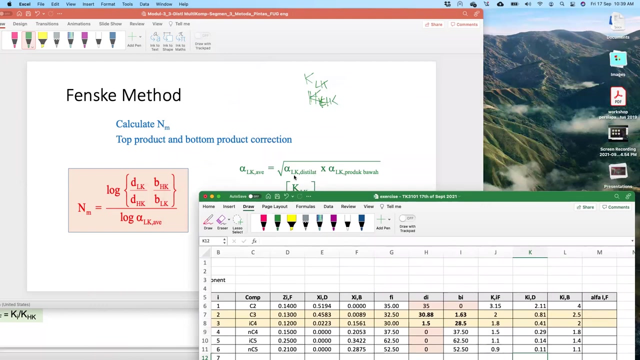 and 0.9, yeah, 0.11, yeah, just let's say, uh okay, let's say i got this one, yeah, this number, okay, maybe we can make it bigger, yeah, okay, okay. so here i have to find the lk average. yeah, i have to find the lk average, which is um lk distillate plus lk of the bottom product. 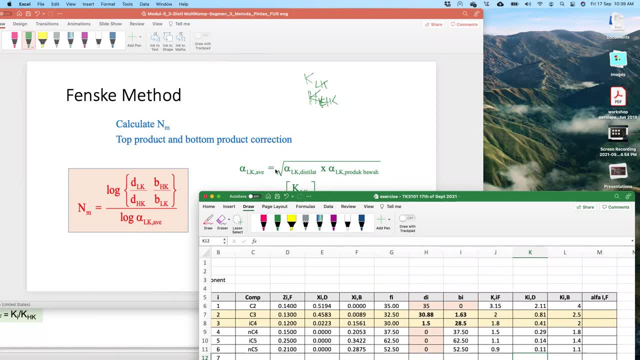 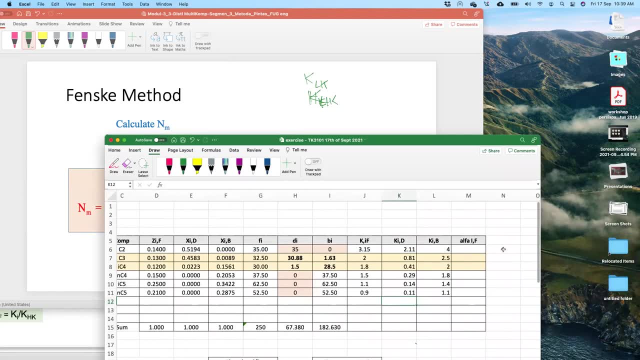 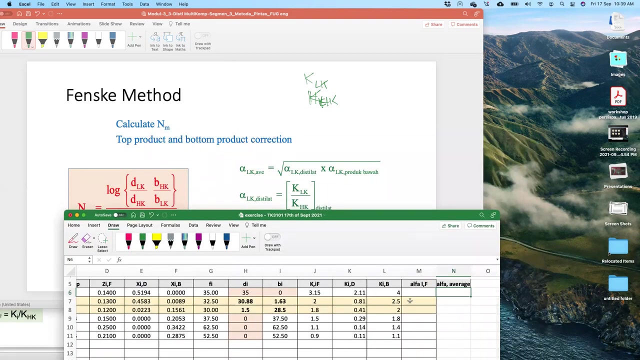 uh, multiply it and then, uh, we have to square root them. okay, so here, uh, i can write: maybe, here, uh, alpha average. so here, uh, i can right. maybe here, uh, alpha average. okay, so here, uh, i can write: maybe, here, uh, alpha average. Okay, alpha alpha. this one is the LK, so alpha, so alpha, so the alpha alpha LK. wait, wait, so this is the alpha, so the alpha. 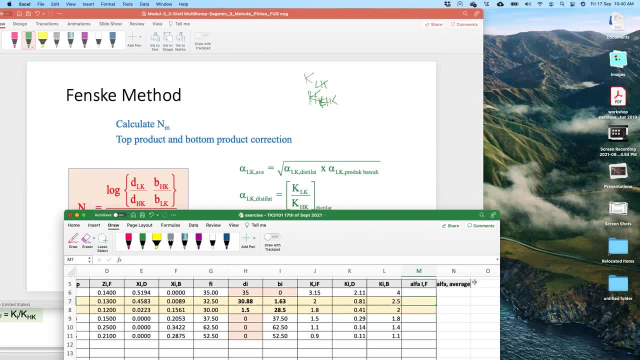 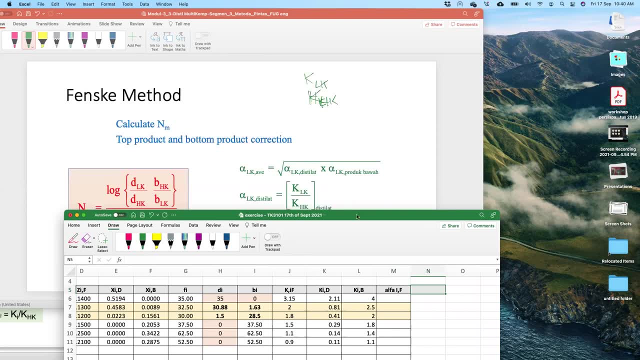 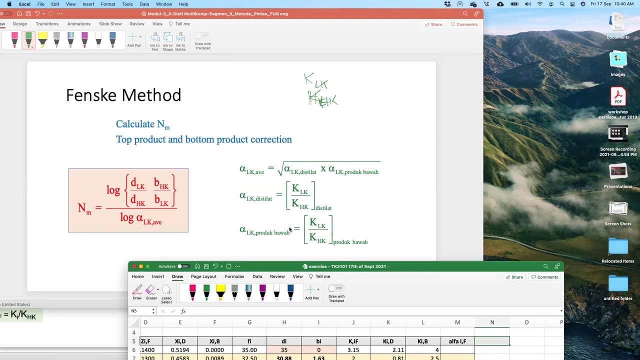 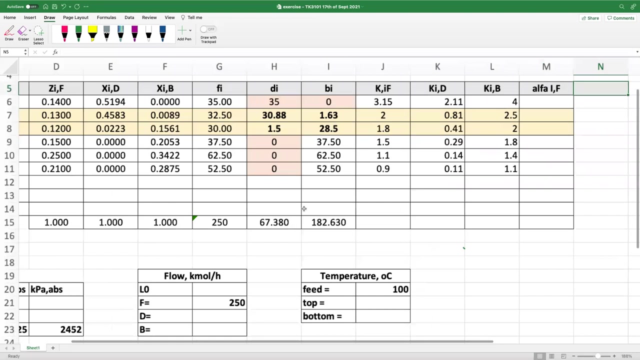 so first- sorry, we have to find first also not the alpha average- first we have to find- wait, we have to find alpha distillate first. yeah, alpha in the distillate and alpha alpha in the H key, the heavy key. okay, make it bigger here. okay, so the 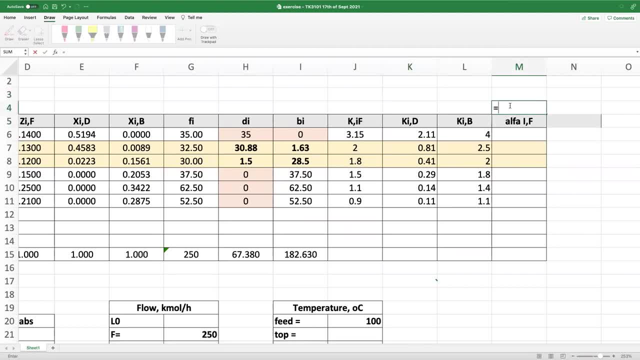 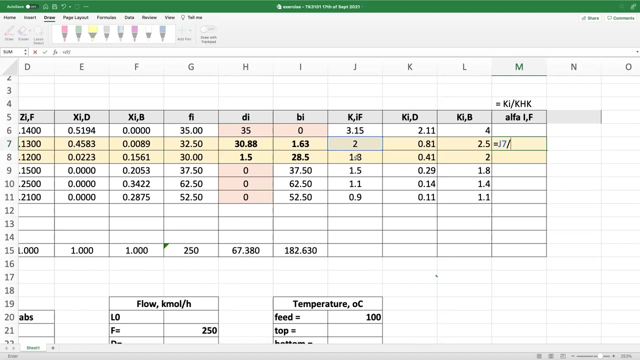 so the alpha is defined as equal to KI divided by KHK. yeah, okay, it's equal to KI divided by. okay, I divide by KHK. so this is the. so the alpha alpha of the feed, for example, here is equal to alpha of the feed divided by the alpha of KHK in the feed, this one. 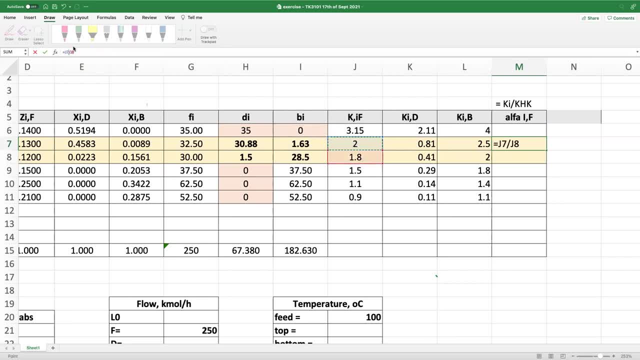 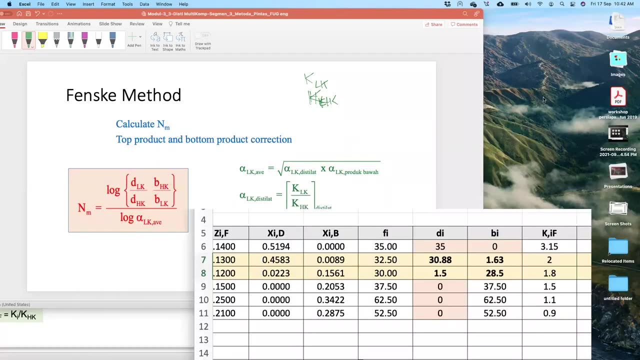 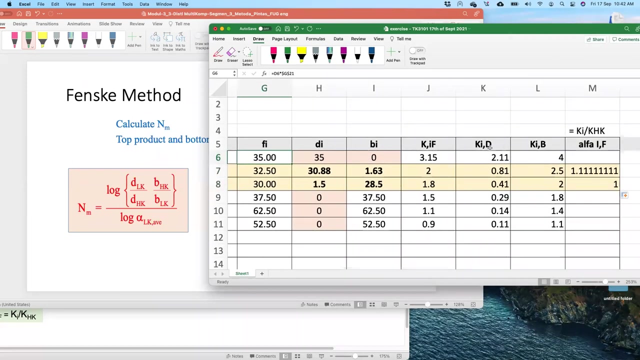 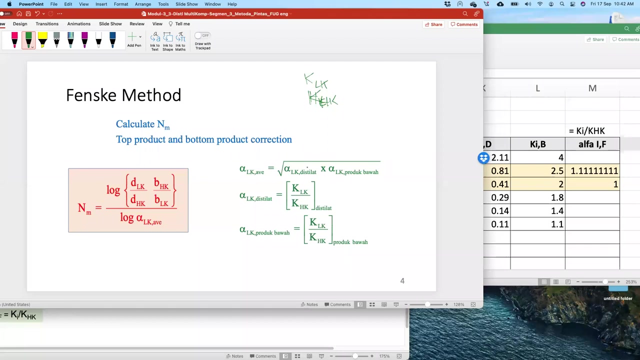 alpha in the feed divided by alpha HK. HK in the feed, I'm gonna put it dollar there. so this is the alpha and this one over there, alpha like that, okay, and then we do it like that so to get those. so once we know the KIF, KID and KIB, we find also the alpha. and also once we find the alpha there and then find the distillate, 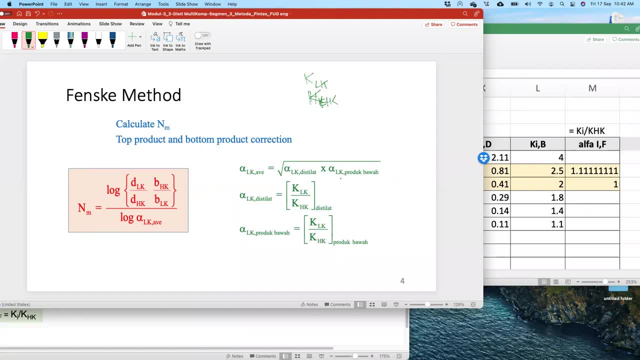 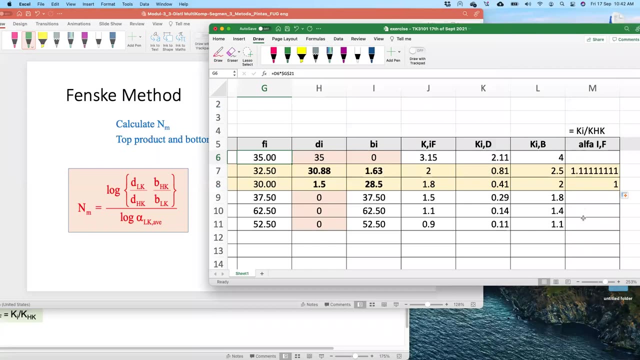 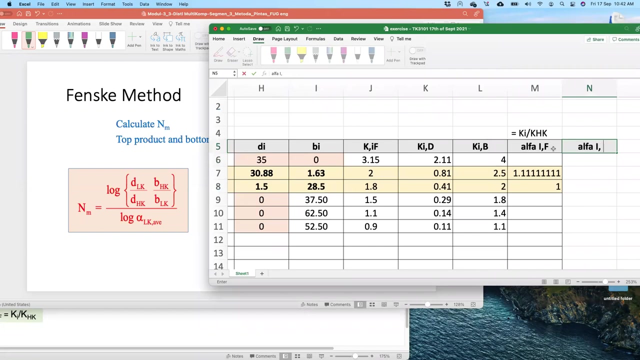 in the distillate and alpha in the bottom product, and then we square root it and we get the alpha average, okay, and then with that then we can calculate the NM. okay, so then this is pretty straightforward. but you have to know all of the this one. so you have the alpha E in the feed. you have to find alpha E in the distillate. you also have to find alpha E in the bottom. 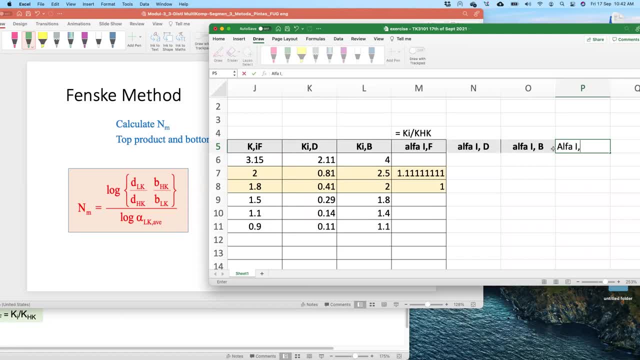 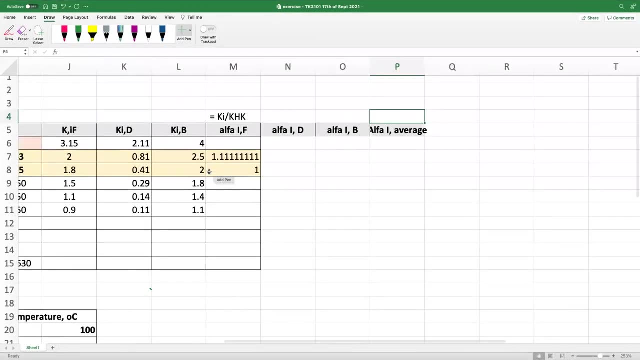 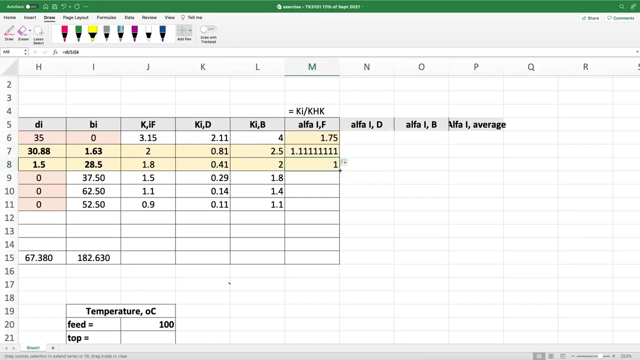 and then you want to find the alpha E in the separate K, so you have to do the co. those too, образом. Okay. so let's do that quickly. This is the alpha in the feed. there In a hurry. 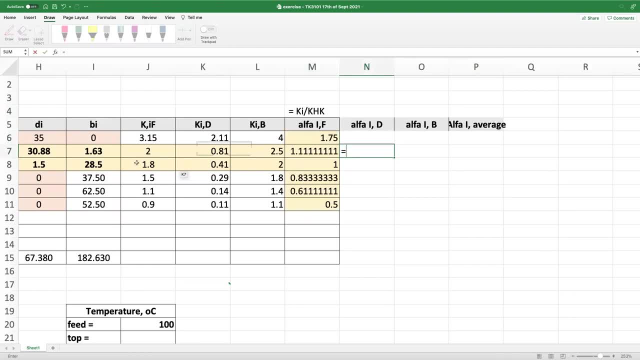 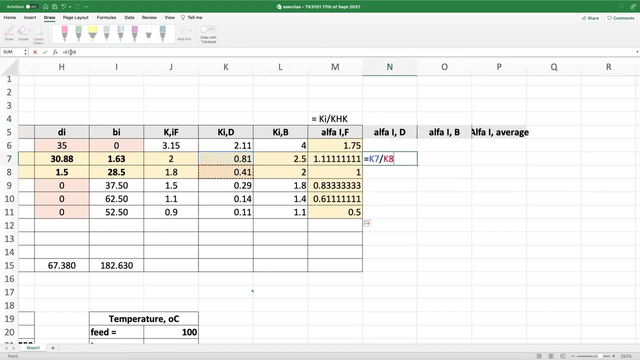 Okay, And then this one is: I want to find all four Aquí: the distillate, which is the K in the distillate, divide by the heavy key. yeah, you also want to find the heavy key there and put it there. and also alpha in the bottom. make it easier, okay, and also alpha in the bottom. 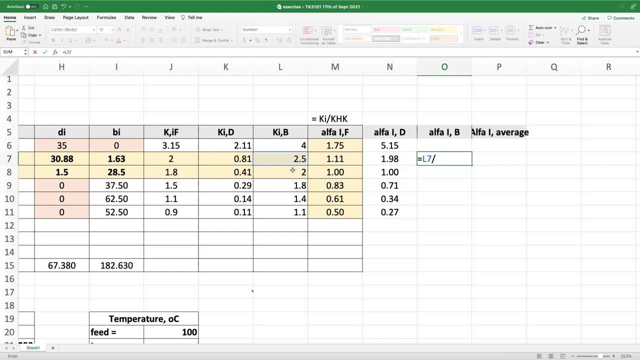 K in the bottom. divide by the K, H key, yeah, H? K in the bottom. put the dollar in, so divided all of them and alpha average- alpha average is actually alpha in the distillate- multiply with alpha in the bottom and then you square root, yeah. 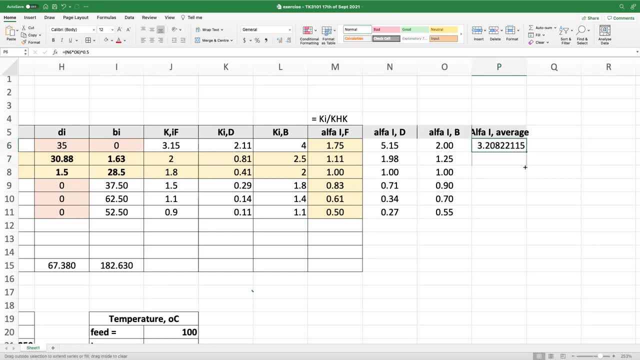 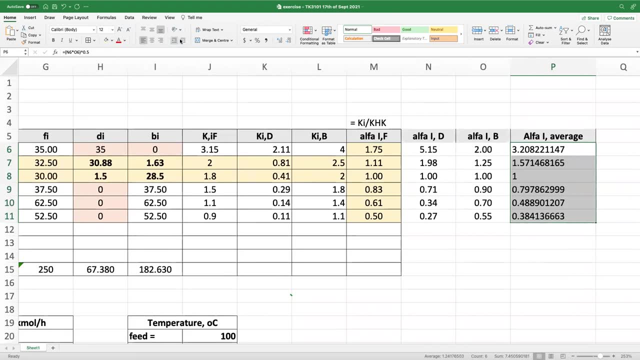 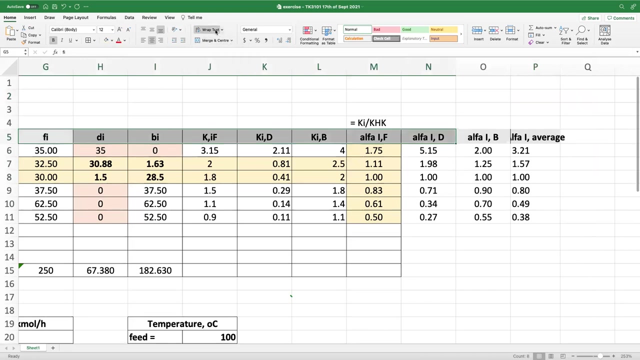 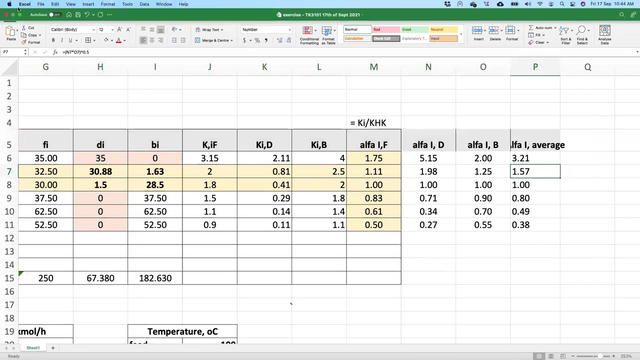 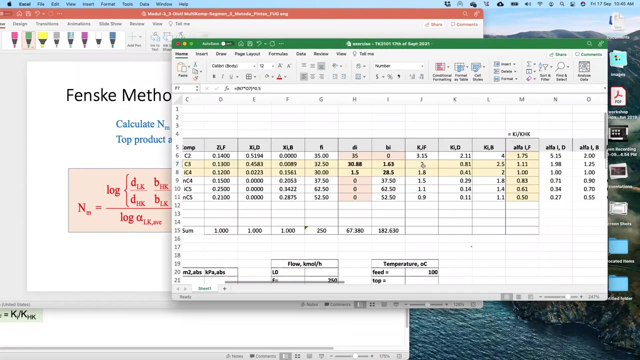 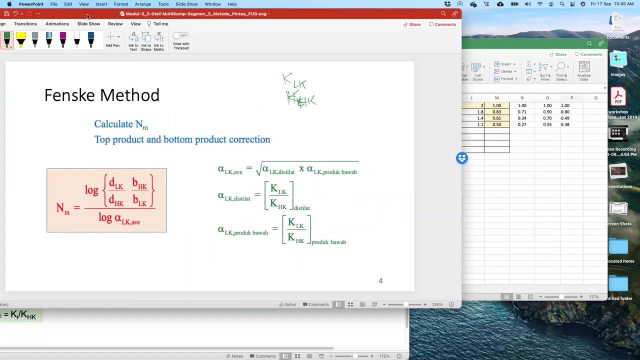 multiply with 0.9, that is your alpha average. okay, so you know the alpha average. now put it there. put it there and then stop text here. okay, so once you know the alpha average, then you can calculate this one. so NM: yeah, I'm gonna copy this one here, just to make it easier. 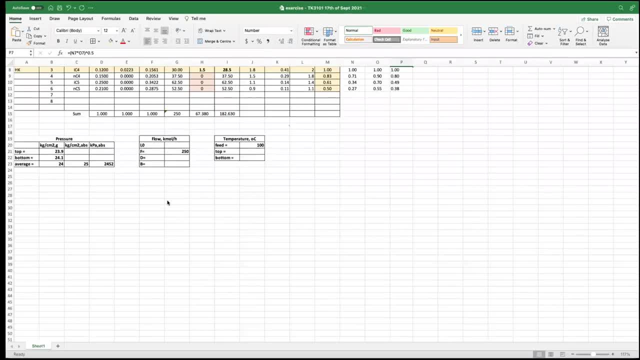 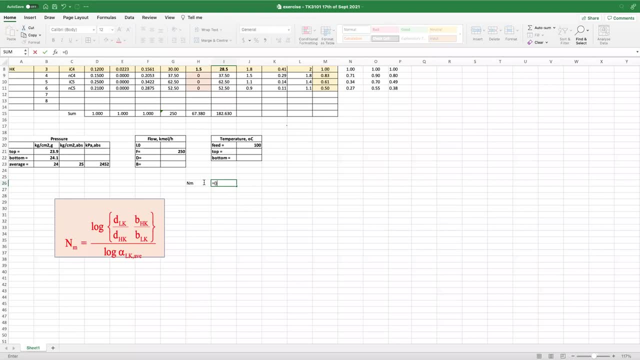 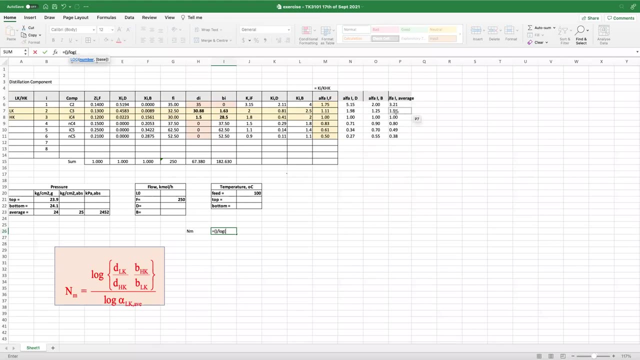 to the spreadsheet. we have to go back to the spreadsheet. so, NM, if the divide by log of the alpha average, alpha, the light key average, which is this one alpha light key average, and spot the value of alpha camera andowing value of alpha lens to the predetermined value of alpha hair. so this is 1.. pictures, forehead viplay: zoomаки effort円 a cat. 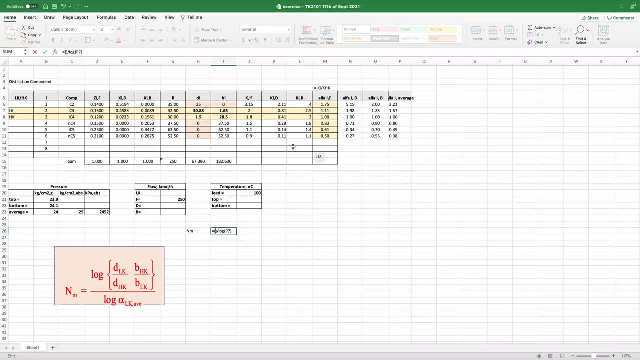 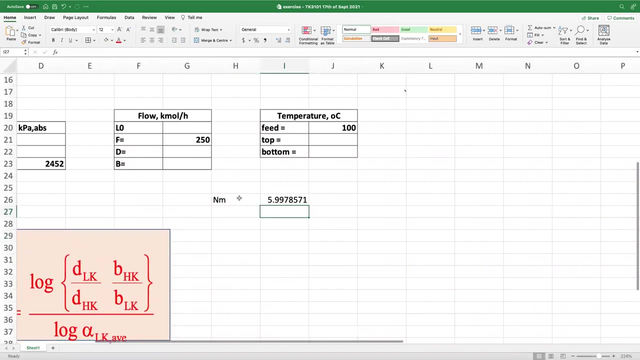 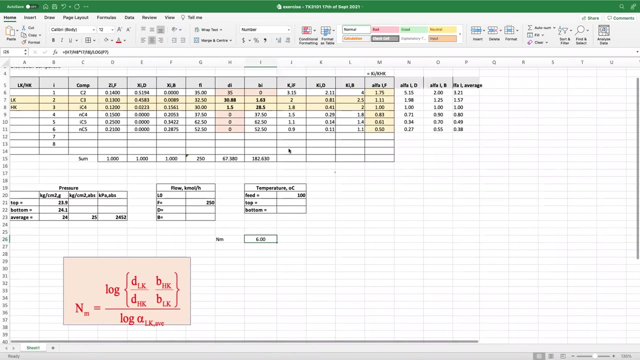 And then if you look at here the NM, it should be DLK. so this is DLK: DLK divide by DHK. multiply with BHK divide by DLK: See. So my calculation says that the minimum is about 6,. yeah, So NM is my minimum value, okay. 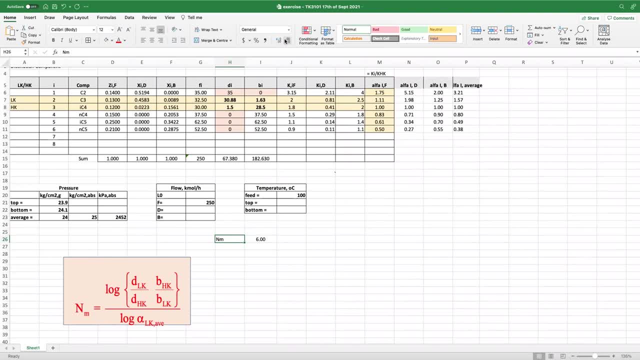 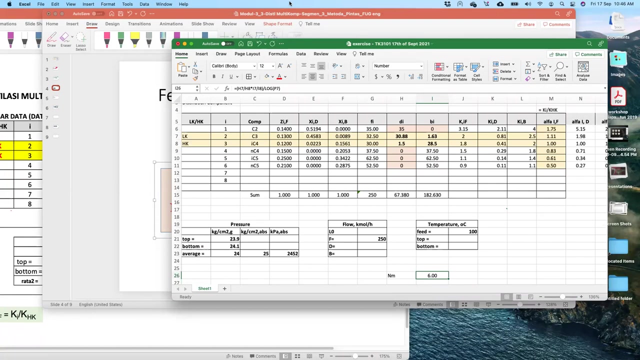 So this is my NM, or maybe, yeah, 2, is fine, yeah, There, okay. or just 2, okay, So this one. So my NM is 6.. Now the question is so based on this one. of course it's gonna be recorded. so after this, maybe on Friday night, I'm gonna start uploading to YouTube and then put it into EduNext. yeah, 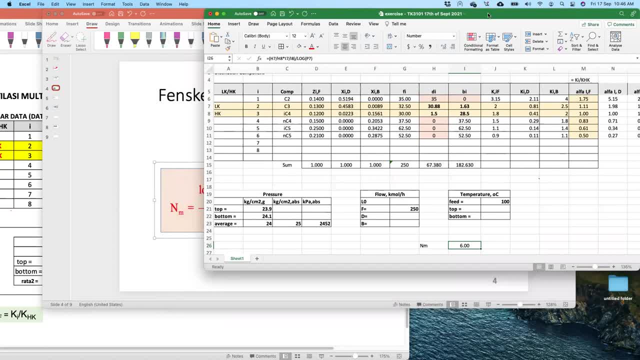 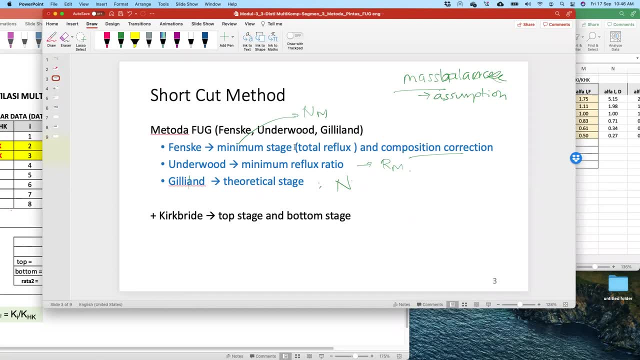 So you can have a look. The next step is to. I promise here that Fensker is to find the minimum stage, NM, the total reflux, which is I got it. The second one is the composition correction. ah, how to get that, yeah? 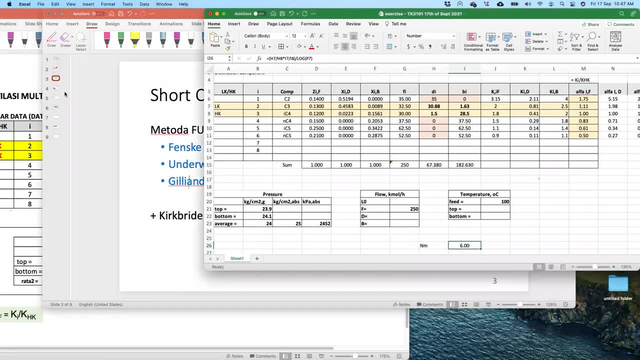 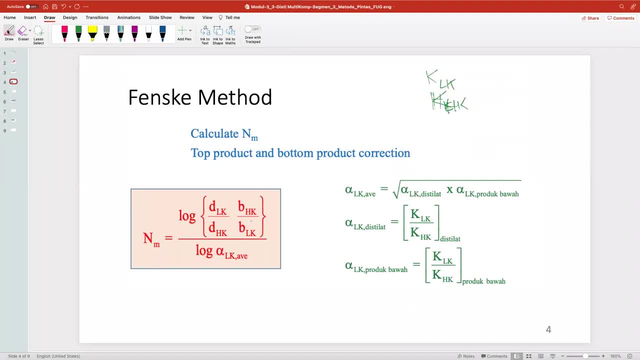 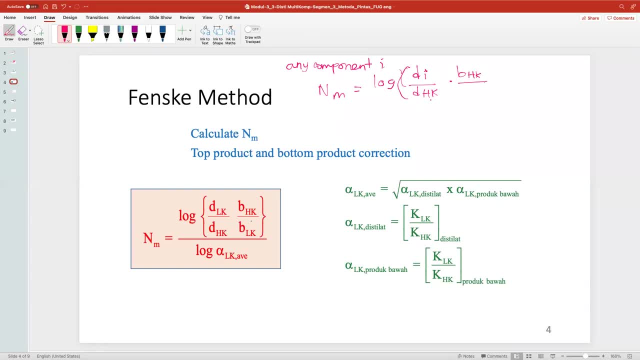 Divided by BHK, for ah B DI, yeah, divided by log alpha I average: yeah, So, ah, because we know NM, yeah, we know NM. ah, we know BHK. divided by DHK, we also know the EI average. then we can find the ah DI over BHK. 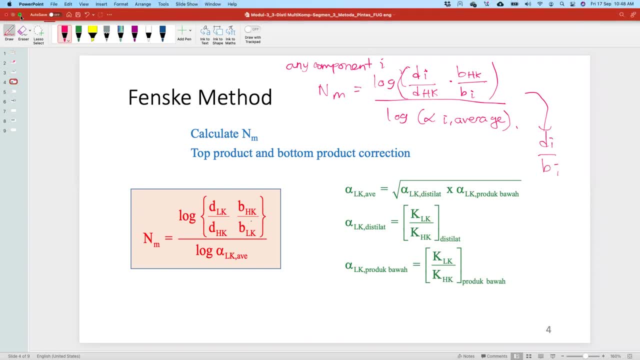 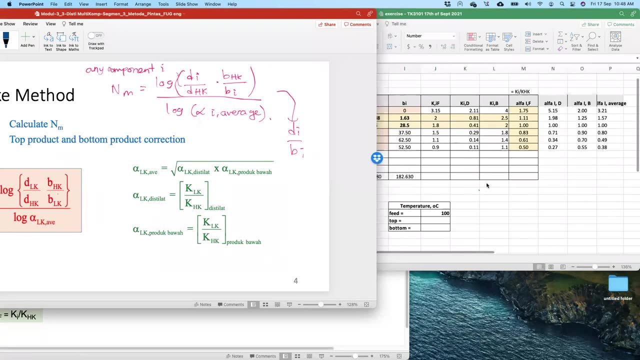 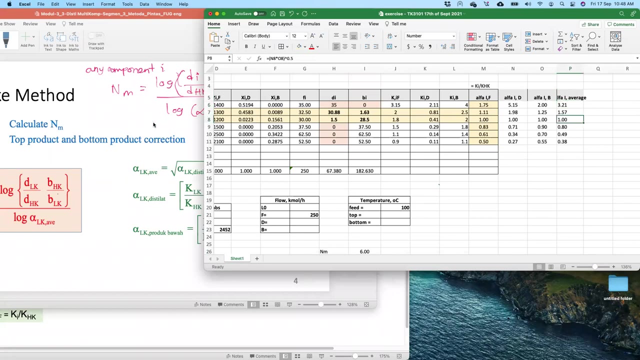 So from here we can find ah DI over DI there. yeah, Ah, the alpha average. we know that for for each ah component, I, ah, we know the NM. now NM is 6.. 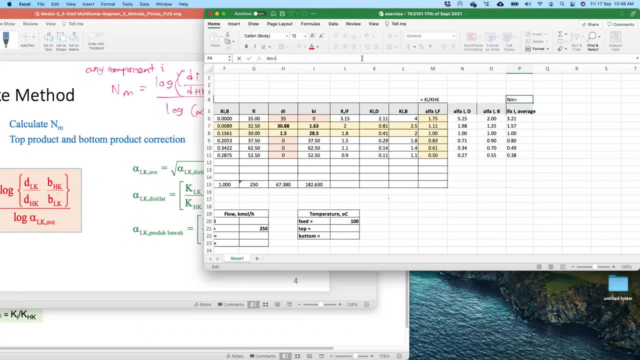 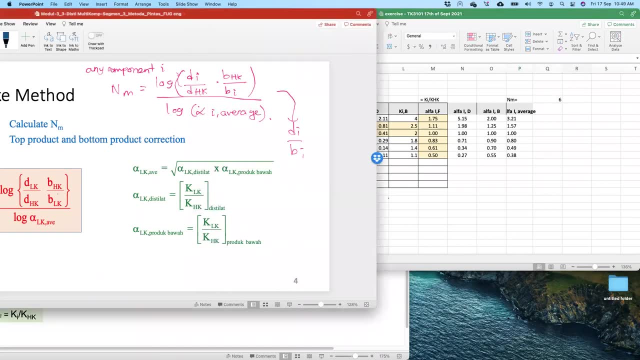 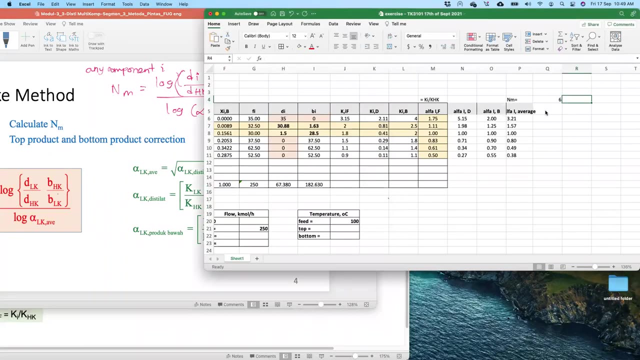 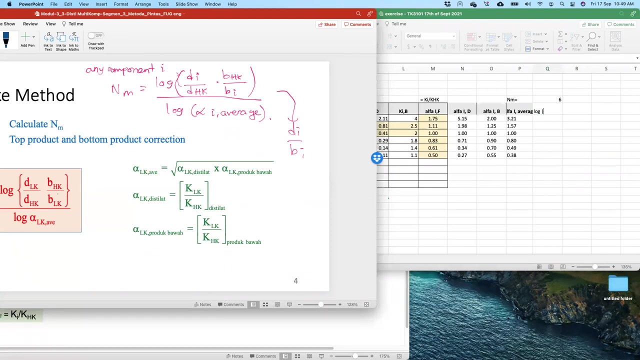 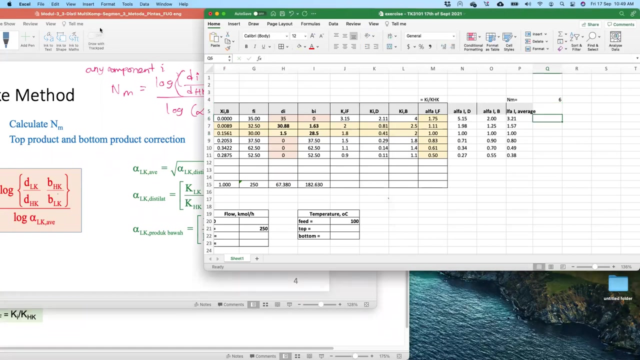 Okay, Okay, Um, we also know the ah. so then we can find: here is the log, ah, that one there, yeah, The log, oh yeah, so anyway, it's going to be too long, but anyway, later on you can, you can find it. ah, back to here. um, yeah, 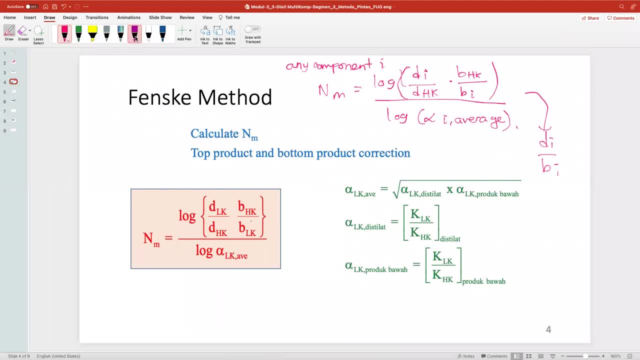 It's going to be too long, but anyway. Okay, you should find the NM. you got it, for example, 6.. You also can calculate the alpha. I average, yeah, for each component from 1,, 2,, 3,, 4,, 5,, 6.. You know the BHK, the component in the, the amount of the bottom and also the amount of the heavy key and also the distillate of the bottom and the distillate of- sorry, this one is. we want to find this one, yeah. 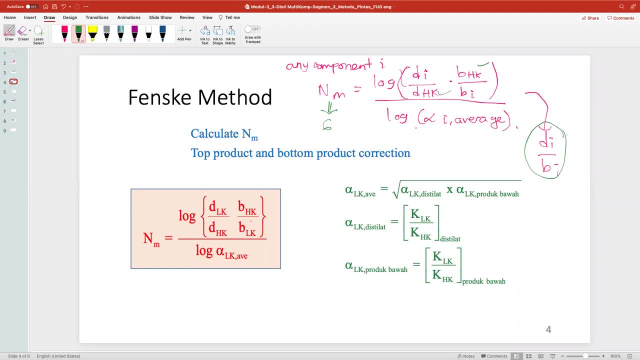 So this one is known, this one is known, this one is known and NM is known. then we can find DI over BI. So this can, and also we know that DI plus BI is actually going to be in the feed. okay. 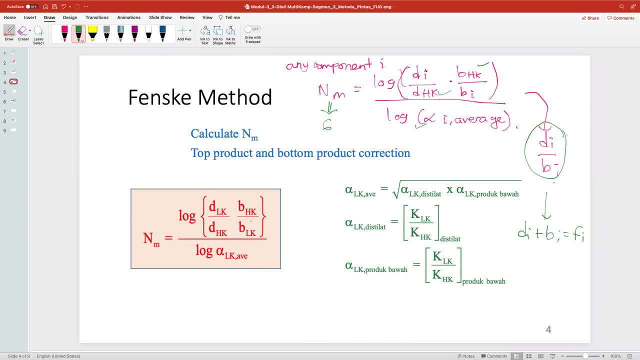 So once we know the ratio between the DI and BI from this equation, then we also know the feed. then we can find the DI over BI. DI and BI corrected: yeah, Sometimes the correction, sometimes, yeah, there should be some correction. 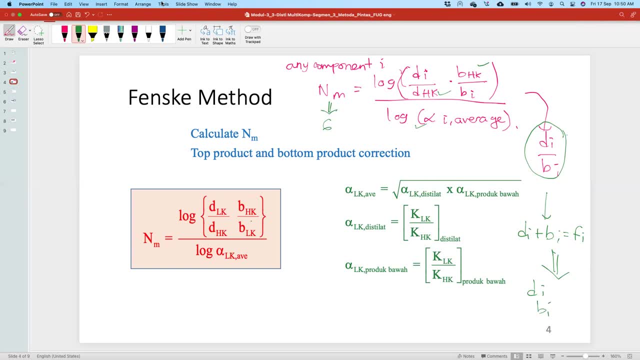 So our assumption sometimes is not correct. For example, there's some tiny bit of component heavier than heavy key in the in the distillate. but again, let's see this correction. All right, you may want to see this video again. 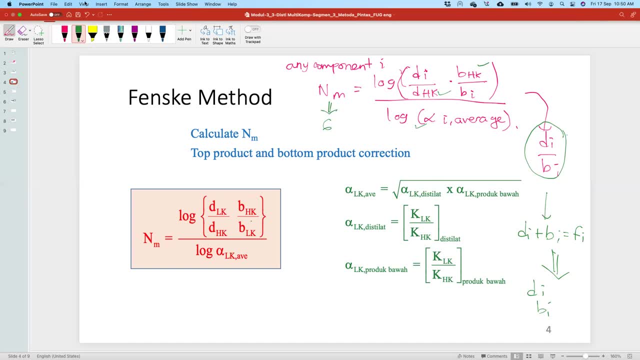 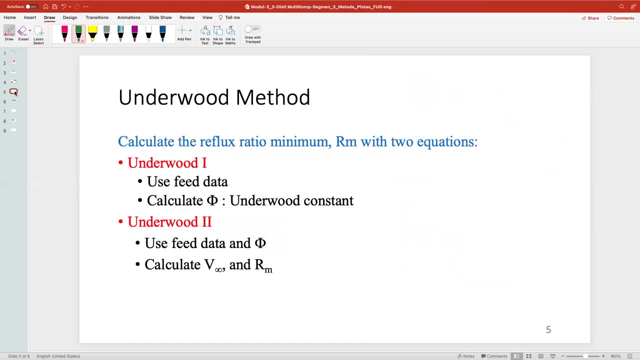 When you do the assignments, maybe the next two weeks, but anyway, just for now, just just leave it like that. yeah, Okay, the next step, the next question, is to, once we know the NM, the next step is to find RM. yeah, with Underwood method. 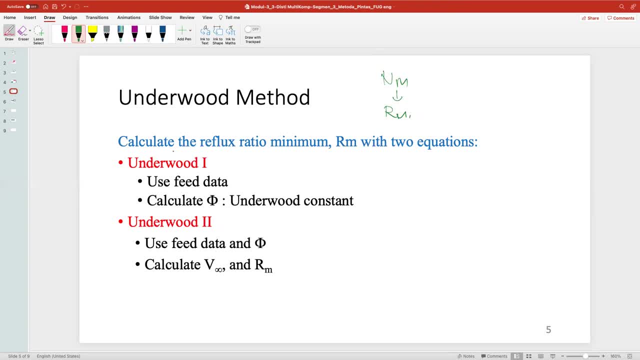 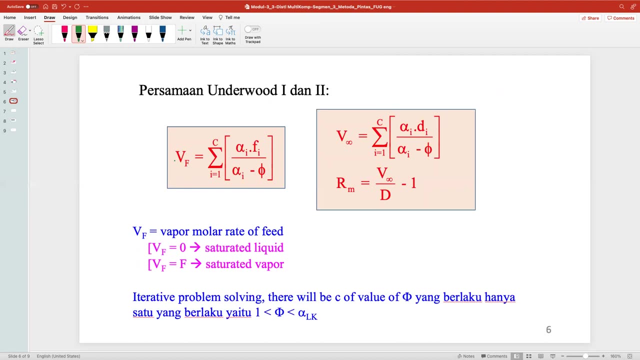 In the Underwood method we calculate reflux minimum RM with the the RM. So what are two equation? the equation First is Underwood 1, and Underwood 2.. Okay, in the Underwood 1 and 2, this is the first equation for the Underwood 1, and this is the Underwood 2,. the equation two: 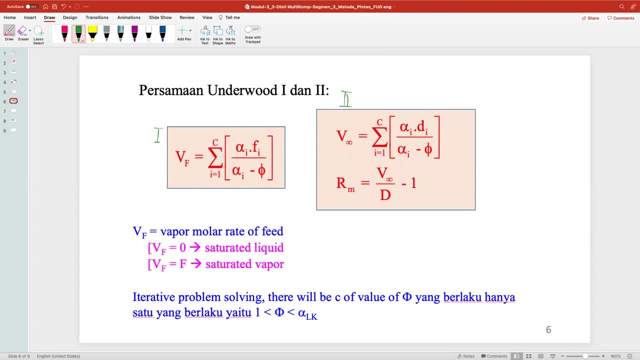 Okay, So we want to find the VF, which is the vapor molar rate of the feed, The molar rate of the feed, vapor feed. we calculate it with a sigma or alpha i divided by fi. yes, so if it is, we have, for example, 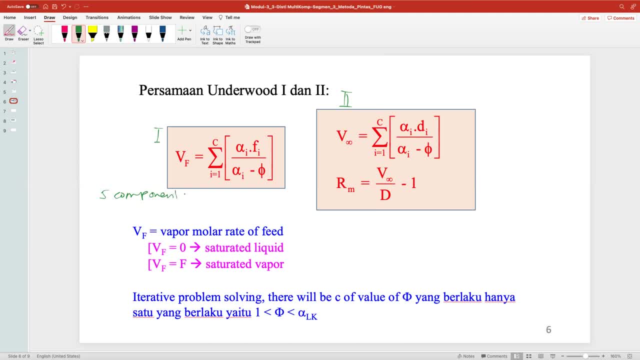 five components. you can imagine it's gonna be a very long equation. so vf would be: alpha i divide by f multiply with f i. alpha i minus c plus alpha two. f two divided by alpha two minus c. this one, yeah, plus alpha three. f three divided by alpha three minus c plus alpha four. f four divided by. 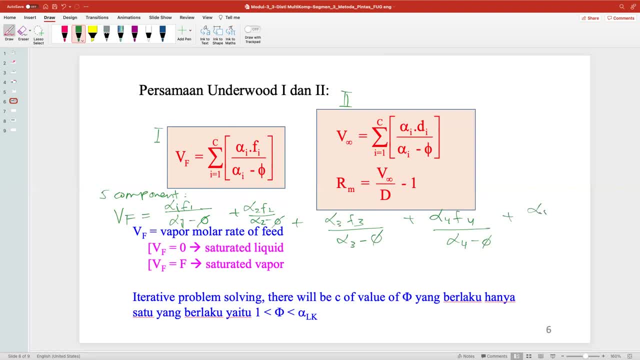 alpha four minus c plus alpha five and five divided by alpha five minus P. so you, you know, the molar fraction of the feet in it should be in the in the in the problem. yeah, it is saturated vapor, or is it so on then, then, what you want to find. you want to find. 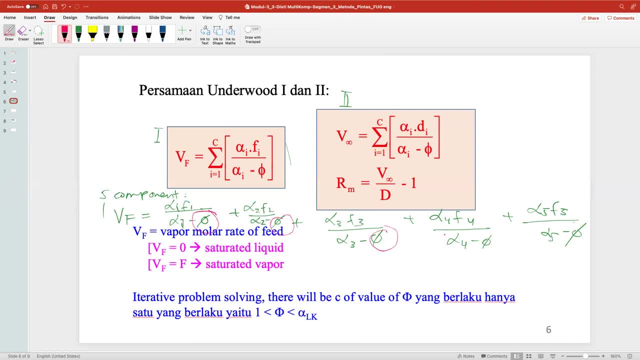 this C, okay, so in in Excel you can't do that because it's not really linear. yeah, it's not in your equation. so we're gonna use a solver. so you solve for in your Excel, you single thick yeah and then use again. use the button yeah at our. 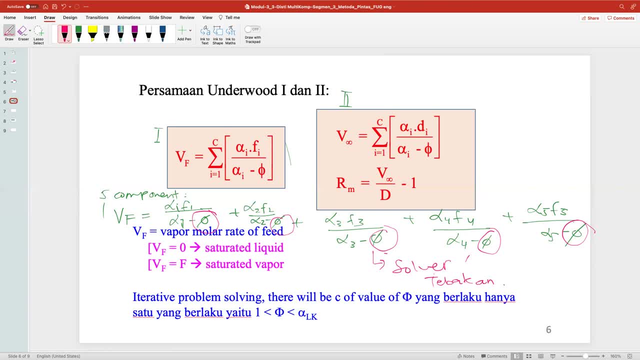 assumption. so it is going to be iterative problem solving. so there would be C values, you of C, and then the one that is applied is only when the P C between 1 minus 1 to alpha. now I keep: yeah, so that. so of course, if you remember about, about, 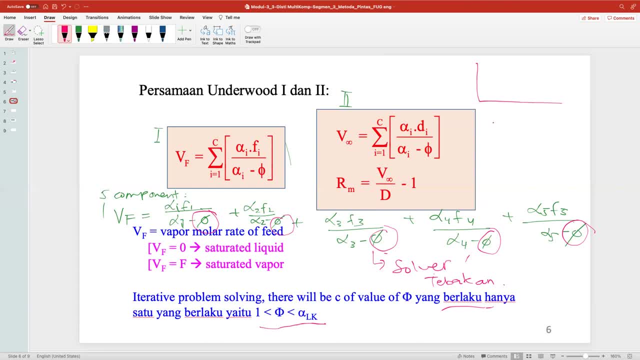 Newton, Raphson and so on. yeah, if, if this is an example, for the body is an equation- are one, two, three, four, five? maybe there is a one, two, three, four, five num uh value that uh can go to here? yeah, but then you want to only uh, so find the assumption tebakan uh that close to uh. yeah. 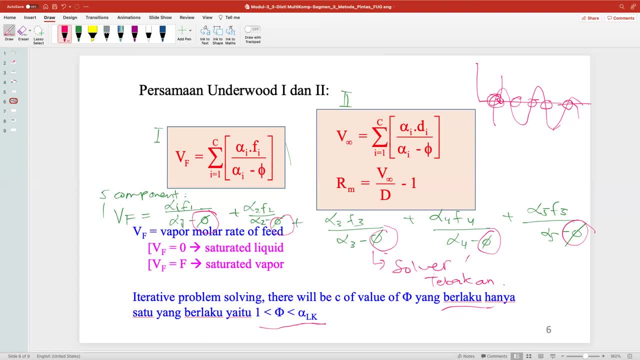 your, your tebakan or your iterative assumption should be stuck between zero and one, two, uh, like key. okay. so once you find the c, the next step is to go to the v, infinity, uh. and then here you can just calculate: uh, the alpha i multiply with d, i divide by alpha, i minus the c that you get. 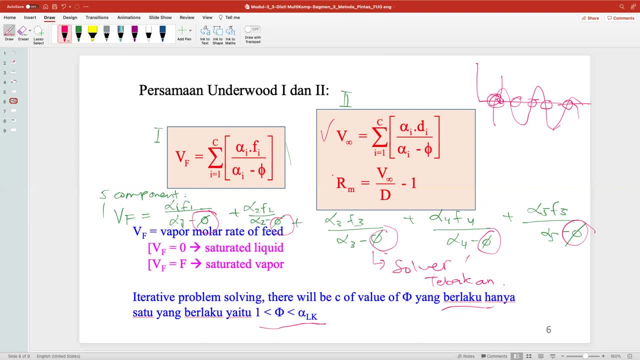 and then, once you got the v infinity there, you can find the rm, uh, by v infinity divided by d minus one. okay, so this is the underwood correlation. okay, so now, uh, once. so it is gonna be quite long as well, uh, to find the rm, to find the c first, and then to find the v infinity, and then to find the rm. 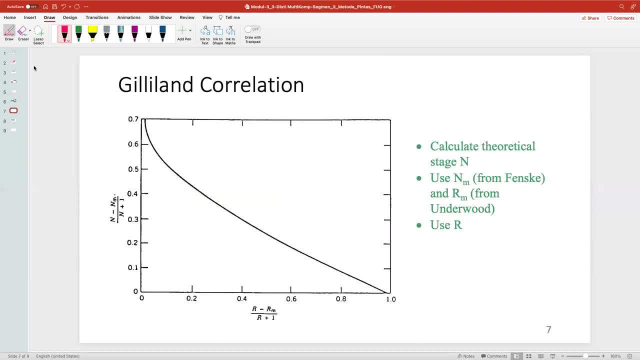 then the next step after that is: we want to find the gililand correlation. yeah, in gililand correlation it is just using a graphical correlation. so they have a graphical correlation between uh n minus nm divided by n plus one. uh with r minus rm divided. 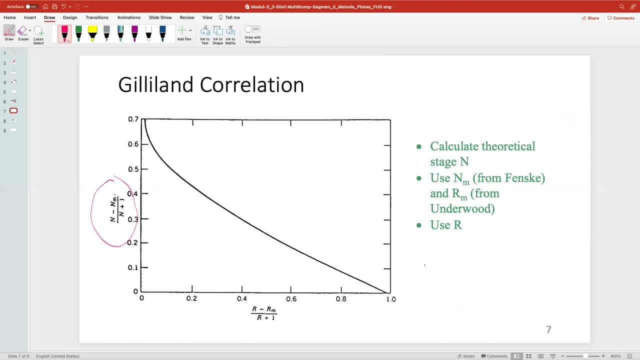 by r plus one. okay, so, uh, you know the rm, and then maybe you can find the r bay. i don't know, uh, based on the problem, maybe 1.15 or maybe just uh, maybe the d minus d minus d nm divided by 2. okay, and then um, um, that's what we're going to do for now, okay, so, um, so, let's go ahead and we'll go ahead and check the problem. okay, so, let's just go ahead and see if we can solve this. um, let's see what happens here. okay, uh, so. 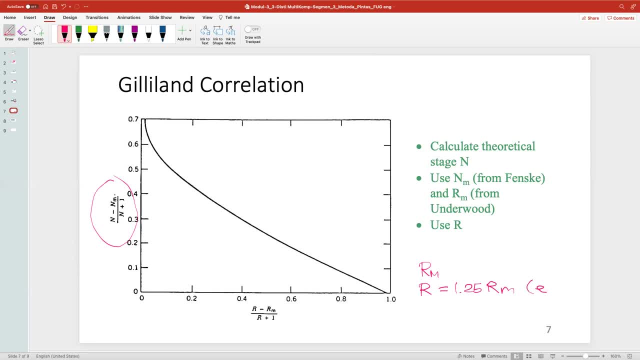 125 RM, for example. yeah so, and then you calculate this one here and then, for example, you can get the that one there to the graph and after that you follow the graph goes to see the vertical axis and then you find your N minus NM divided by N plus 1. okay, you know the NM, it's known from the Fensker correlation. 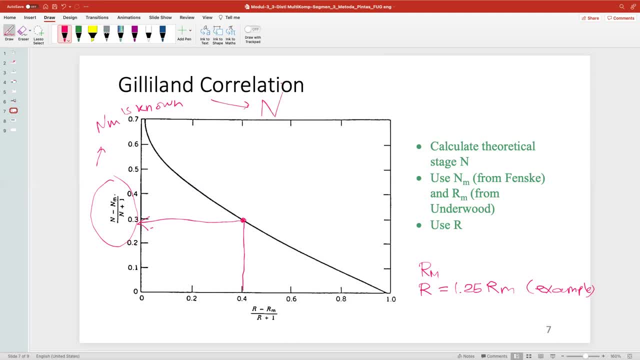 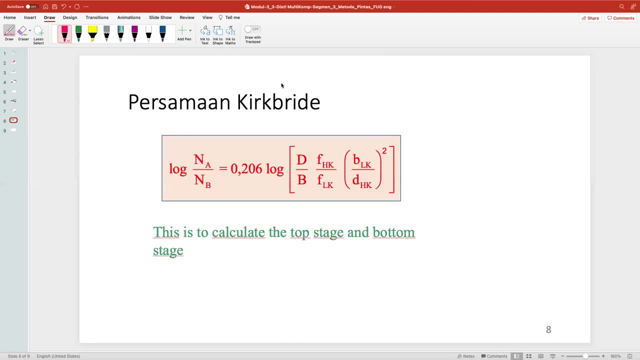 and then you can get N, okay. so that is to get the N okay. and the next one is the Kirk bright to calculus, top, top stage and the bottom stage using log. yeah, so it's the top and the bottom stage. So we know the D, the composition of D, composition of B, we know the feed, also light key and heavy key, B, L key and heavy key, and then put into this correlation then we can get the NA divided by NB. 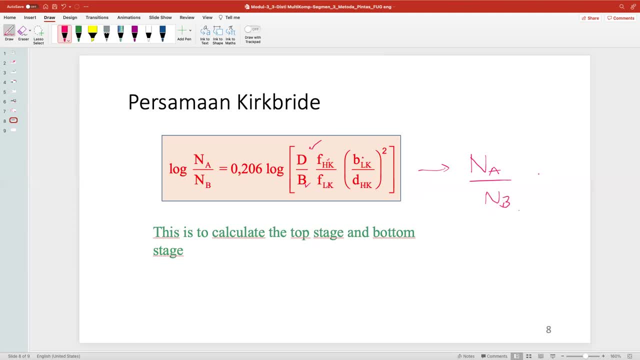 Okay, and then we also. this is equation number one, for example, blah, blah blah. and the equation number two is where the NA equal to N plus NB equal to N. Yeah, we also got it from the previous one. yeah, the Underwood, the Gilliland method. 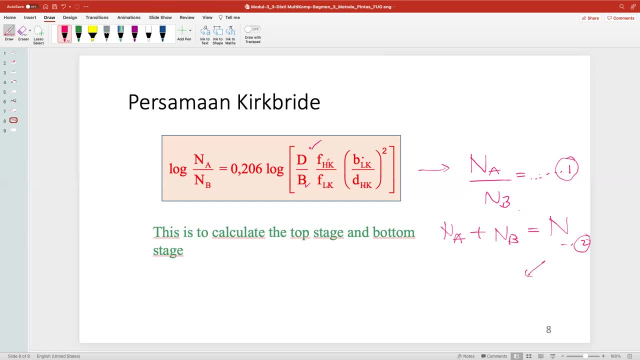 So once we know the N, then we know the NA, N and B. Okay, so so then. So that's, that's the shortcut method to find the number of theoretical stages in the multi-component system. It's still a good assumption, even in the high-speed. we have to do shortcut distillation first to get the idea how many stages that we will have, and after that we will go to the. we will discuss the rigorous method or the egregious method. 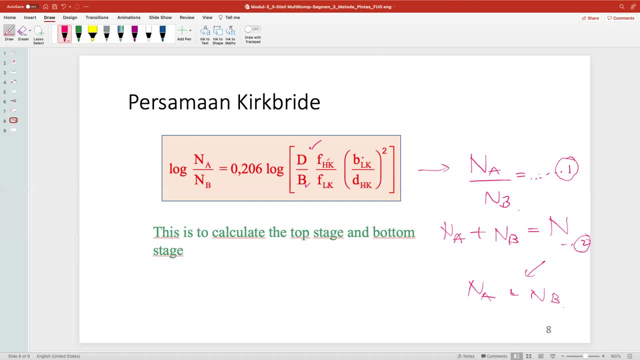 Where we're gonna do the iteration in each stage to find the the, the correct temperature, the correct pressure and also the composition in each stage. All right, okay, that's quite heavy for you, Anyway. do you want to have a comment or questions? 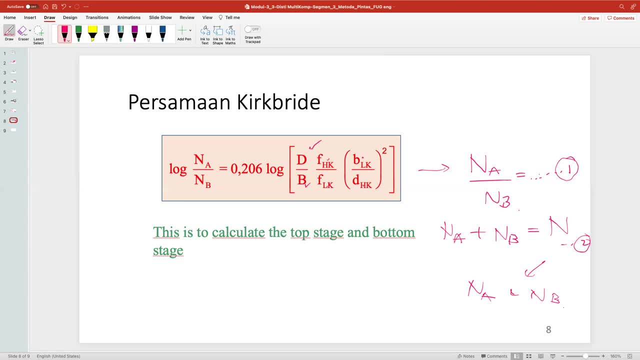 Questions: Ibu, Yeah, Nadifa. Ibu, Yeah, Nadifa. Ibu, Ibu, Ibu, Ibu, Ibu, Ibu. I asked about yesterday's exercise. Yes, yes, you can. I'm still quite confused with the energy balance. 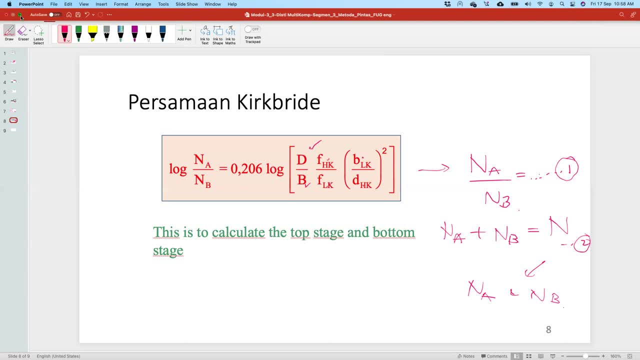 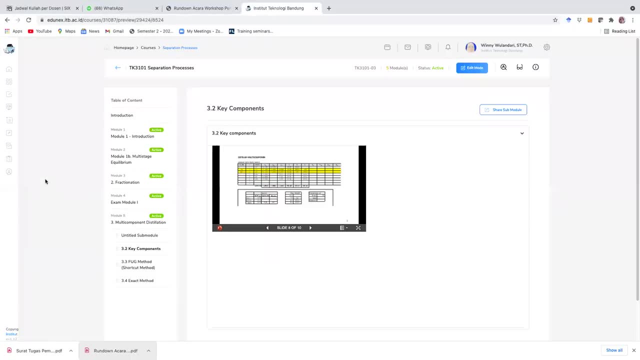 Right, good For that one. I have put the answer in the edu next, So you may want to have a look, but please again do it by yourself. You can go back to the exam module, the practice and this one. 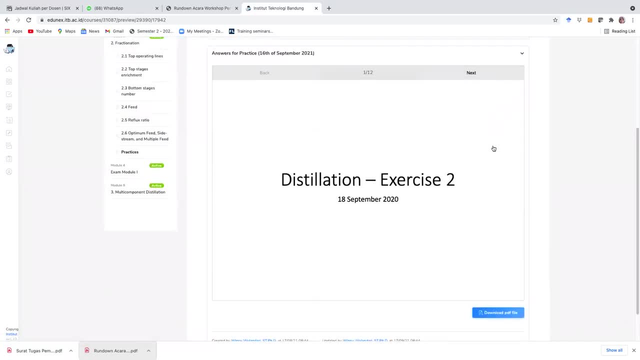 So Ibu Grace has prepared the This one there. So this is 17 September 2021, so exactly almost one year ago. yeah, So here Ibu Grace has explained to you about the condenser duty. yeah, 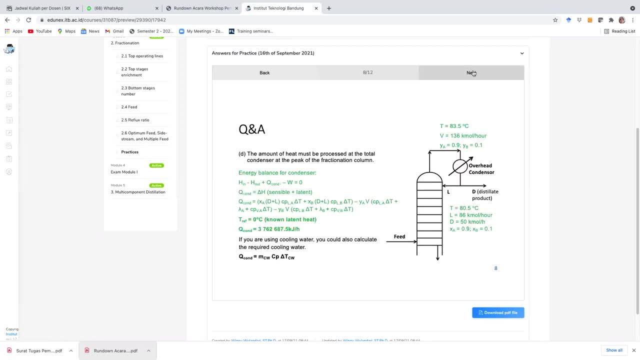 So, Nadifa, have a look, and all of you have a look. You can feel free to rewrite, but when you do, when you rewrite them, think about yourself and then do it by yourself. yeah, So, so, so well, so it can. apa nempel di kepala ya. and anyway, back from here. the, actually the. 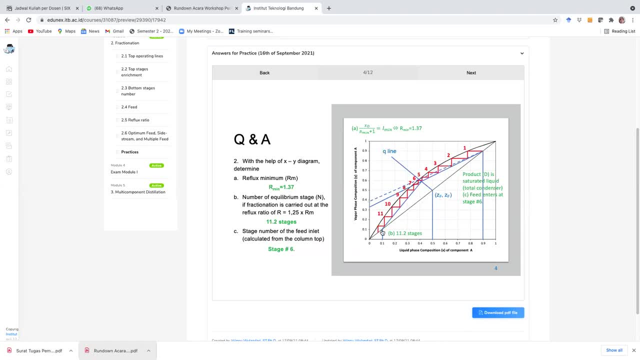 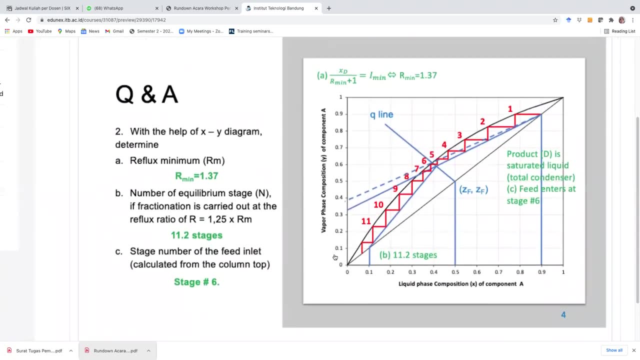 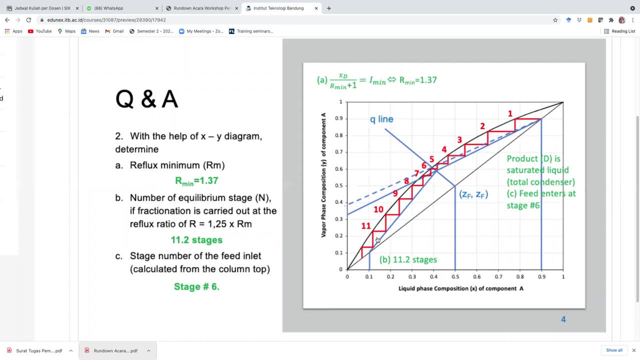 the stages is 11, 11, more than 11.. yeah, here there are two type of uh comments. yeah, first one here. uh bugrae said that is it 11.2? but uh, i say, if i round it up to 12.. okay, which one is correct? uh, it depends on uh how you see it. yeah, uh, if, if i'm checking your uh. 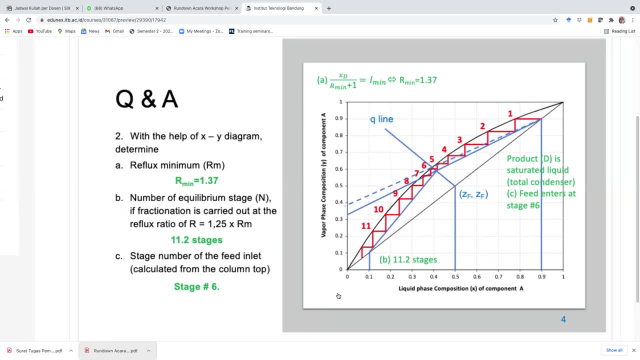 answer: 12 is right. so i'm going to say 12 is correct. so i'm going to say 12 is correct if the equipment is 12.. because in the equilibrium stage we can't have 0.2 stage, right? if you look at the the equipment later, we can't have two stages. so, uh, here i'm gonna round. 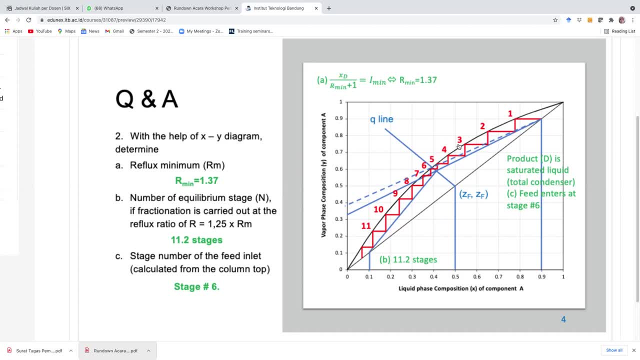 it up if, if it looks like this: one, two, three, four, five, six, seven, uh, eight, nine, ten, eleven, i'm gonna run it out to 12 stages. but if, for example, 10 point something, i'm gonna run it out to 11 stages. if it is nine something, i'm gonna run it up to 11.. i'm going to round up the equipment. 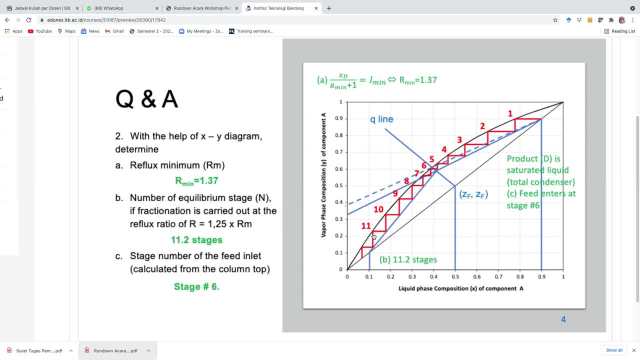 right, because in the equilibrium stage we can't have 0.2 stage, right? if you look at the the equipment, up to uh 12 states, ever up to 10 stages. okay, get it. so, um, of course, i'm gonna explain this to the team teaching as well. so because in the uh in the equilibrium, uh in the tray, yeah, in the equipment, 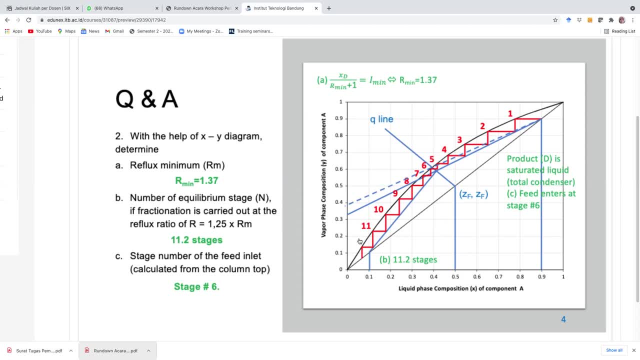 we can't have 1.2 stages, we can't have that one, we have to have full stages. okay, but if you want to write like this: uh, that's fine as well. okay, usually the stages. later on it can be used for the packing column. in the packing column: uh, there is no tray, gada, there's no tray, it's only. 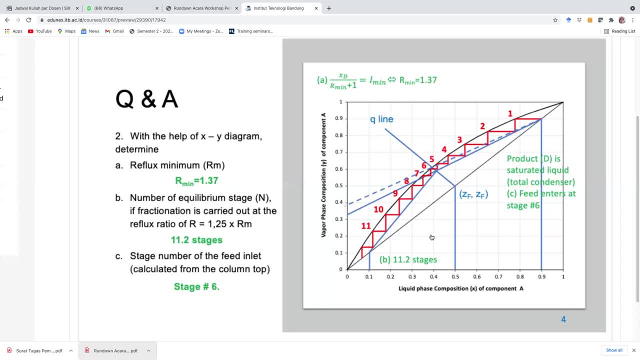 a full of tower, uh. and then you put it: um, yeah, it's just like, uh, like like a tower, uh, like a tower. and then, uh, you, we can uh, for example, specify the length, yeah, and there's nothing inside, just put all of the packing, uh, it may happen in the packing. 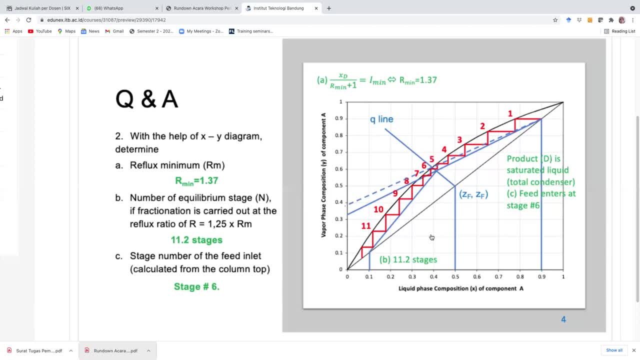 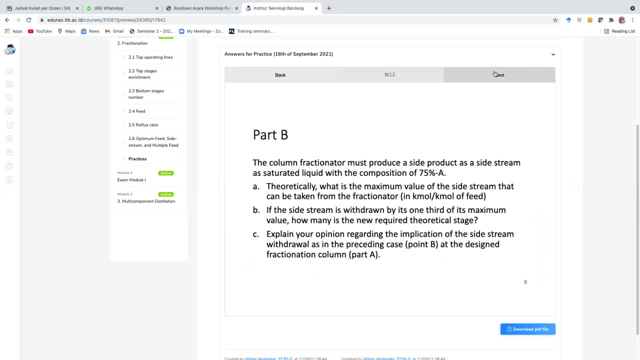 tower, but for equilibrium stages in the tray column. uh rupa bakibaki tray. it is looks like in stages. okay, everyone have a look. so i have. uh, i've given the clue for the answer: practice, so you want to check. and uh, if, and if you look at here, there is also part b in the exam, so this is a tip. 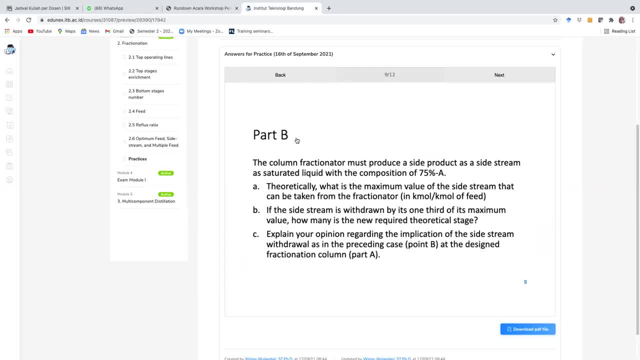 typical. an example of part b: yeah, uh, which is, uh think, uh, let you know about the problem solving. yeah, for example here, uh, for example, if the fractionation must produce a side product as a side stream, at the composition of 75 percent a, for example, as a saturated liquid, what is the maximum? 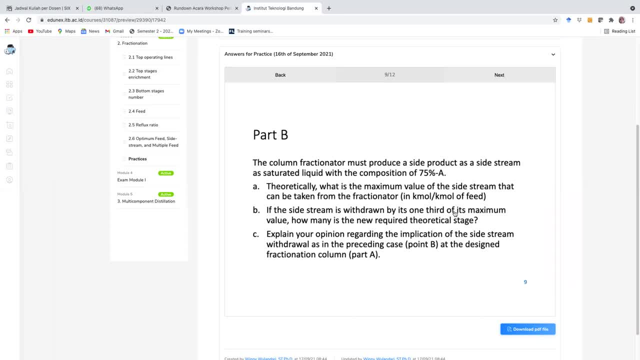 value in the size stream and if the size stream is withdrawn by one third of its maximum, and how many is the new particle stages needed, and then explain your opinion regarding the implication of the size stream withdrawal at this. the design fractionation column: yeah, uh, have a look how to get.